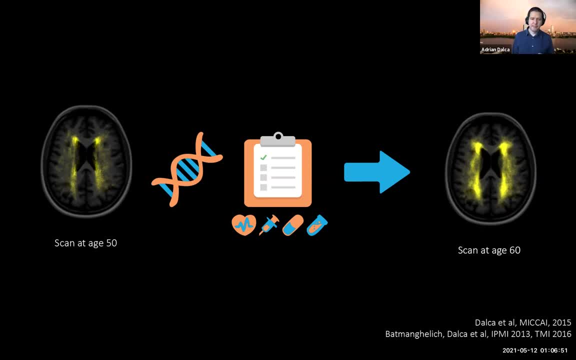 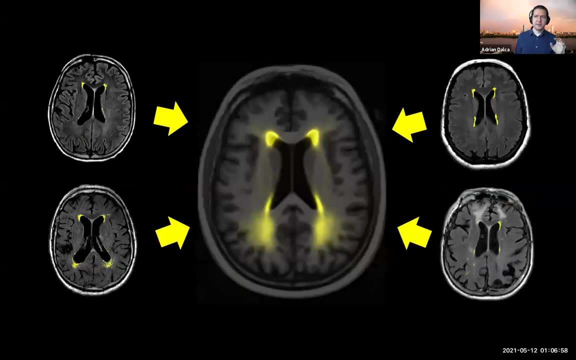 us all kinds of information we want for treatment and so on. But at the core of basically everything I did in my PhD, there was this one operation that was central to everything, which was aligning images to a common reference frame, And it's so central that it's been developed over many. 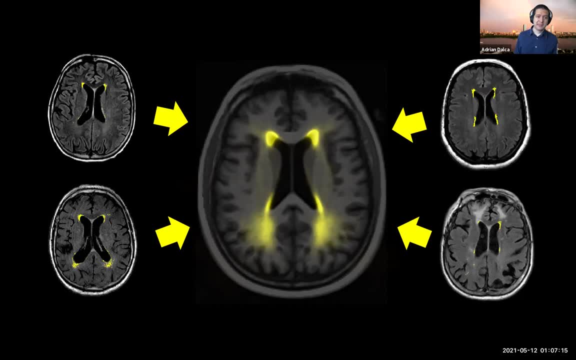 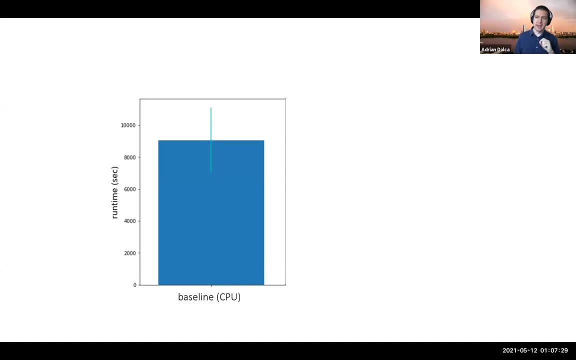 many years, but we had one big problem at the time. We were really really like young students. we really wanted to come up with really fancy models for our data, But just this registration or alignment step took two hours for every brain And that was a problem, because every time we 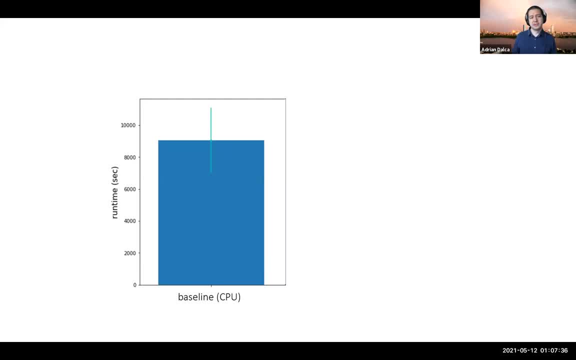 wanted to align something. it would take forever because we had thousands of brains to analyze. But not only was it a problem that we had to one-time align these brains, but it was a problem in that we couldn't develop sophisticated models, because these models 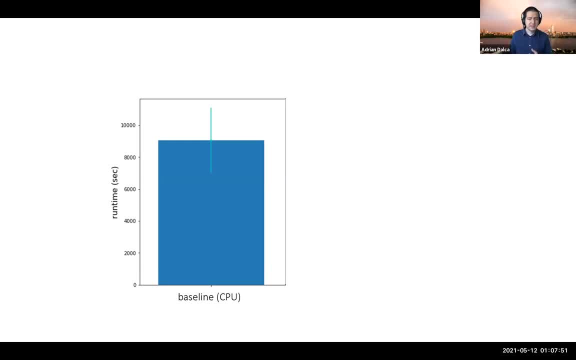 as an internal step, had to do alignment, And so it was just very prohibitive. Okay, so what I'm going to talk about next is the first step, which is the alignment step, And the first step is the alignment step, And the first step is the alignment step, And the first step is the alignment step. 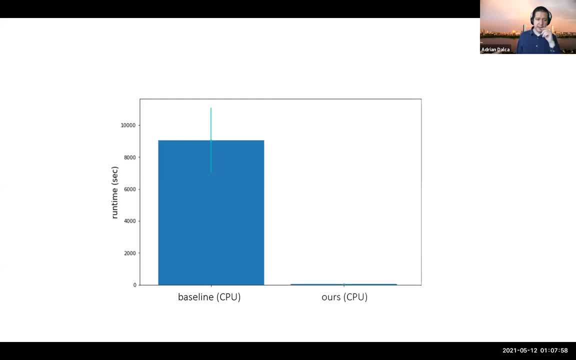 So the alignment step is the alignment step. So the alignment step, the alignment step, is significantly faster. It's that little bar at the bottom there. It's less than a minute on a CPU, it's less than a second on a GPU And that's fast. And I'm sort of jealous of all the students who. 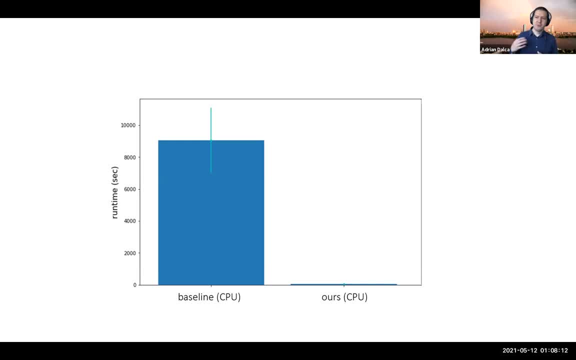 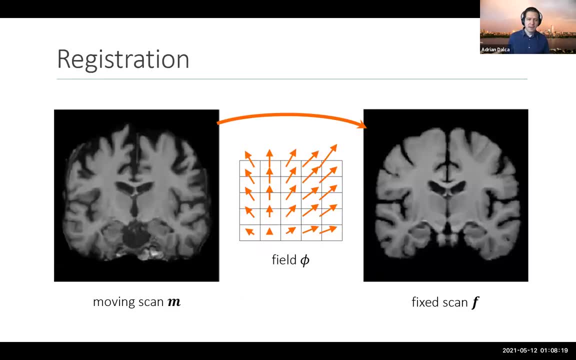 get to use this now, But more than that, it really changes the way we do research in this sort of arena, And that's the part I'm really excited about. Okay, so let me get a little more precise. When I talk about registration, I mean, you're given two images. usually they're big 3D volumes. 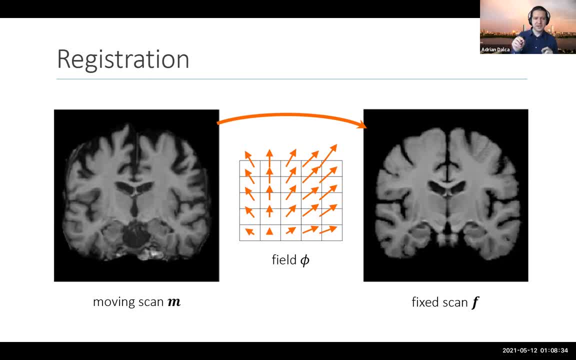 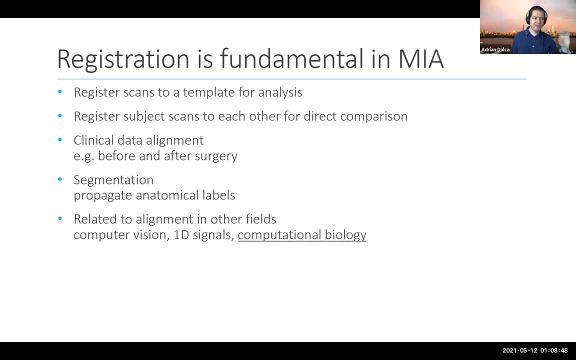 And what you want is this deformation field. At every location, you have a little arrow that tells you how to move one image so that it matches up with another image. Okay, So the goal is this deformation field And just to illustrate, you know how fundamental this is. we align or 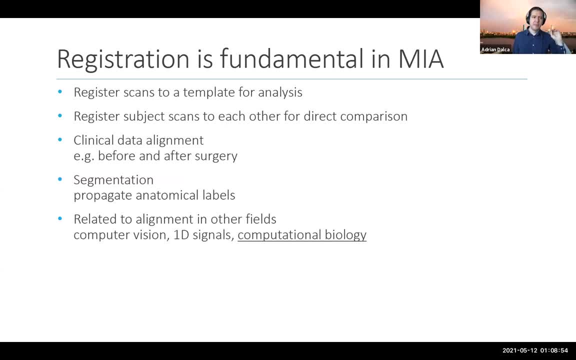 register brains together. We register brains to a template all the time. We register subjects between each other all the time to kind of compare anatomy. We align a subject before and after surgery, 10 years ago to now, to see how something has changed, to see how a tumor has grown. We propagate information from 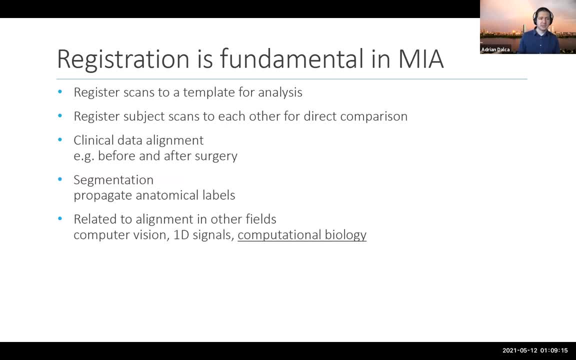 one to another, from one brain to another. so parts of anatomy and that sort of thing, And all of this is related to alignment in a lot of other domains- computer vision, even computational biology, Where I actually got my start in research when I was aligning DNA sequences. So it's all kind of 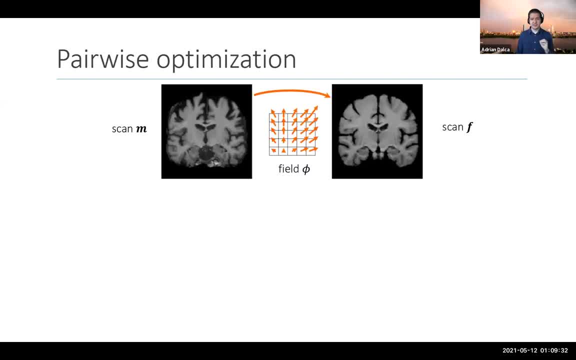 related And so, because of the importance of this, people have done a tremendous amount of work And it all boils down to this one optimization problem. Basically, you want to find this deformation field, that I'll be using this notation a lot, this deformation field, And this deformation field should have two properties. 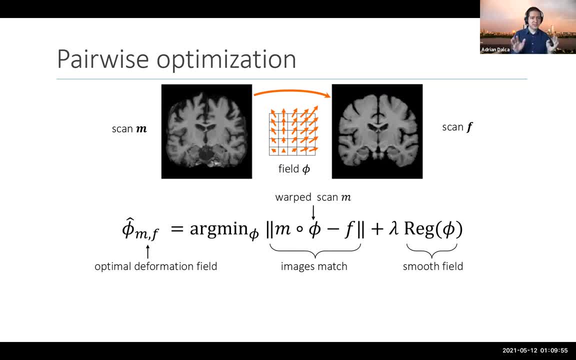 The first is that it matches up images. well, That's pretty simple, right? The second is that it should be regularized in some way. So this is a fairly standard optimization strategy or sort of setup, And over decades people have done better and better image matching terms. better and better. 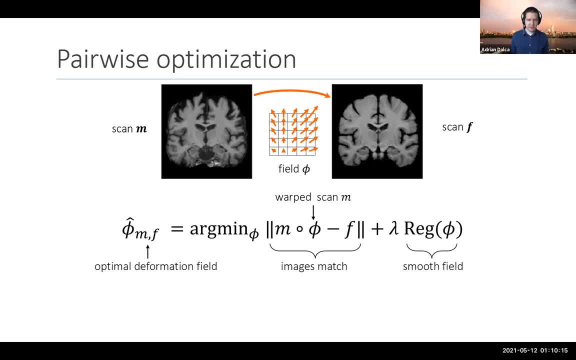 smoothness terms, better ways to optimize the whole thing. It's been a lot of research, So it's great. But at the end of the day, this is a slow process because you get these two 3D images, you pretend you've never seen images before and you start wiggling them around. 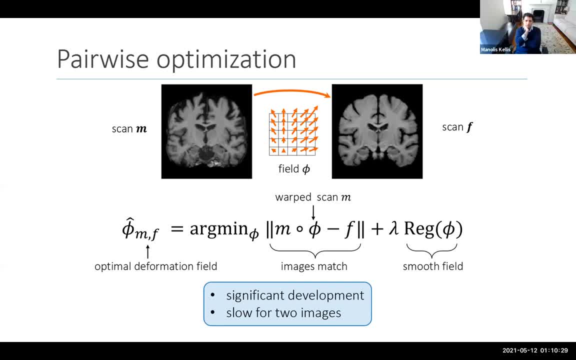 So it takes a couple hours, as I mentioned. Adrian, can I ask you a very general question? I looked ahead at your slides. I couldn't find the answer, So I'm going to ask now, which is if I do image stitching. 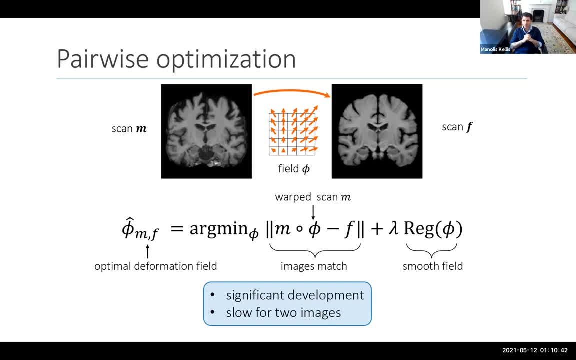 back before our phones did it automatically. it's one thing to warp with a field and it's another to actually match landmarks with each other. So I'm curious whether the field has been looking- and by field I mean the discipline- has been looking at just fields or also landmarks. 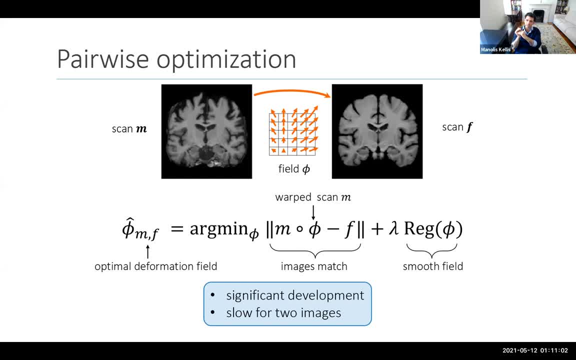 Because the two are very different, Because I could be off by a millimeter in my landmark, I'll know immediately, But I could be off by a lot more in my field and I might not even notice, Right. So, as you say, in some sense they're very related. What I will say, the relationship is and 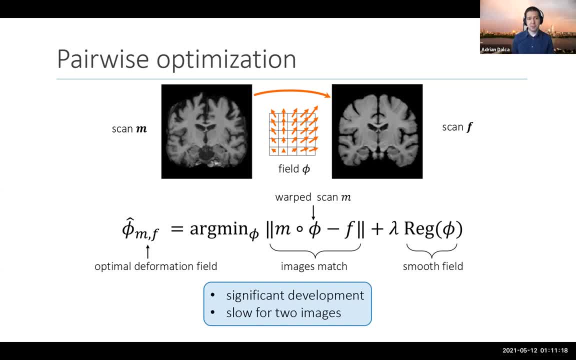 what the field has done is they have used landmarks to match up parts of the brain And then from those they interpolate fields for everything else: Perfect, Beautiful. So it's not one giant field, It's a bunch of subfields in between landmarks, basically, 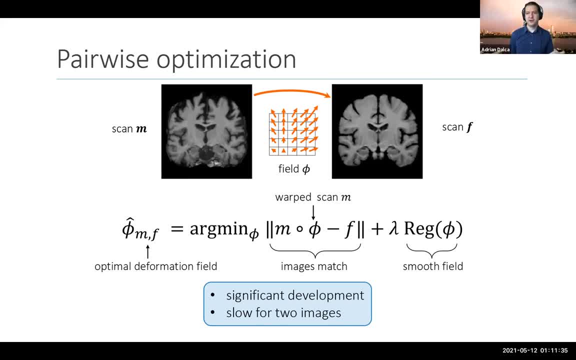 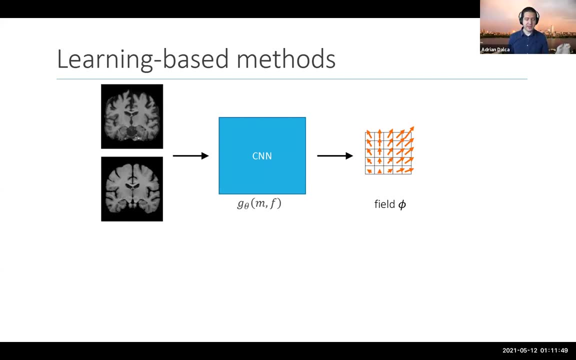 So that is one branch of it. yes, A lot of research is like that, but a lot of it doesn't do landmarks at all. A lot of it is just automatically find a dense field, Perfect, Thank you. So around, I want to say three years ago, 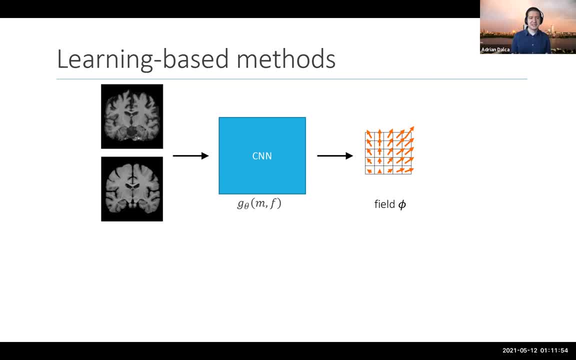 learning-based methods came around and tried to tackle this problem. The very interesting things. as with most learning-based things, I think these methods completely forgot the decades of research that had been done in registration And they said: we're going to treat this as a black box. 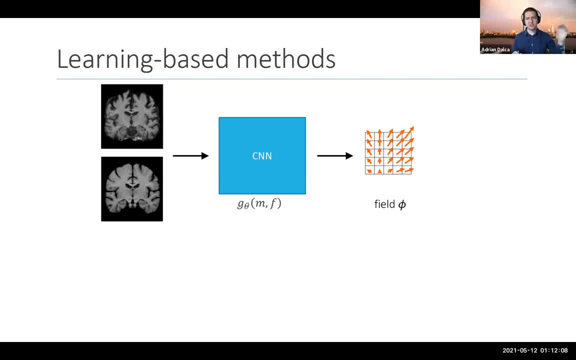 problem. We're going to assume you get these two images, You put them through this black box, CNN, You get a deformation field out And I'm going to use some sort of supervision. What that means is I need to get a really large data. 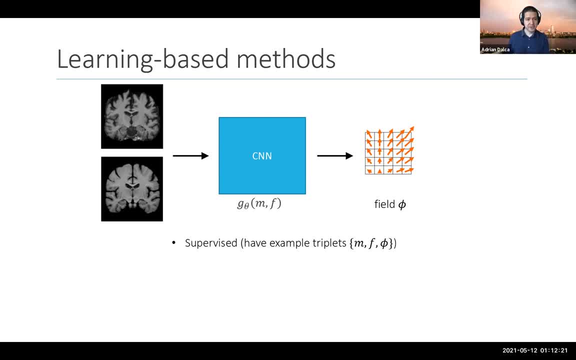 set that has pairs of images and the ground truth deformation field between them, And I treat this as one big regression problem And this was a great idea And there was some work that showed that this is possible. But the problem is we never really 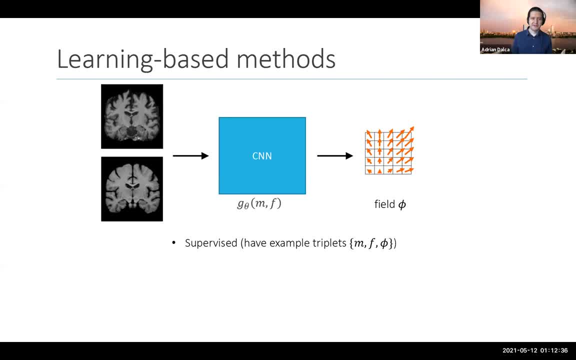 have this ground truth deformation field. You can't really get it from experts because an expert would need hours or days to draw out all these little arrows. They could do landmarks, but that's also extremely costly because this is all in 3D. 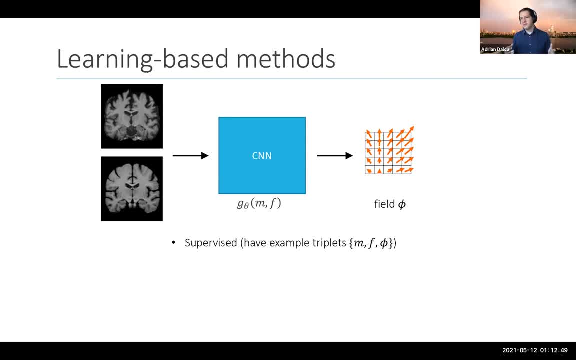 So it's really hard to kind of find correspondences. You could run simulations, But in the end it wasn't a very elegant end-to-end solution that everyone could use, And so this is the part where we kind of came on the scene. 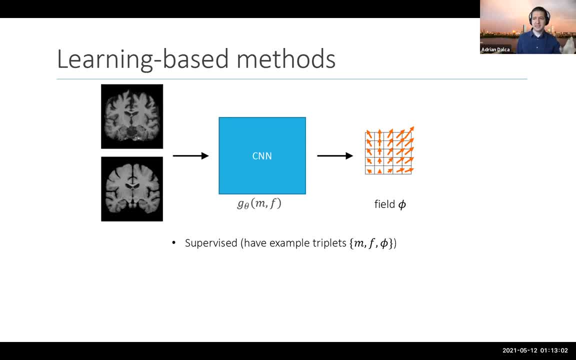 And we thought: well, everybody has one thing which is data, Everyone has data that's unlabeled, And so could we use just these images to learn the same thing. And so this is the method I'm going to talk about today, and all the follow-up work. 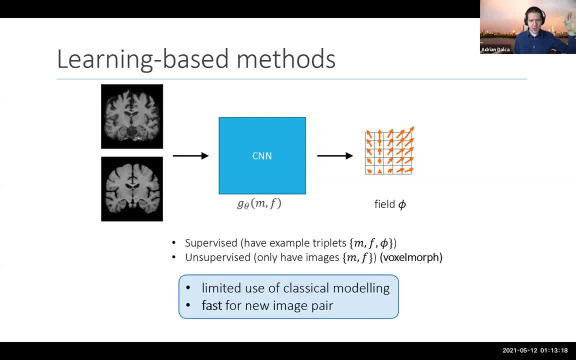 So, as I said before, we kind of came on the scene all of these kind of forgot about all the classical models, all the information and registration methods, But they were really really fast because it was all just a feed-forward neural network. now, 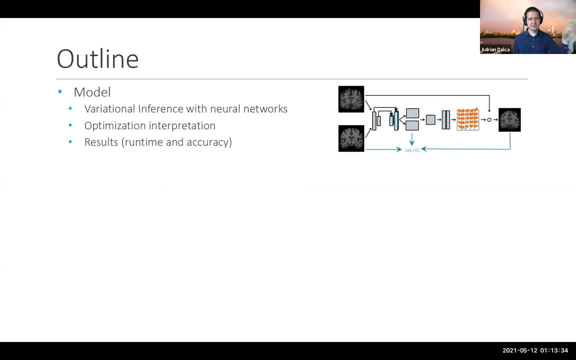 So I'm going to have basically two parts in the rest of the talk. First I'm going to talk about the fundamental model. It's not complicated at all, But if anyone gets stuck at all here, please let me know, because everything that follows assumes. 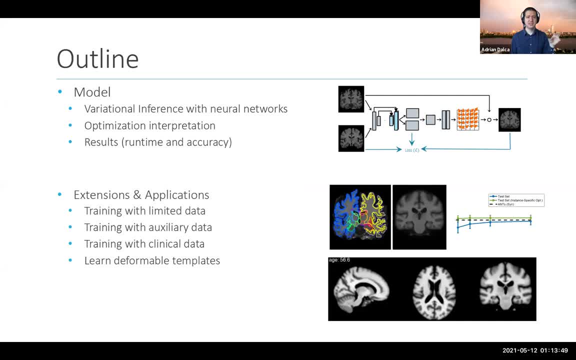 you fully understood it. And then I'm going to talk about a bunch of different projects that we've done since then that I'm really excited about, because they've really opened up the way we think about registration and downstream modeling and work All right, so the framework's really easy. 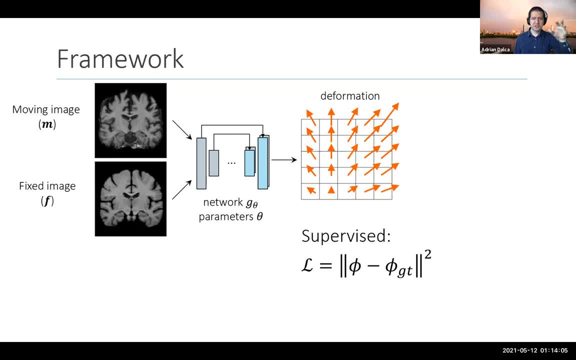 if you have ground truth deformation, You get two images. You push them through a neural network- Nowadays it's mostly a UNet, although I guess now it's changing to transformers or something- But it's just a neural network and you get a deformation field. 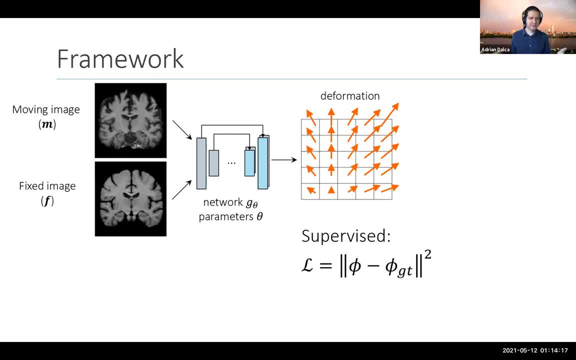 out. And how do you tell the neural network whether it got the right deformation field? Well, you have the supervised data and you take the difference in some way. So let's assume we don't have these deformation fields, How do we tell the neural network? 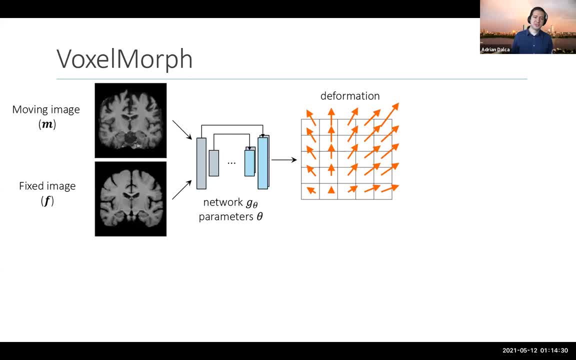 that it did a good job or not, And so this is where we started looking at these classical models and try to borrow from those developments, And it turns out we always had a way to tell the algorithm whether it does a good job or not. 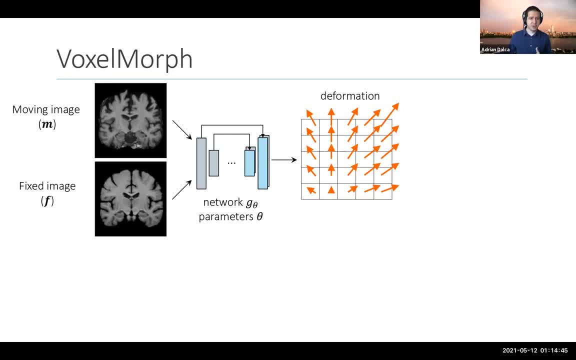 We can just take those loss functions that we used to optimize a single deformation field, and now we're going to optimize And we have a whole neural network based on those fields. So, for example- this is what I talked about before- You have a loss function that says well, 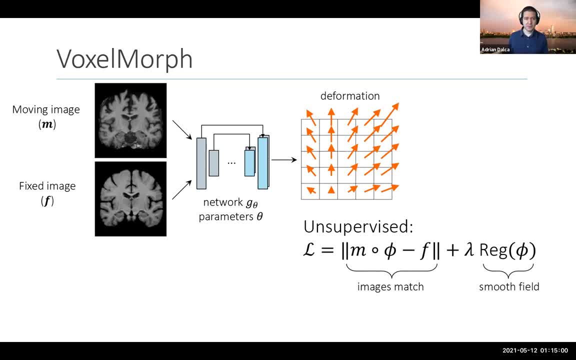 this field better match up the images and it has to be smooth And you don't just apply it to one image but you apply it to all the images in the data set, So you keep feeding random image pairs to your network. The deformation field has to have a low loss under this. 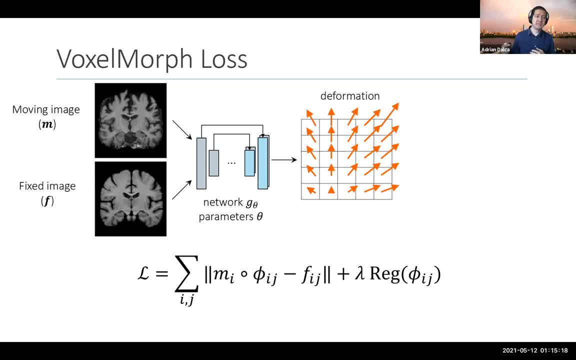 And again, I'm not optimizing deformation fields here. I'm optimizing a network. It gives me deformation fields, So it's borrowing from classical methods in that I'm using those loss function-based intuitions, But of course I'm optimizing neural networks. 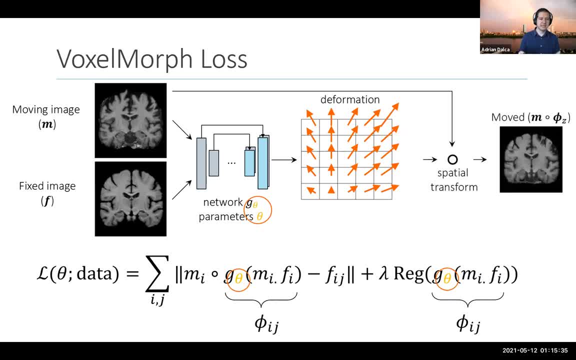 so I have to use, or we use, stochastic gradient techniques and that sort of thing. Now, how do we make sure these losses are differentiable? Well, for some of them it's pretty easy. For some of them it's a little harder. 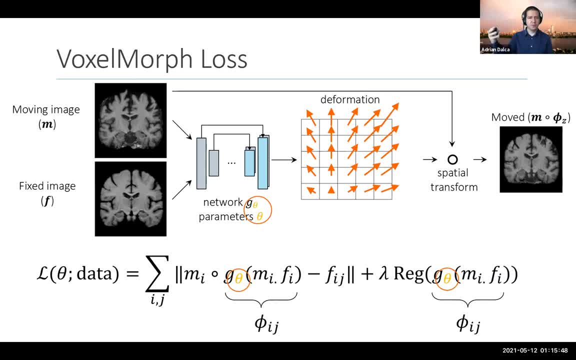 But at the end of the day you take the deformation field, you actually warp an image. The way you do that is just linear interpolation really- And then you have your two images so you can compare them in fancy ways or in simple ways. 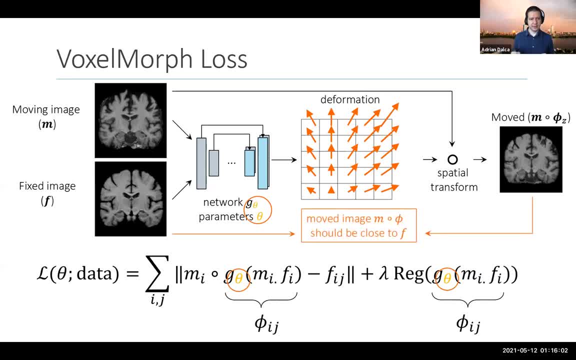 And you can check whether your deformation field is smooth by taking spatial gradients. So it's actually pretty easy to implement this whole thing. Again, use stochastic gradient techniques And at the end of the day, you'll learn this big network that outputs this deformation field. 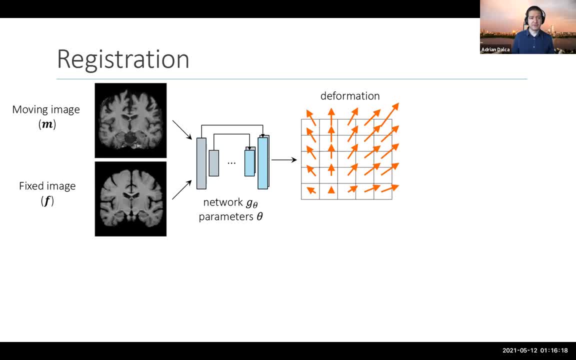 And the cool thing is, you've never really needed a ground truth deformation field. It's an example, So any data you have lying around you can train this network. Now, underneath all this, we published a bunch of papers that show that there's actually really. 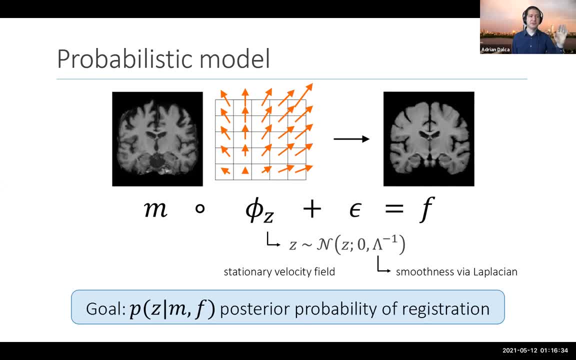 nice theoretical connections to a bunch of other things, for example to probabilistic models. Our field for a long time developed these probabilistic models that offered you all kinds of elegant connections between images, between deformation fields, uncertainty estimates, all that sort of thing. 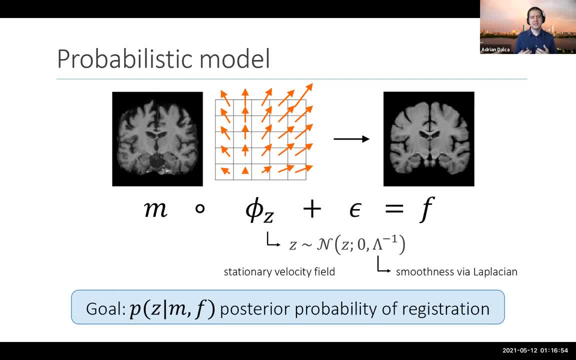 I don't want to go into detail now but I'm happy to take questions. But essentially, if you set up these probabilistic models and you try to do inference and you try to approximate that inference with neural networks, you end up to this solution. 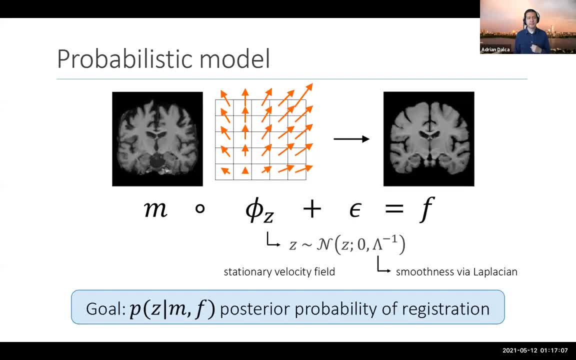 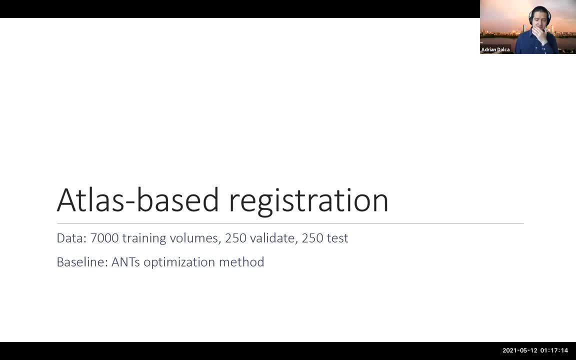 So that's pretty nice because you have some sort of grounding underneath. So any questions on that setup Looks good. OK, So this, So does this actually work? And actually it's not a trivial question, but the first thing we cared about. 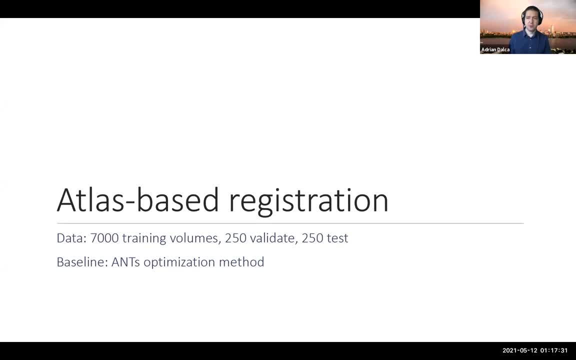 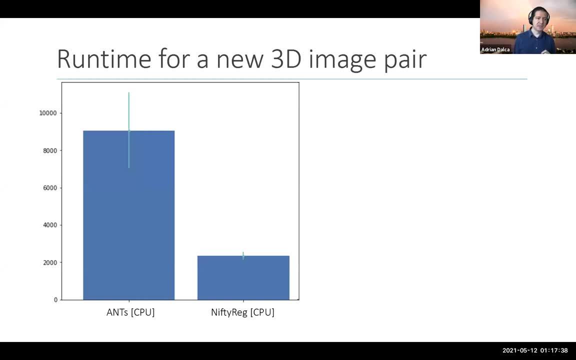 was: how fast is it? Because the whole kind of problem was that things took too long And so we tested a bunch of optimization baselines You got. some of them took two hours and they were very, very, very good, And some of them maybe had slight losses in accuracy. 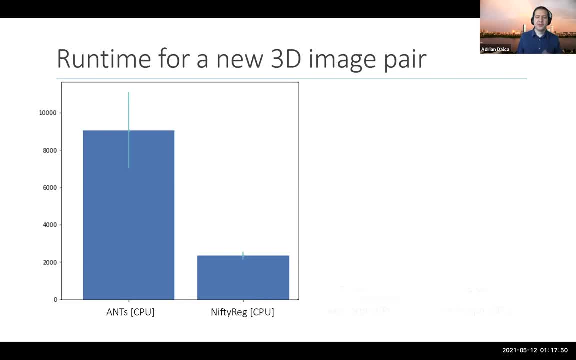 but they were 10 minutes, 20 minutes, So that was better. But then we ran voxelmorph at the time, So this was 2 and 1 half years ago or something. It was less than a minute on a CPU. 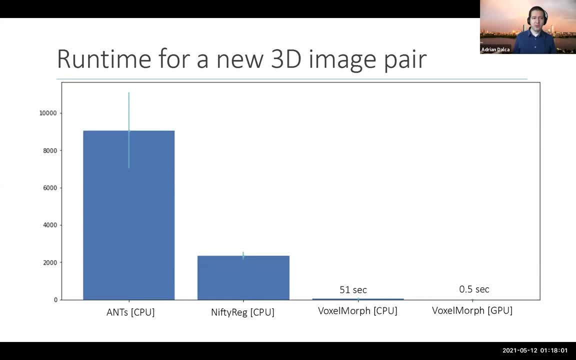 less than a second on a GPU. So that was cool because you could get the whole output very, very fast. It's obviously faster now, But how do we know if we actually do a good job And so the way you actually do it? 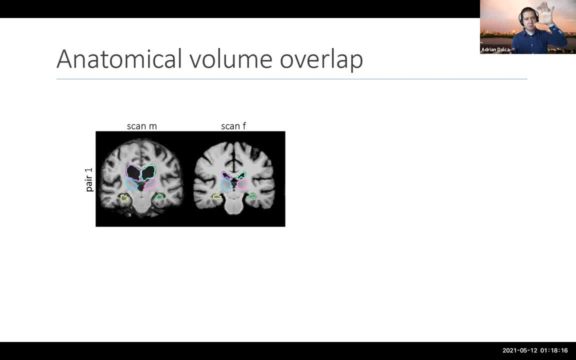 so if you want to just align one image, take one image, morph it and compare it to the second image, OK, You might think you're doing a good job, But realistically you might not, because the deformation field might not be smooth. 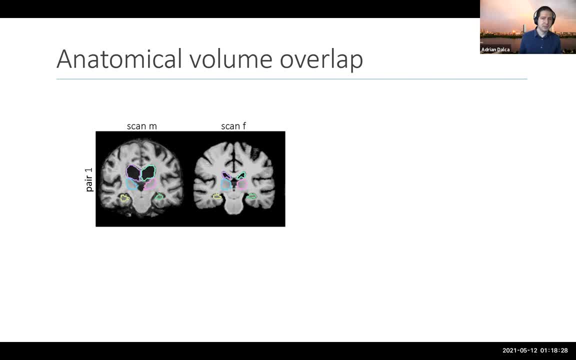 Maybe it's copying some pixel from the background and it's moving it in the middle of the brain. It's really hard to figure that out, And so what we actually do is we outline anatomy for evaluation. So here you can see that I've created this. 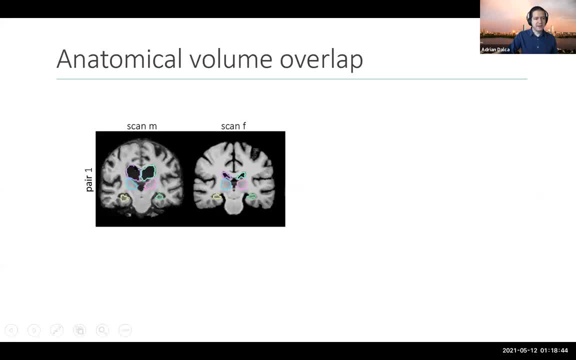 Oops, sorry about that. You can see that I've created these outlines here around the ventricles and the hippocampi, And then I'm going to go ahead and do a little bit more of this. I mean, these are just structures in the brain. 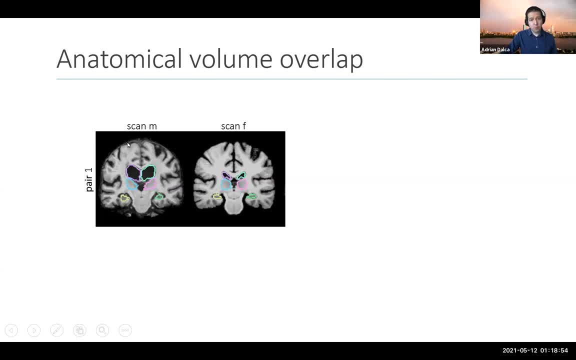 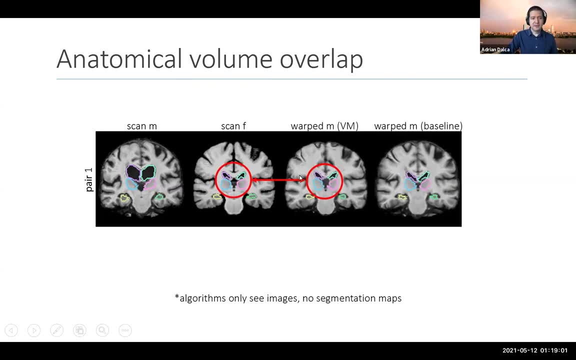 I've done it in the moving image, I've done it in the fixed image, And now when I work this first image, I check that the anatomy matches up, And so you can see visually that they kind of match up right. The ventricles look about the same, and so on. 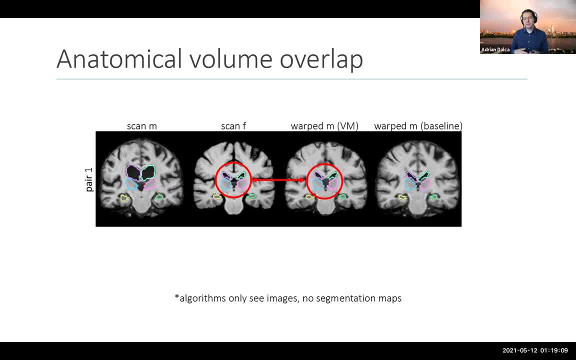 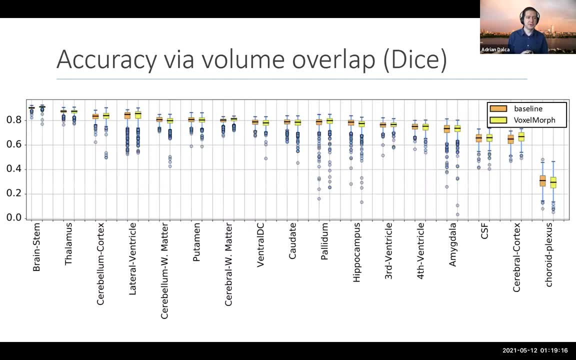 So qualitatively it looks like it's doing a good job. But now how do I quantitatively look at this? Well, I measure. I do some sort of volume overlap measure right. So here higher, Here is better. 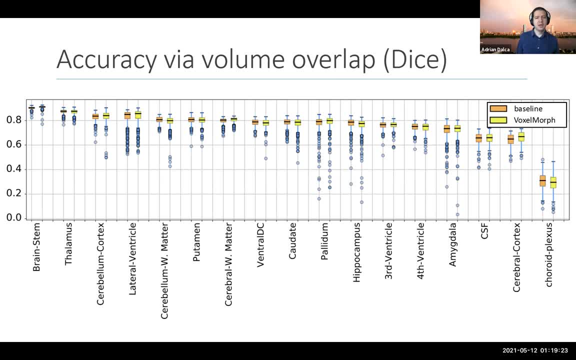 On the x-axis is a bunch of different anatomical structures we outlined, And the bottom line is that this algorithm, voxel morph, is basically the same as the baseline, while it's orders of magnitude faster. So what's happening here is that this neural network 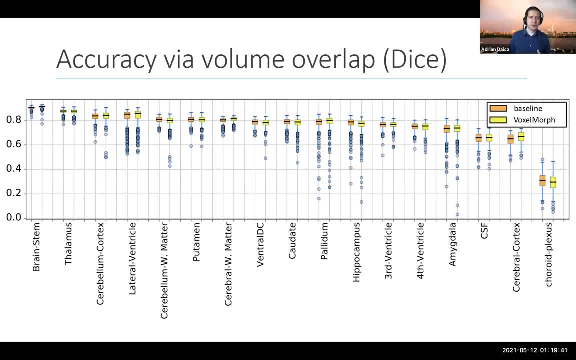 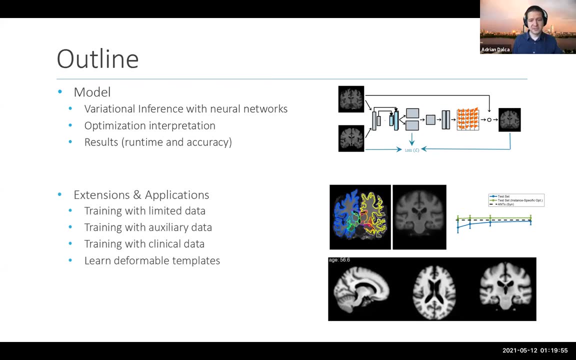 is able to estimate the output of an optimization procedure. So that's pretty cool because now we can do all kinds of modeling With this approximation. So I'm going to move on to all these other kind of things. First, we did a bunch of analysis on what this means. 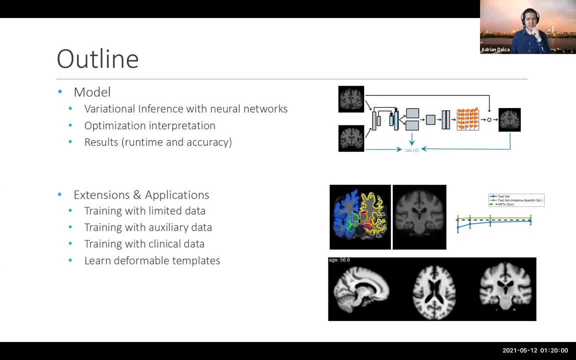 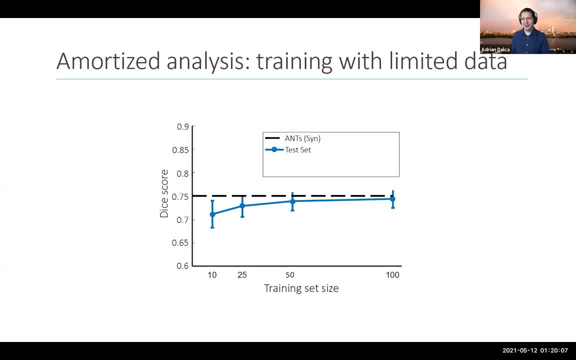 And then a few kind of small projects, All right. So the question that we always got. So when we first train voxel morph, we just gathered all the data we could because we thought, well, neural networks, Neural networks need a lot of data. 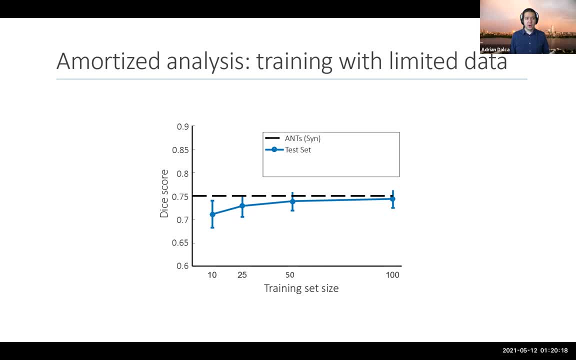 So let's kind of train Really, Really large, with really large data. But everyone came and asked us: well yeah, but I only have like 50 images around, Can I still use your neural network? And so we did this analysis. 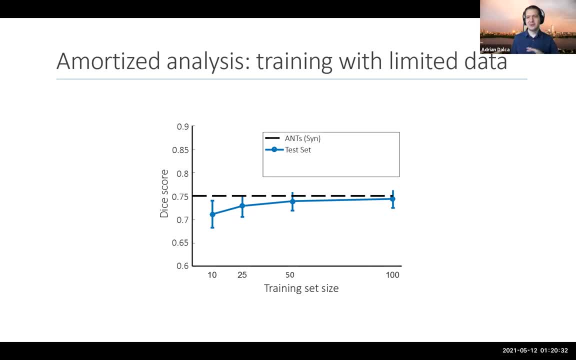 Now, at the time, we had no bells and whistles, no data augmentation, no, nothing fancy, And we trained four models with just 10 images: 25,, 50, and 100. And we found that you get pretty close to the state of the art. 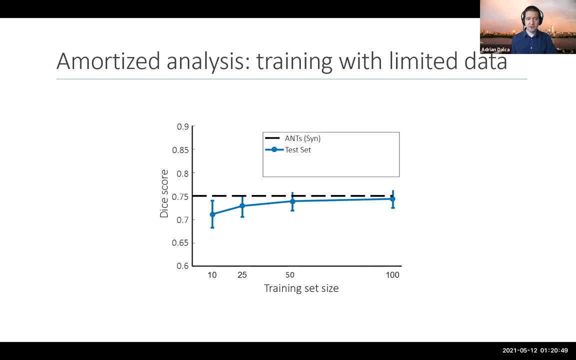 even with just 10 images- Not perfect. You need 50 or 100 to really get to the state of the art. But with just 10 images you got close. So that made us think. well, if the deformation field is almost 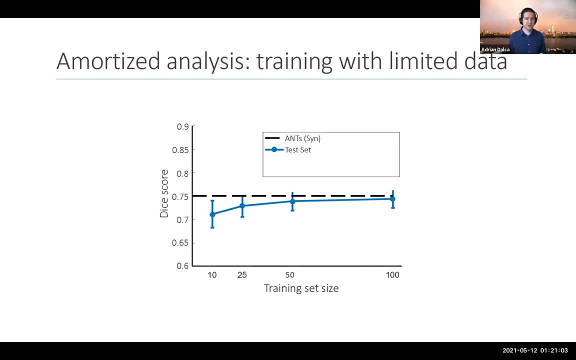 right. couldn't we just take that output from voxel morph and just optimize it a little bit for just a few seconds? Just wiggle those vectors around And it turns out that if you do that for just 20 seconds you get to the state of the art or better. 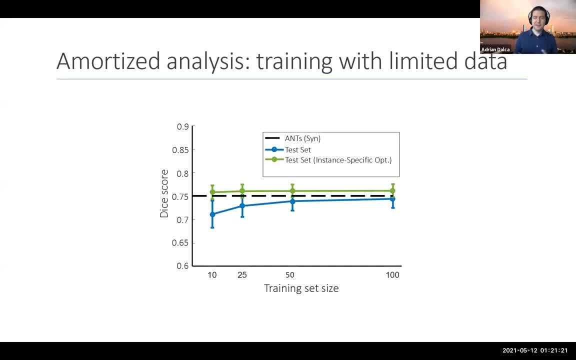 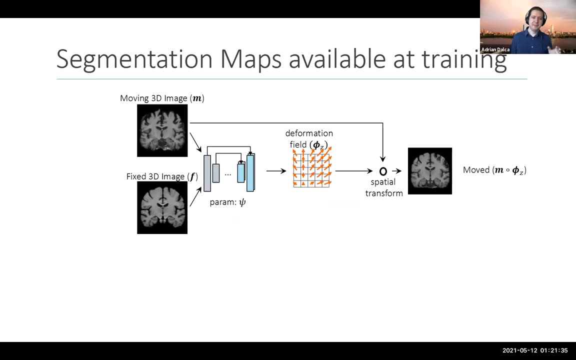 In other words, voxel morph is really useful even when you have just 10 images And most data says now you have at least 30,, 40, 50. So that was good, because now it's applicable. The other thing we kept seeing is that people always said: 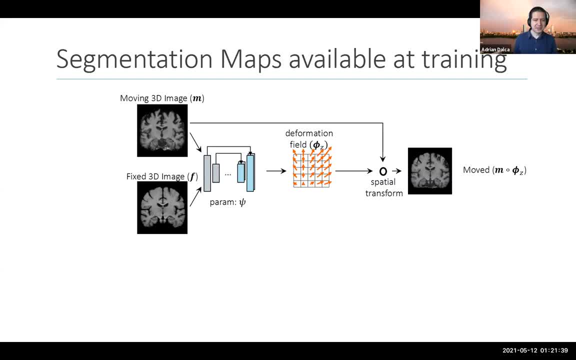 well, I'm registering these anatomies, Let's say I'm registering this brain, but I don't really care. I really just care about the hippocampus because I want to correlate it with genetics or something. I don't really care about the whole thing. 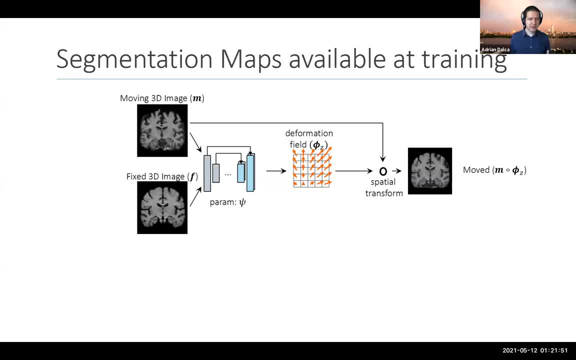 I don't care about the whole brain. So how do we tell the algorithm that you really only care about the hippocampus? In practice, classically, you would need to outline the hippocampus in your test data, And so, if you have 5,000 images, you. 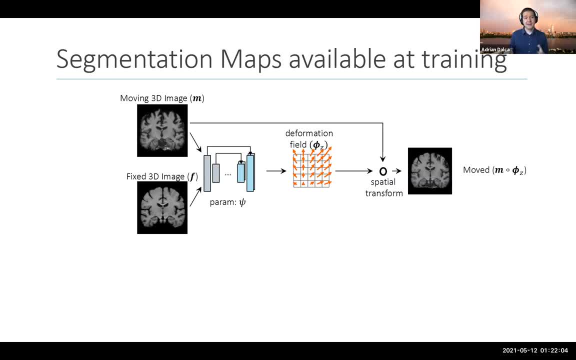 have to outline 5,000 hippocampi. That's a problem. But what we thought is: well, maybe if you have just a few images with outlines, maybe you can use that during training, So the networks never see the outline. 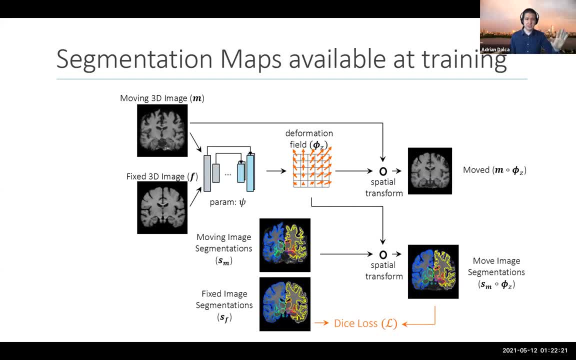 So the labels? they only see the images. This makes sure that at test time the network will only see the images, But during training we're telling the network: well, you've got to do everything you used to do, But now you also make sure that the labels of the hippocampi. 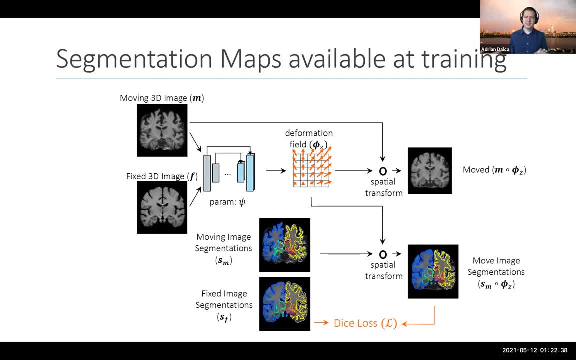 match or whatever labels you have. And what this is teaching the network to do is, in general, it's teaching it to register, But it's also teaching it where the hippocampi is and to spend more of its energy there. And by doing this at training, now again at test time, 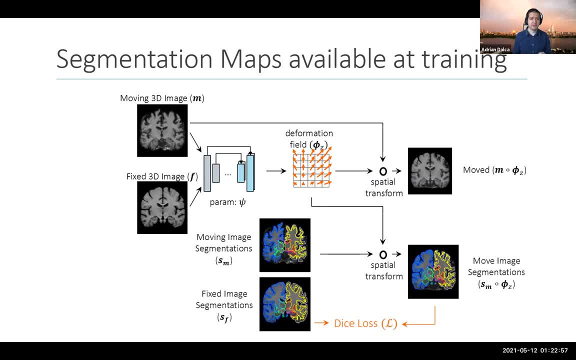 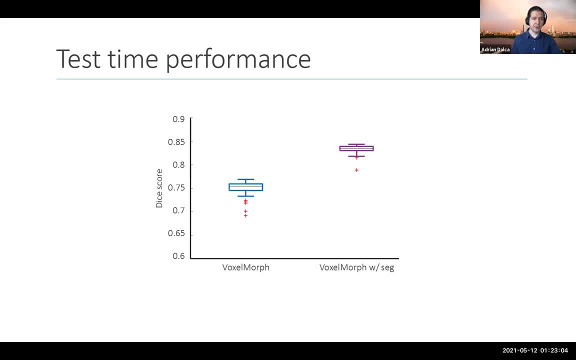 we just give it images that don't have hippocampi labeled or anything. But for the first time we saw that we can actually significantly improve over the state of the art right, So 10% better than the classical methods we're able to do, which is substantial right. 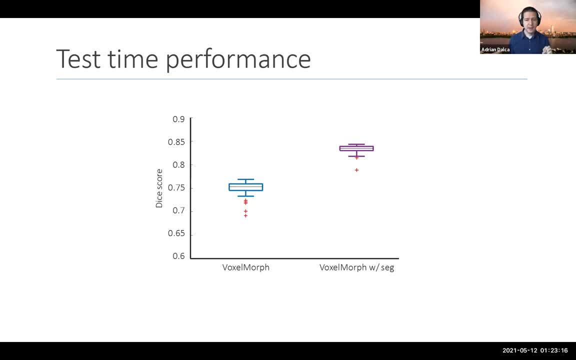 Here there's obviously no p-value question or anything. All right, Thank you. And this is because the network underneath the hood is learning this kind of joint task. It's learning to align, but it's also learning kind of a soft segmentation. 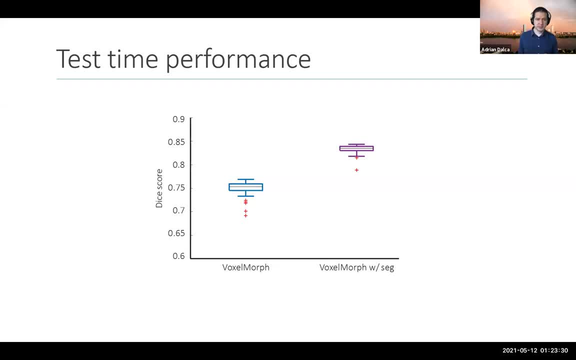 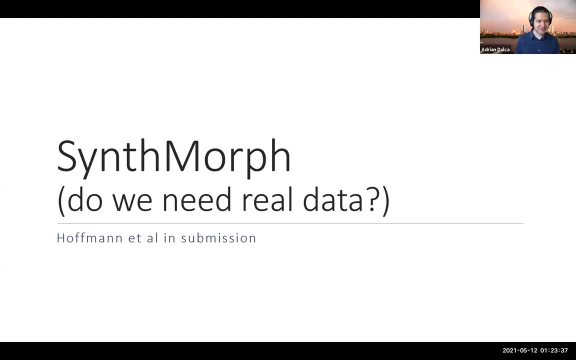 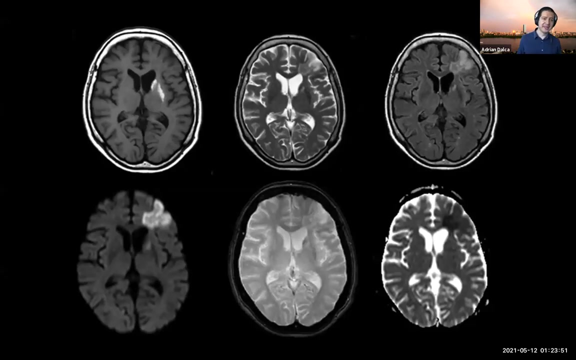 underneath the hood And so it's able to do this. Moving on to sort of more recent projects, And again it's related, So we had I'm going to go into a project that basically solves two problems. One of them is that medical images are actually. 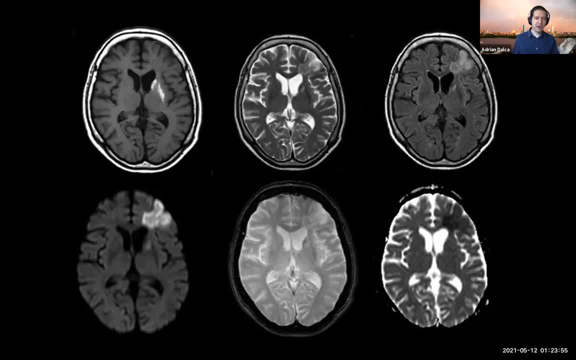 incredibly diverse. Here I'm showing you MRI of the brain, And these are six different types of MRIs. They're all of the same brain, They're all what you would refer to as MRI, But they're what we call different modalities. 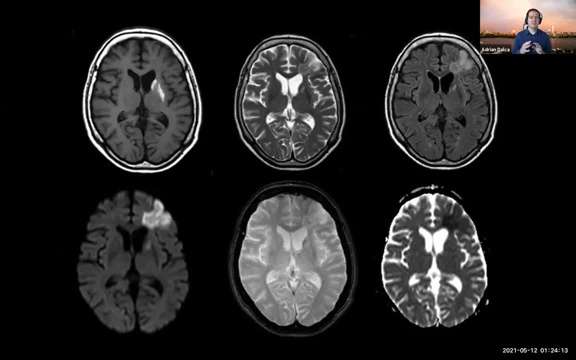 So, even within MRI, your images look different, And so So we know that networks have this issue, that when you train them, you're very susceptible to the data you've trained with, And generalizing to other data is a challenge, And so if I train on this first modality, which a lot of people 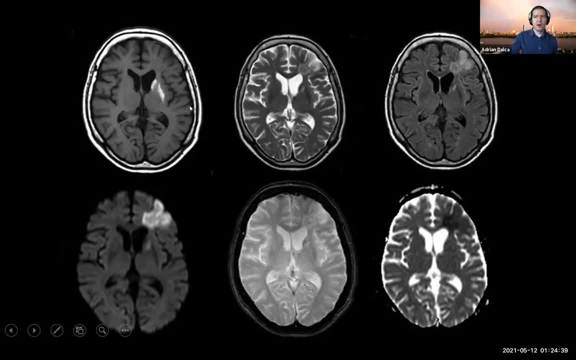 actually tend to have, my networks will probably never be able to register or align these images or these images or even modalities Between each other, right, And so this is kind of disappointing, because if you release a tool in practice to clinicians or scientists, the reality, 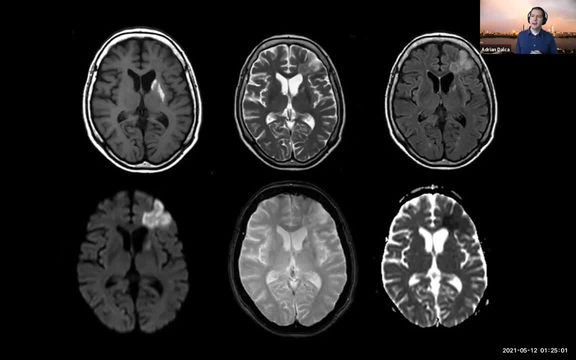 is, it's not going to be very useful, even though it's fast and it gets this accuracy, and so on. So we thought, OK, how do we get past this? Now we could try to gather up a lot of data and try to train one big model, but that model will still never. 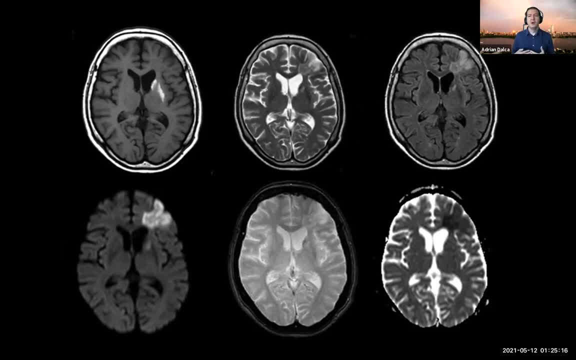 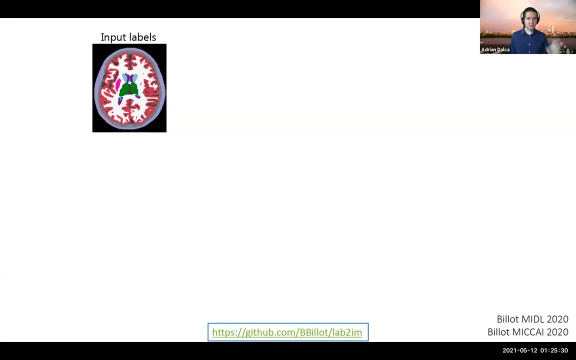 generalize to new data and new sequences that people come up with, Or to CTE or something right. So how do we make these networks robust to things that they haven't seen? And that's when we came up with this idea of essentially simulating brains. but the idea was: 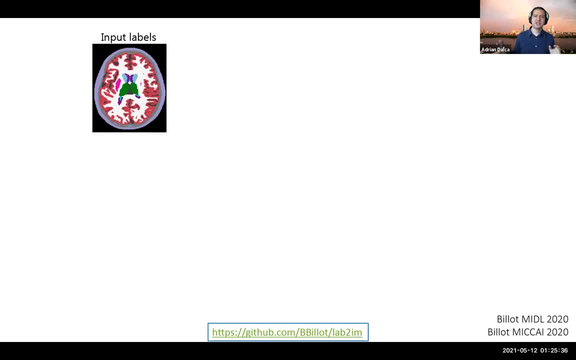 to simulate brains so diverse, so extreme, so unrealistic that the network will essentially see so much variability and contrast that it will decide to ignore it. So let me show you what I mean. But, Adrian, I mean this has been basically. 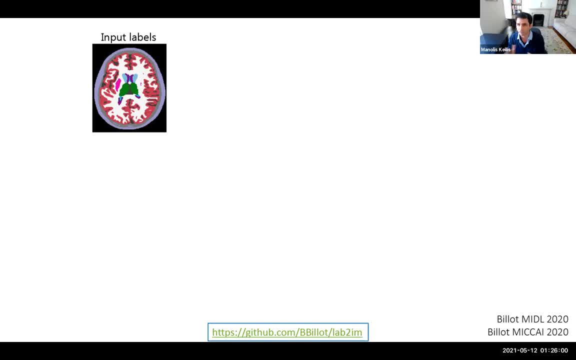 there's many schools of thought here. So one of them- in the sort of self-driving cars, for example- has a physical model of the world and then simulates novel scenes and stuff like that within that to then train the model. Another one basically says: I have an existing world. 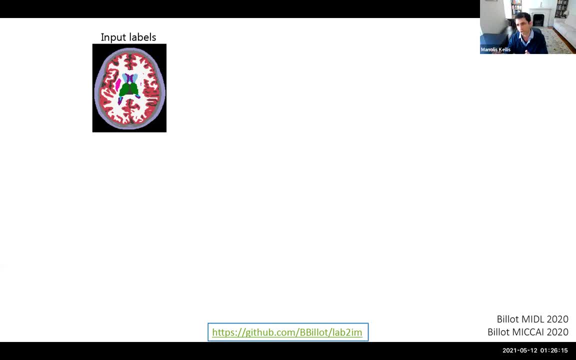 and I'm going to modify that world according to a set of transformations: Yep, Yep. In both cases, the transformation that you put in and the types of scenario that you put in teaches the model about the diversity that it's going to be able to learn. 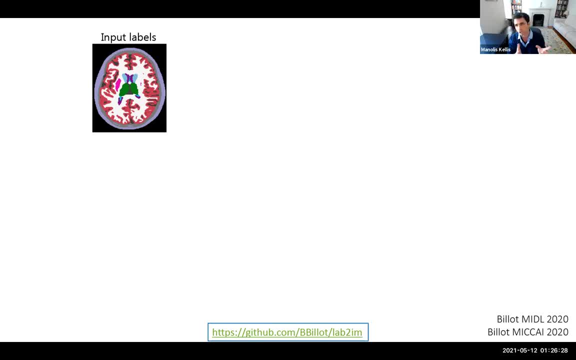 I'm curious: how are you driving those transformations and how much does that influence what you're learning? Or are you just trying to be not necessarily physically relevant but at least diverse enough that the model learns to be robust to that variability, Right? 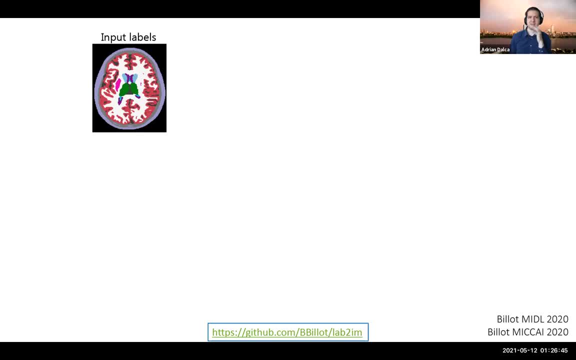 So we did experiments. We did experiments comparing, simulating really diverse crazy data that you would never see, simulating data that we think is realistic, and taking existing data and just modifying it the way I think you're describing, And the problem with the last two. 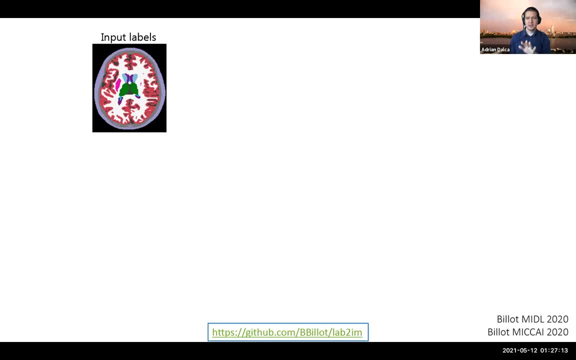 is that they are still in some ways constrained, Right? So if you're simulating it, you're simulating data that's somewhat realistic, you will often well, at least in our experiments, and what we were able to do, we weren't quite. 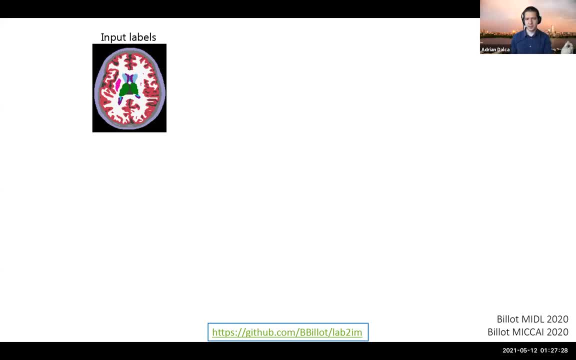 able to get the network to be quite as robust, especially to outliers, If you start with realistic data and try to modify it. that was significantly harder for us because basically we weren't- again, it was an issue of we weren't able to expose the network to enough variability. 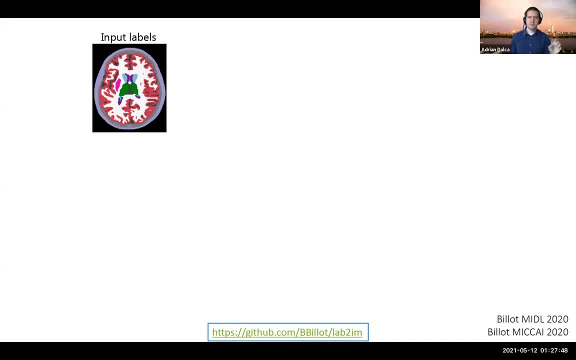 if that makes sense. Yeah, Let me also maybe go through this slide and see if I don't answer. So what we do need for this first version of the slide is some labels, some image labels. Now you can download these from the internet. 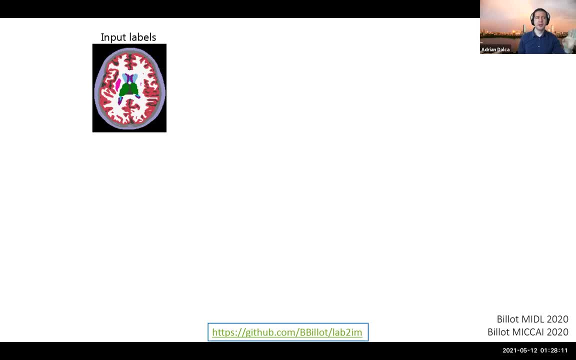 because some brains have been labeled at some point right, And so you can just download just the label maps, no images, And so what we do is we randomly deform these images. So now we're generating kind of anatomical variability. We randomly fill in values, intensities, 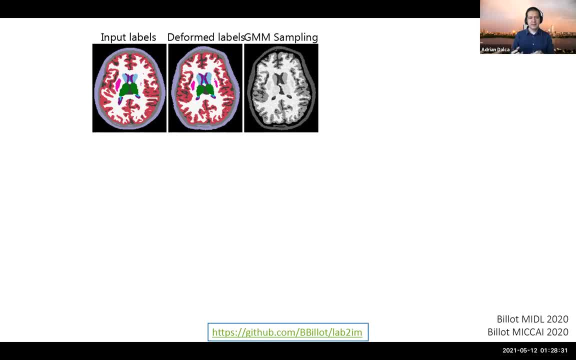 with a bunch of different noise patterns inside the label. So now we've got something that kind of looks like a brain. We add all kinds of effects. Here I'm showing just a blurred image, But we actually have a bunch of different effects we add. 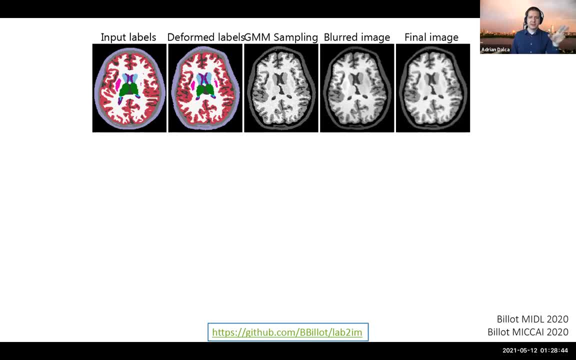 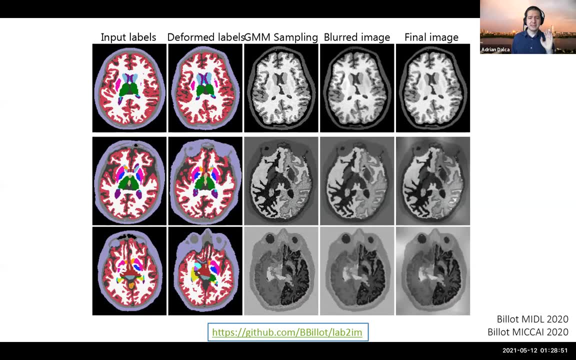 kind of like errors you might get in an MRI And then you get this is your final image. That's how we simulate data And we simulate crazier and crazier data. These are images you would never see, you would never have in the same tissue. 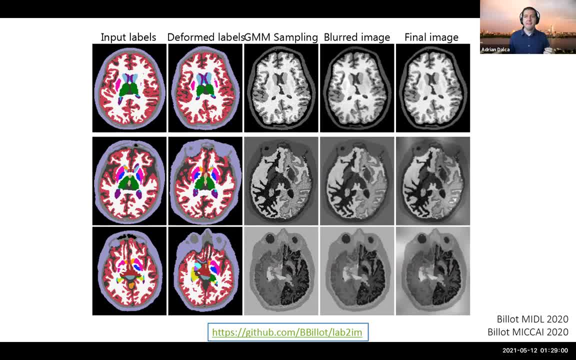 black on the left of the brain and white on the right on the brain. But the point is that the network's going to be exposed to so much variability that the real data will be included in there somewhere. So that was the idea, And so we started kind of doing these experiments. 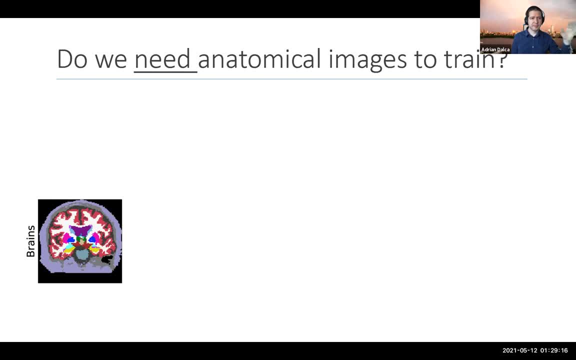 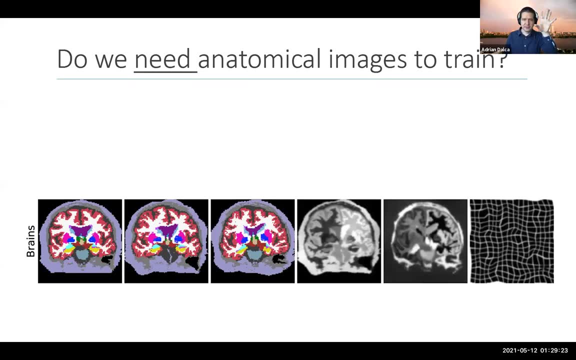 for registration. I mean, first we had some segmentation, We had some segmentation papers, But then we looked at registration And you take a brain, warp them in two different ways, fill in different values, different intensities, And that's your simulated data. 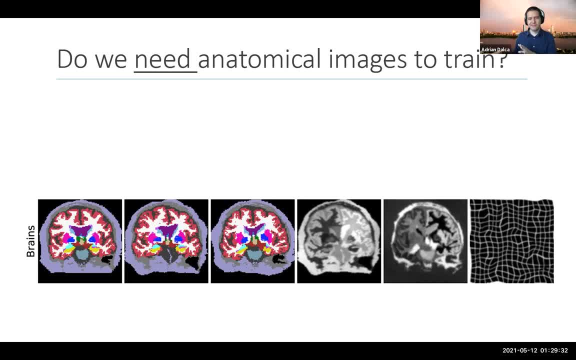 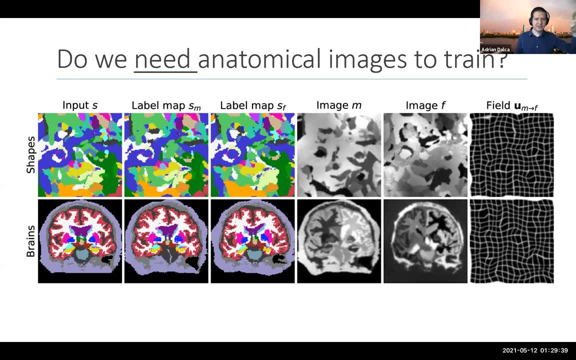 But then at some point we thought: well, we're really not really that constrained to the brains. What if we just fill in random shapes? So start with some random blobs, deform them in two different ways, fill in random intensities. 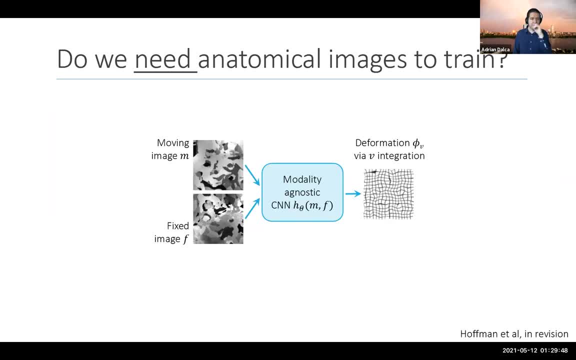 And that's the data. So we push these images through the model And this gives us a deformation field. Now how do we tell whether this deformation field is any good? It's really hard to tell by looking at the images, because the images have been sort of filled in. 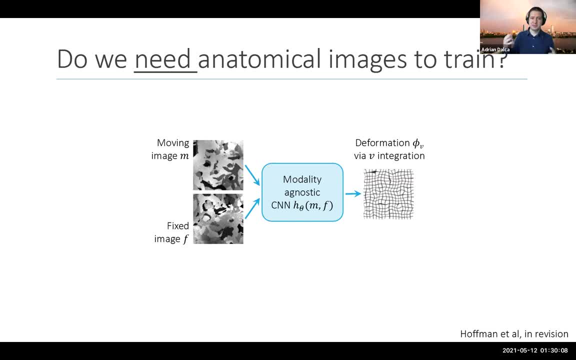 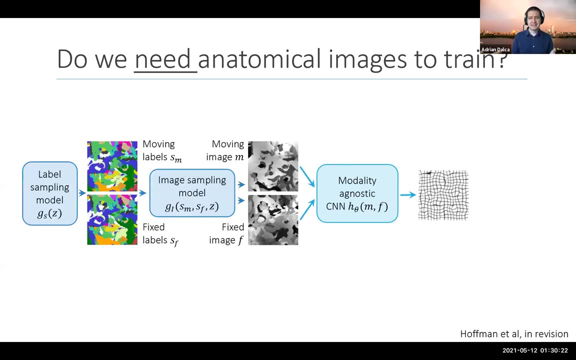 with very different contrasts. So you have to come up with these statistical measures and so on. But remember, we simulated these images starting with some segmentation maps. So we can always say we can always give the network just the images, But we can ask the network if it registered the segmentation. 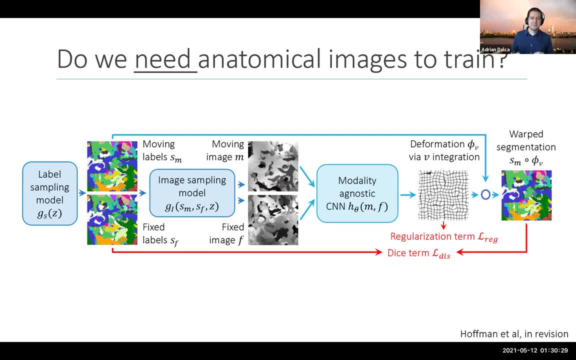 maps well, And this makes sure that the network essentially learns to figure out shapes from the images, But it also learns to ignore the exact intensity It sort of figures out: well, the intensity doesn't matter, And that's the invariance we're trying to create here. 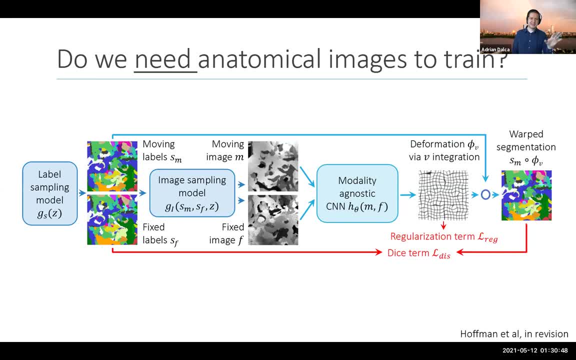 So that kind of sums up what we did. So we ended up training a bunch of different models. We trained some voxel morph models, starting with a particular type of MRI but then trying to synthesize variability around that type of MRI, And then we tried two different versions. 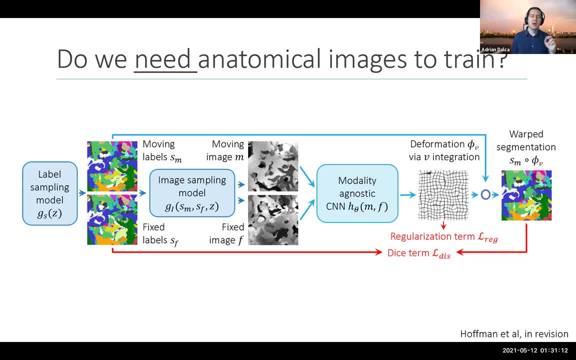 of this model, which we call synth morph, because we're synthesizing beta, Two different versions of this model, One with random shapes, One with random brain images, And so that's what I'm going to be showing here Now. red are classical methods. 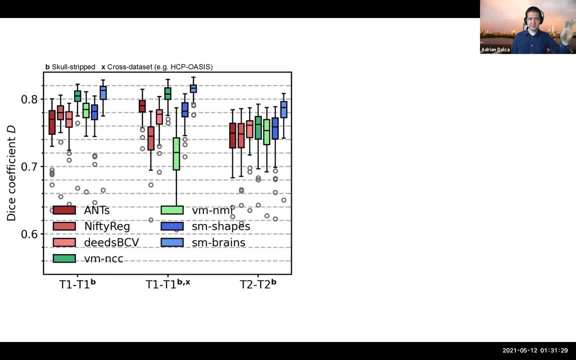 Green are voxel morph models trained with some variability, And blue are the synth morph models. But here what I'm registering are images of the same intensity, Same intensity I trained with and also same intensity when you register, image one and image two are of the same intensity. 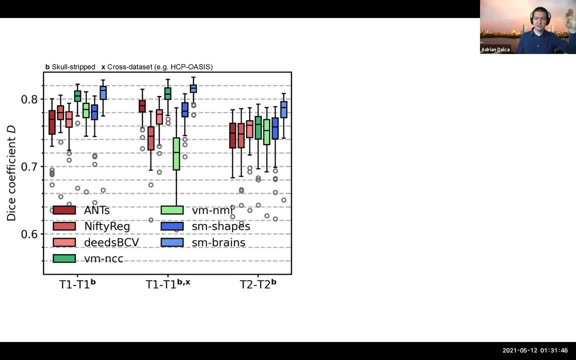 So classical models do. Well, we've pushed voxel morph to do a little better now because we've added some variability and some robustness, And also we've kind of gotten better with these networks And the models we trained, the synthesized models that never 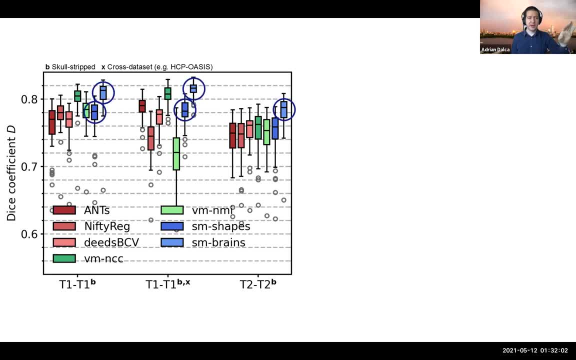 see any real data, but they either have simulated blobs or simulated brains. do roughly the same as voxel morph. They do better than the classical models, And the model that's trained with completely synthetic brains does better than every one, But roughly the same. 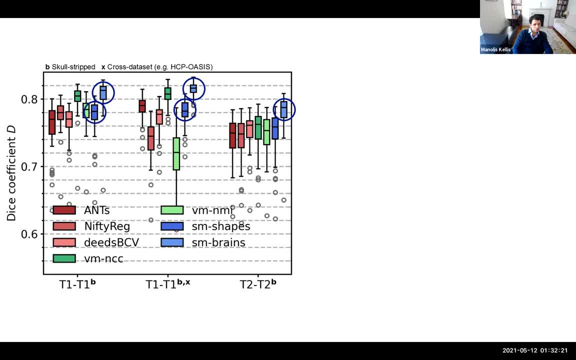 Not really a big deal, But of course the light green voxel morph. they're just really poorly in the middle one Right. So we trained two versions. One of them is trained with this metric called normalized cross correlation. that we know is a very robust metric for same contrast. 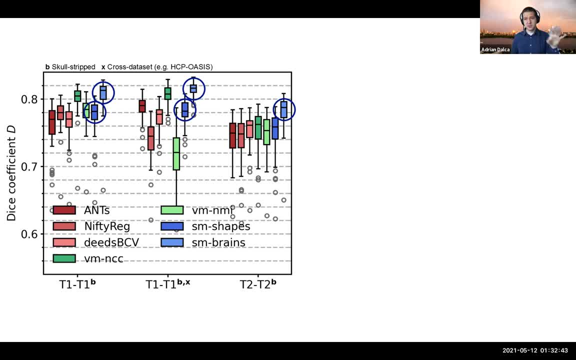 And then we also trained with this other metric called normalized mutual information. OK, Yeah, in general that is a good metric, for within contra, within different contrasts, but within the same contrast it's not as good. what's happening is it's- uh, it computes these statistics. i mean, you know mutual information right, so it computes these. 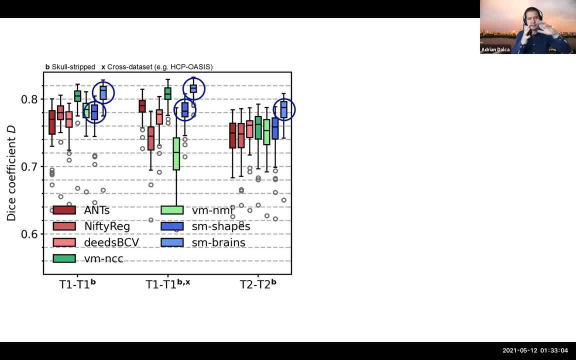 approximate statistics and to do that, it kind of uh needs this, it's kind of it needs this like field of view and it's very approximate and so it's basically the bottom line is it's not as robust, if that makes sense, right? um, but again, it depends what you want to do, right? we know these. 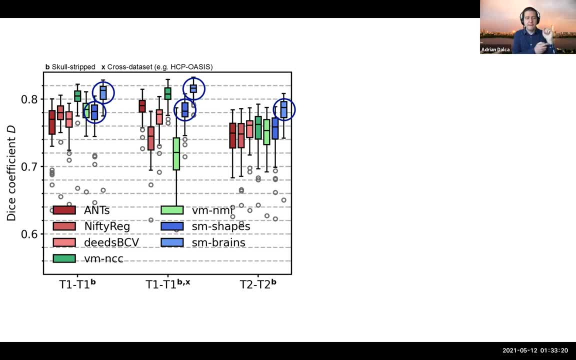 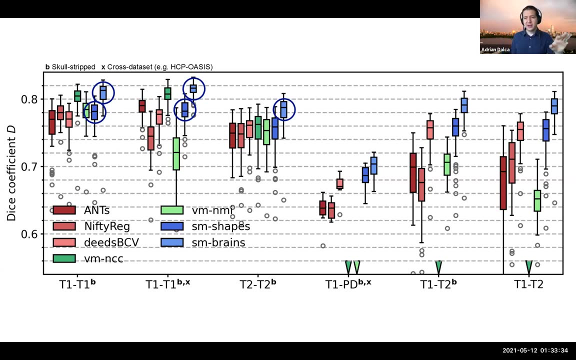 are within contrast. so training with ncc makes more sense. but what happens when we start looking at modalities? we have modalities we haven't seen and trying to register between modalities, and so this is what happens: the classical methods they don't do quite as well, and part of the reason. 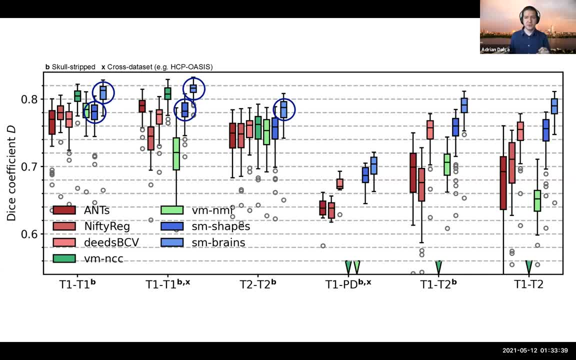 is exactly what i just said. the. the metrics that force us to look between modalities are are these statistical measures, and they tend to be nowhere near as accurate. they still get the right idea, but you start suffering the voxel morph models, especially the one that was trained with. 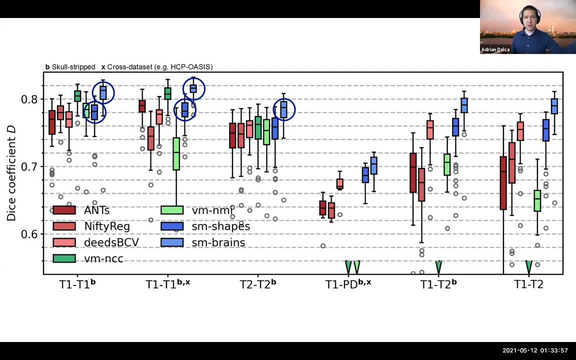 ncc, the, the deep green one that did well within modality, just completely collapse because they've never seen these images before, they've never seen these modalities before, and so it just crashes. it's these are real images. now, these are all. sorry, i should have made that clear. all real images. 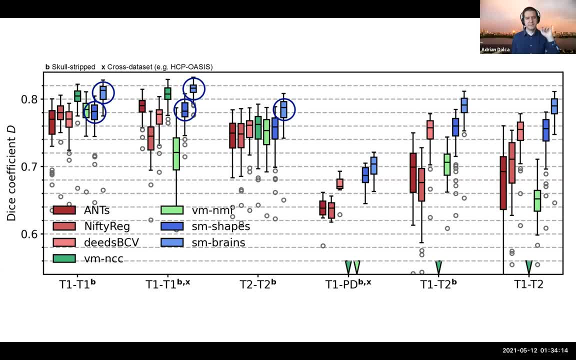 that's amazing. all real images and um the synth morph data models are remarkably robust and i have to admit i was surprised. so um a little bit of a converse question, which is: is it possible to make that training space so large that the real images you know are kind of such a small subset that 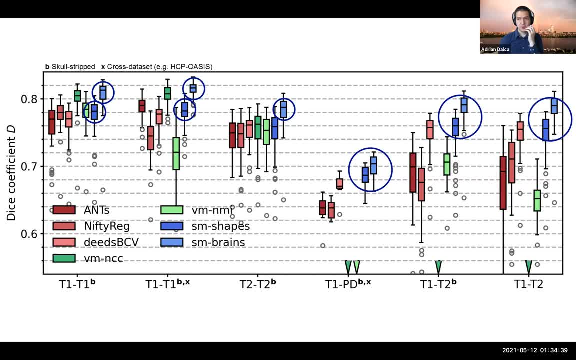 you're not really capturing their features anymore. yeah, so it's definitely a very good question and the answer is that, um, we see this happening as a function of model capacity. so if you have extremely diverse data simulated and your model is fairly limited, you have this issue where it does. 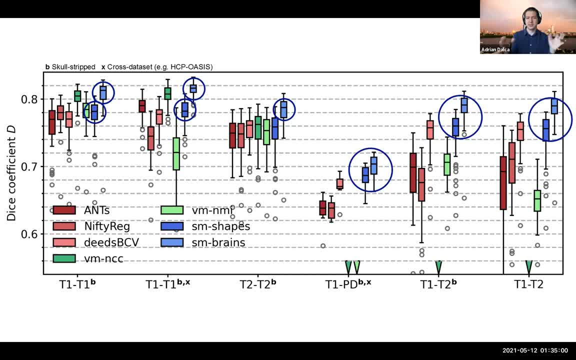 really well on training, but it starts suffering on real data because it's as you say, it's only a small section. yeah, bigger. you make these models, though they start being able to cover the whole space very well. what's really phenomenal in the field of machine learning more generally is what: 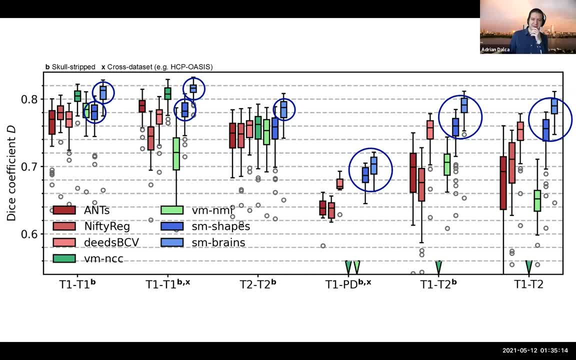 are you just like you know, like you keep trying and you'rebuch. the second part is like you search for models, but you have to think about machine learning, something, data. what a challenge is it's on the continent of itsitan Akuwa, for instance, and so for a lot. 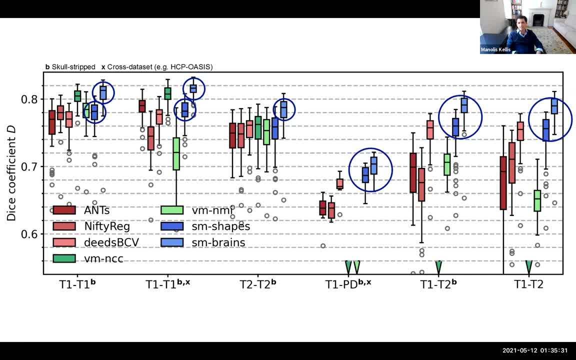 of engineers this day to experience it. it's so important. it's one line for them to feel like really human, yeah, and i feel that's so jó. so, yeah, yeah, we understand that probably anyone on this call is going to enjoy the details. thank you, um, let me show you, uh, maybe a little bit in practice, uh, what this means and why we're. 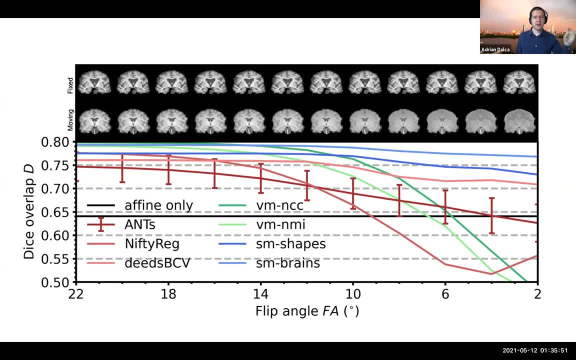 really, really excited. so here i'm, i'm simulating, sorry. the first is a scan of a brain and it's just the same scan. okay, in like 12 different scenarios or something. the second one is the same brain, but we acquired, um, this big sequence that you can simulate a bunch of different. 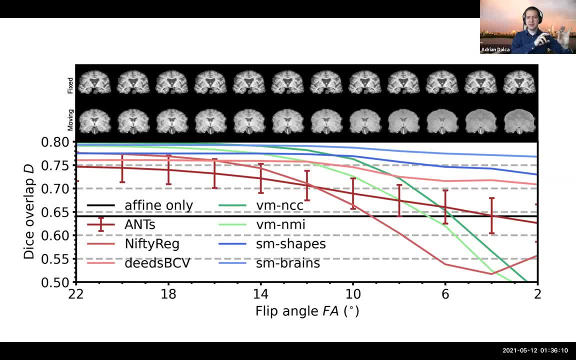 sequences. so same brain, exact same position, but different sequences, right smoothly varying, and it's the same stuff as before. red is classical models, um, green is is um, sorry, green is voxel morph and blue is our method, and you can see that as you start complicating the, the modality. 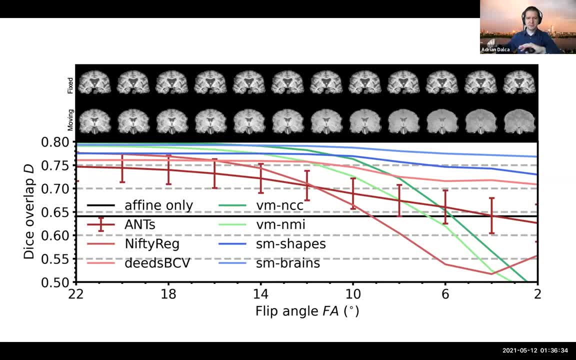 as it changes. classical models are suffering, voxel more, star suffering, but synthmorph it does something like that, but instead it changes the model of the brain and it gets familiarize with that and then you start individuals start suffering, but synthmorph it does something for a little bit, but you can see that it's quite robust. um, we started asking ourselves: why is this? 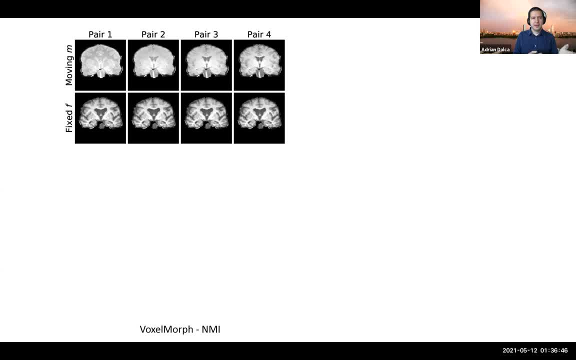 happening, like what is the network doing? so we started poking at the network again. these four different contrast pairs here, uh, voxel morph. if you look at the last, if you look at the features in the network towards the end of the network, you will see that the same feature, right, responds. 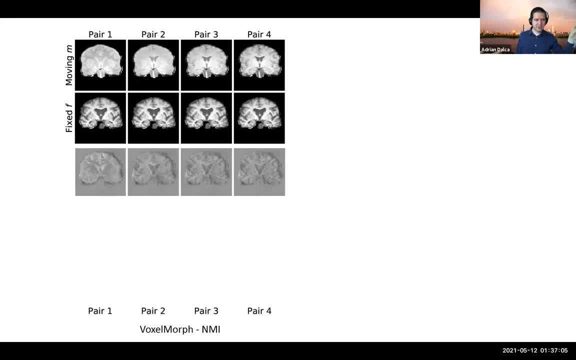 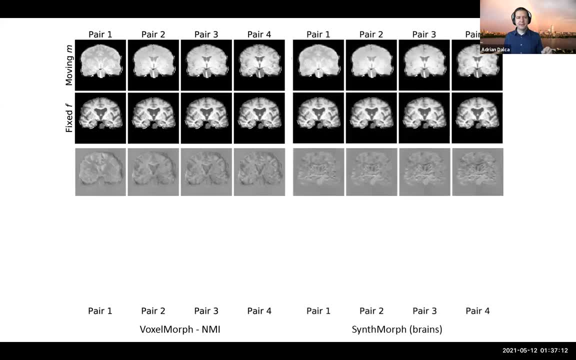 differently to these image pairs. so you know this is the same feature, same number, same channel, but you know it looks a little different because it is responding to what it sees. but synthmorph has learned to completely ignore contrast, like it's somehow extracting only the anatomy that matters and these features are after a while. they just don't respond to the. 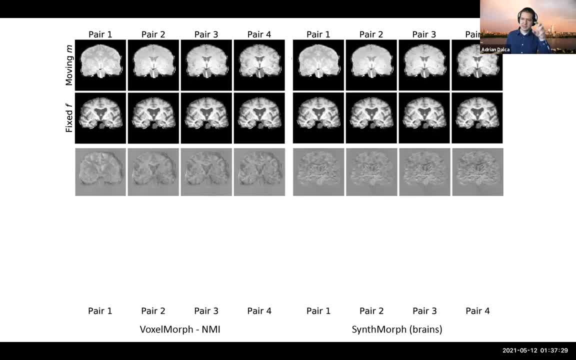 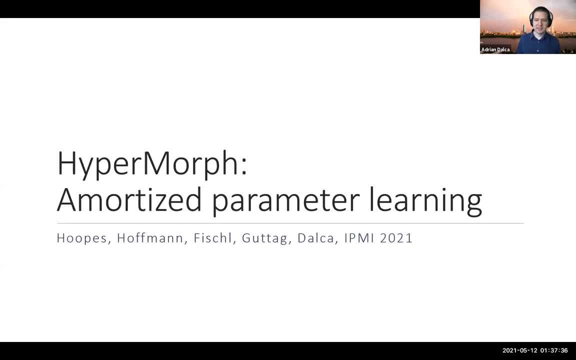 contrast variation anymore, and so somehow there's in the network it's learning to do that. there's a bunch of different features and we have quantifiable things. but, um, i do want to move on. i want to cover a couple more small projects, um, i guess. any questions on that quickly? no, all good. okay, all right. there's one thing, so so there. 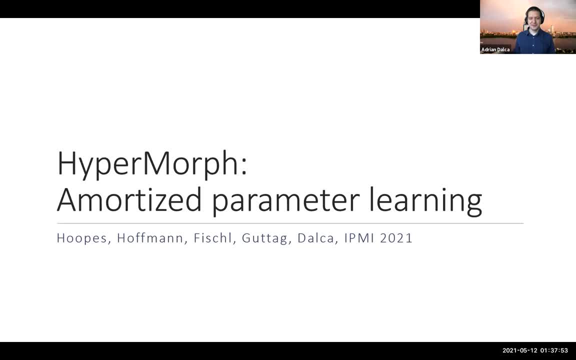 were these two really big things that have plagued, uh, voxel, morph and, well, every everybody. one was this like invariance, and i really do believe we've solved a good chunk of it. the other problem is- well, this is a general problem- we need hyperparameter tuning, and this is true of classical registration. 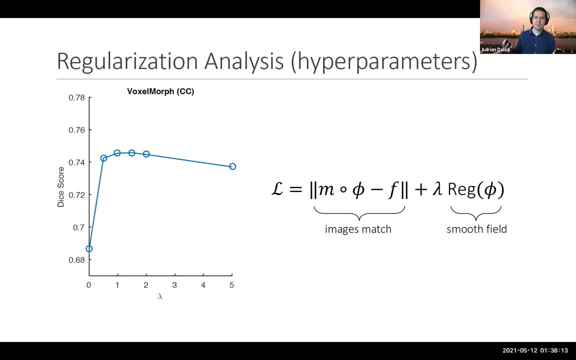 and it's true of neural networks as well. there's usually some hyperparameter that's really, really, really important, and for us, one of those hyperparameters, the most important one, is this, one that trades off between image matching and regularization, and it's always a problem, and 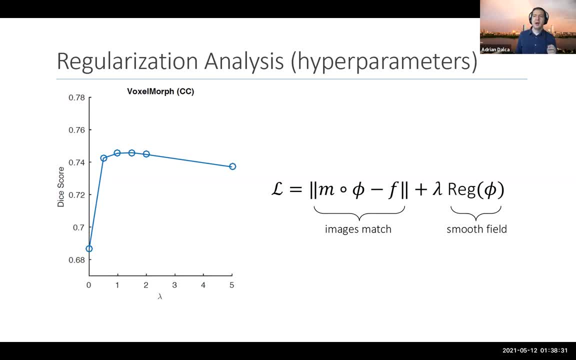 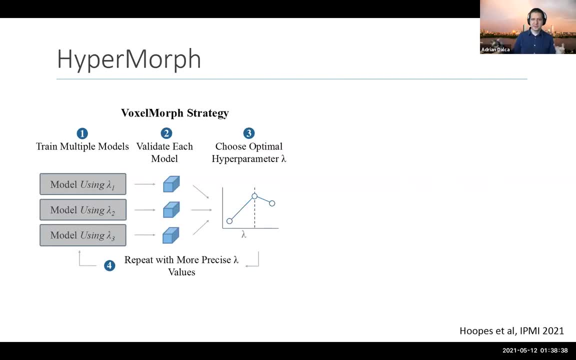 it's always someone, some something, someone tunes- most of the time, obviously, graduate students, and most of the time they do it by you- train three or five models with different values. at the start you have no idea and then you realize: oh, i got, you know, it's somewhere in this range, but i got to train some more models. 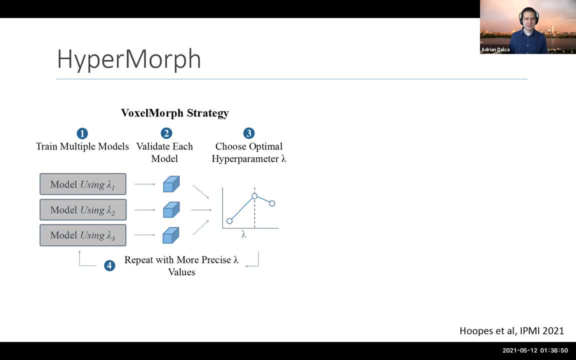 and then you train some more models and then your data changes a bit and this whole process starts all over again, and so it's an extremely painful process. and, um, so we, we thought: well, there's this one weird aspect here, which is these models are probably not that different. um, you know, there's some slight variability in them. probably they they're not. 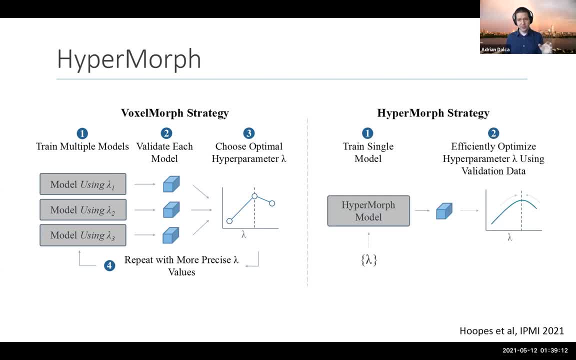 you know intuitively they're not that crazy. so we thought: well, could we train one really large model, kind of a super voxel morph type model that we called hypermorph, where it learns the effect of the hyperparameter on your registration. now, to be clear, it's not going to give you the best hyperparameter for your registration, because 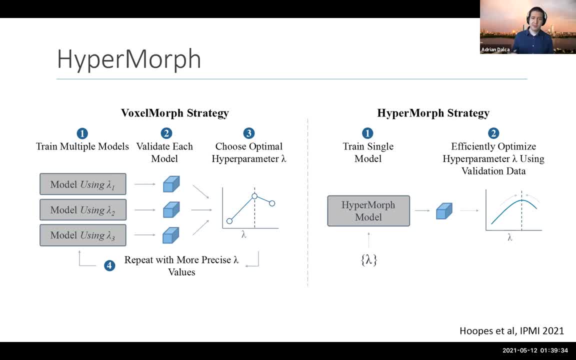 there is no such thing. it's not going to give you the best hyperparameter for your registration, because there is no such thing. um, it best hyperparameter varies with the task and the data and what the clinician wants and things like that, but this network will learn the effect of every hyperparameter value on that. 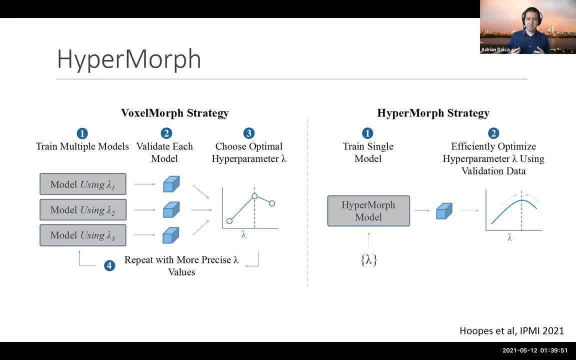 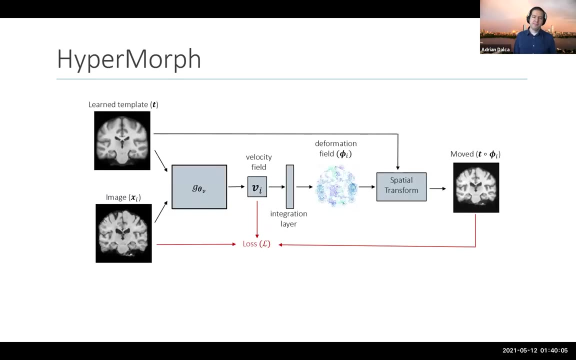 on the registration fields, the. the sort of potential of this is that, at the end of the day, you train one model and you just tune it afterwards, uh, without having to retrain, without waiting for optimization, without anything. um, so how do we do this? uh, this is one variant of voxel morph: the. 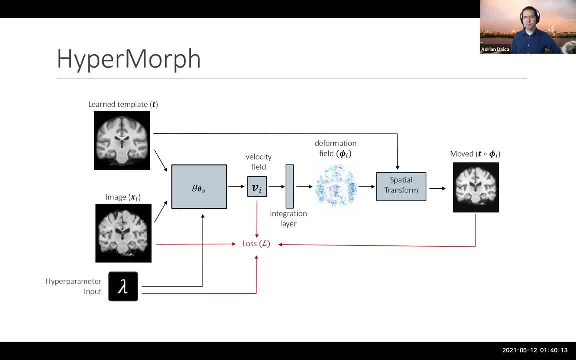 exact architecture doesn't matter. what matters is you take this hyperparameter value and you push, you put it into the network as an input- okay- and you train it by giving it a bunch of different values that it sees and you also apply those values in the loss. so when you say a value of zero, 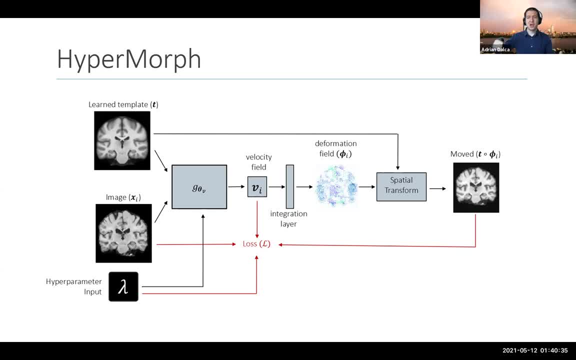 0.5,. the network sees this as input. but it also knows that, oh, I have to give you a moderately regularized deformation field. If the value is zero, the network says, oh, I know that I'm not going to be penalized on my regularization, so I'm going to give you as crazy of a deformation. 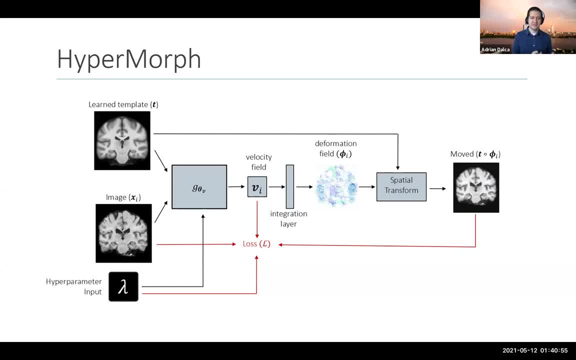 field as I can, and so on. So the network, by seeing the hyperparameter value, it learns the effect on the deformation field. Now, how do we actually do this? We've actually played with a few architectures, but interestingly, the thing that works phenomenally well is these things called. 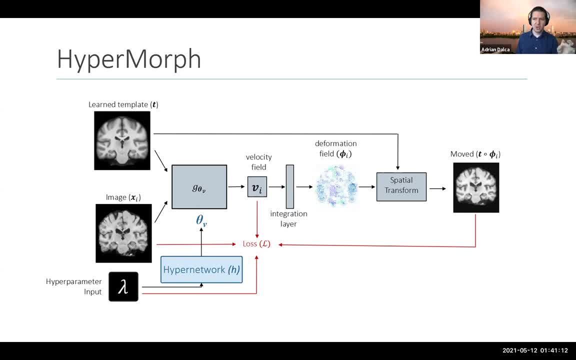 hypernetworks- Basically what these are. they're fairly small networks that take a value. in our case, they take a value and they output the weights of the voxel morph network. They output the weights of the unit, So they essentially change the function as a. 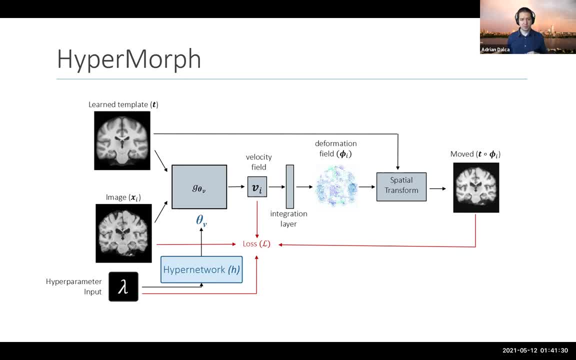 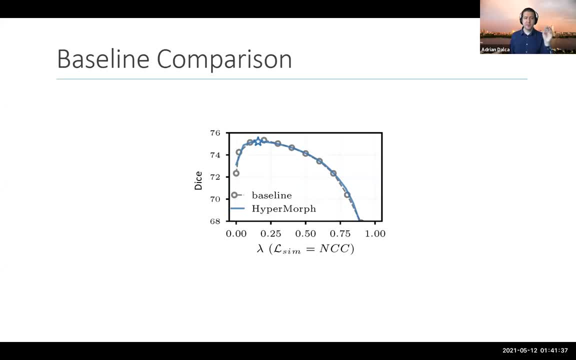 function As a function of the hyperparameter value, And this works, again, kind of surprisingly well. So, just as an example, what you can do is you can train a bunch of voxel morph models and this takes a lot of time right. So we trained- I forget, I think- 12 voxel morph models here. So you see, 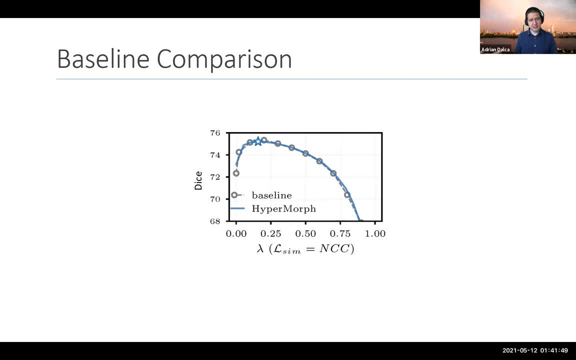 these gray circles, and that takes a lot of time and they're discrete, they're only at certain points. And then we trained a single hypervox model, which takes a little bit longer, but you just train one And you can see that now, at inference, you can just tune the hyperparameter. 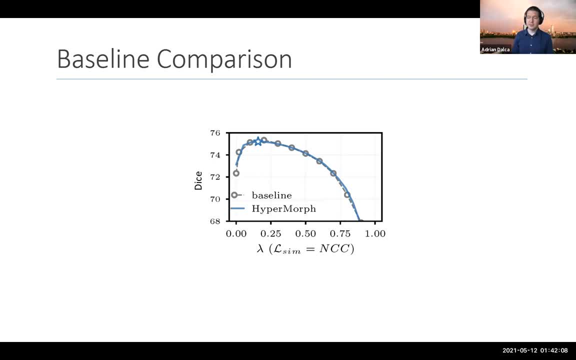 value and it matches up with those other models right. So this means that a single hypermorph model is able to capture this huge range? Adrian, this doesn't seem to be constrained to voxel morph. This is probably a much more general machine learning technique. Yeah, yeah, yeah, So I should. 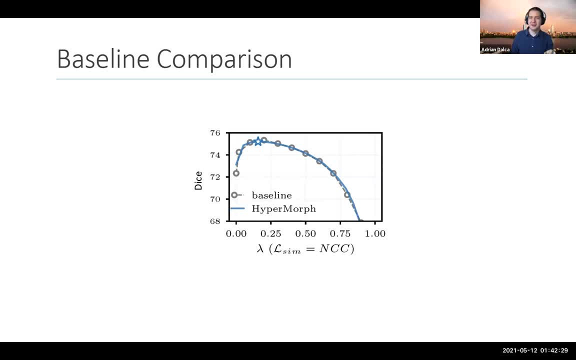 have said this at the beginning, I have definitely turned image registration as a sandbox of trying out new machine learning ideas. Yeah, And so very much agree. What I'm talking about today applies broadly and I can comment a lot on sort of how. Yeah, this is fascinating, Even just this setup, even just this setup of like. 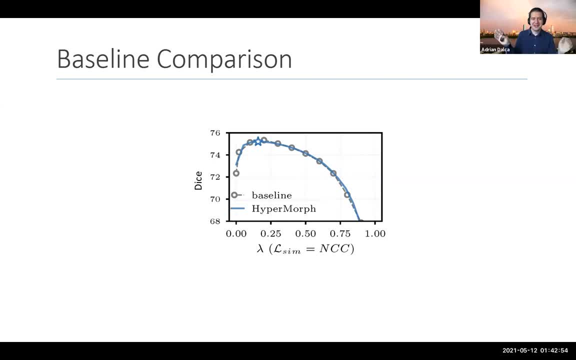 a term plus a regularization is incredibly popular in machine learning, let alone other hyperparameters and other settings. But just this setup right is so broad, And so why are we able to? So okay, this works across a bunch of different versions that you can. 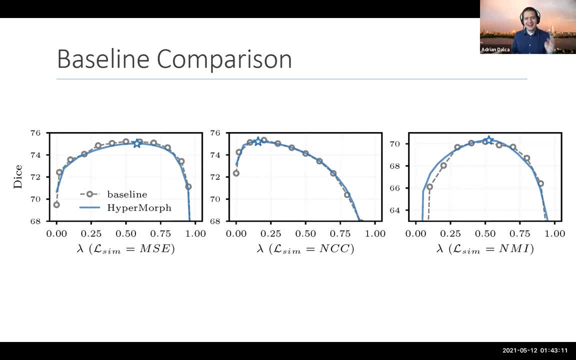 do. but why does this actually work so well? And it doesn't take 10 times the time. It takes about 1.5 times the time of a single model. So you weigh 150% as opposed to 1,200.. Why are you able to? 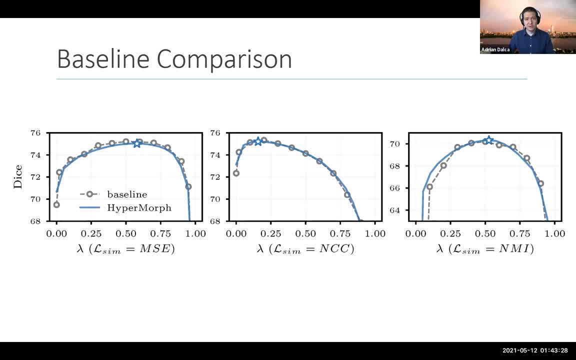 Well, it turns out that when you're trained, Where you're trained, And you learn 2,, 3,, 4, 5 different models with different hyperparameter values, the models learn the same thing over and over again, with slight modifications, And so the hyper network HyperMorph is able to capitalize on that shared. 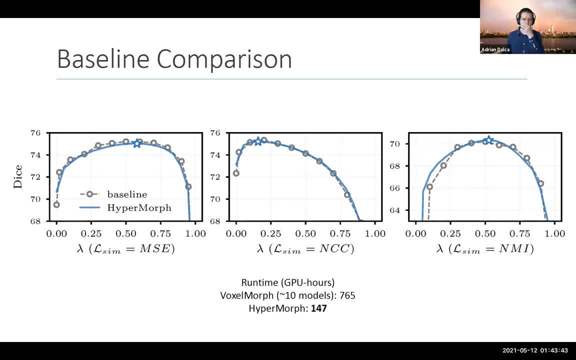 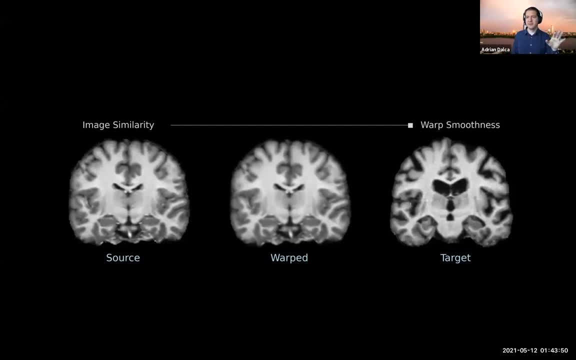 information and essentially just learn this delta. So in practice, in registration, this means a lot of things. The very idea I had originally was more about. and can they tune the hyperparameter value? And it turns out now you can. it's almost in real time. 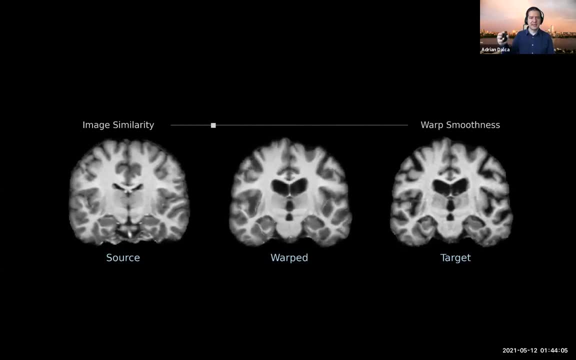 You can just sort of tune, have a knob that kind of affects how much a brain changes, right? This is just as an illustration. obviously you want more fine tune and you want all kinds of other things, but it's incredibly powerful interactively. 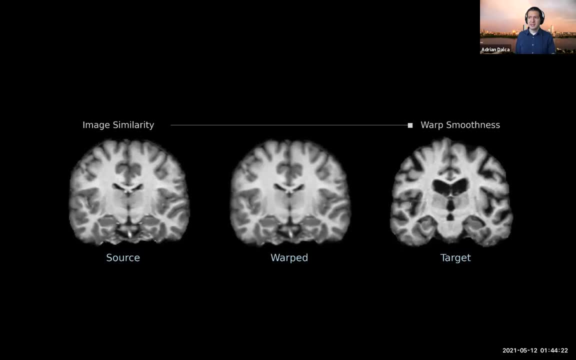 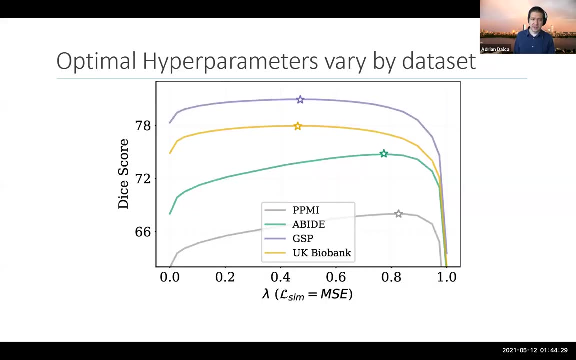 But what we've actually found, somewhat to our surprise, is that the optimal hyperparameter value varies dramatically with a lot of things, And the ability of having just one model that you tune afterwards means you can tune this manually or you can tune it based on some 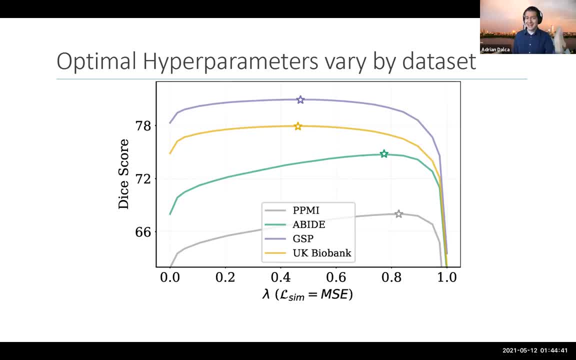 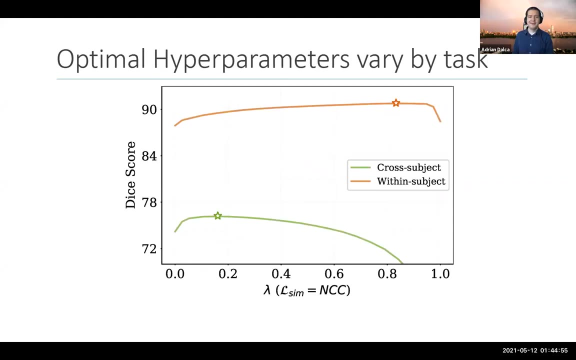 a tiny bit of validation data and all of a sudden, data set. So here there are four different data sets and the optimal hyperparameter value is different based on the quality of the data, the age of the patient, the number of patients in the data set, and so on. 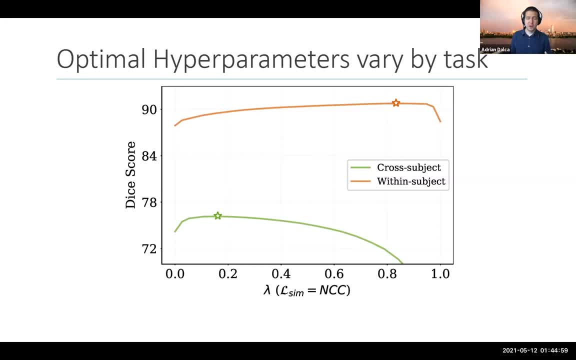 The type of registration task you do will give you different hyperparameter values. If you do between subjects or subject to a reference frame or things like that, you will have different hyperparameter values, optimal even by region. So if you've registered the same brains. 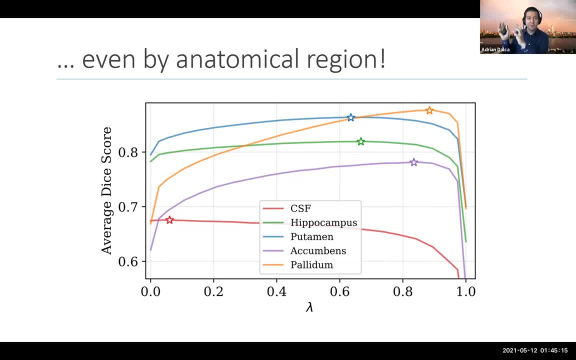 but you care more about the hippocampus versus you care more about the ventricles, you will want to choose different hyperparameter values, And so all of this. it shows a couple of things. First, training: a single model with a single hyperparameter value is not optimal. 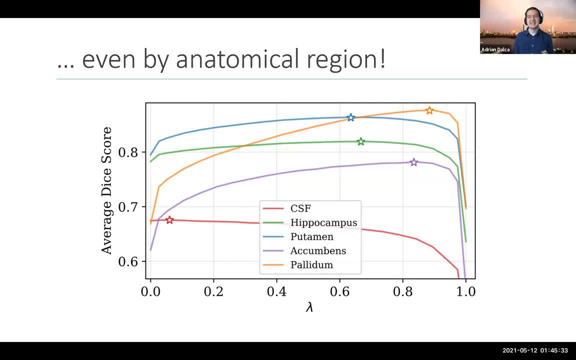 and you shouldn't do it, at least for registration, but probably for a lot of tasks. And second of all, training. just this one behemoth model- it's actually not that big, it's just it looks big- is a really powerful tool. 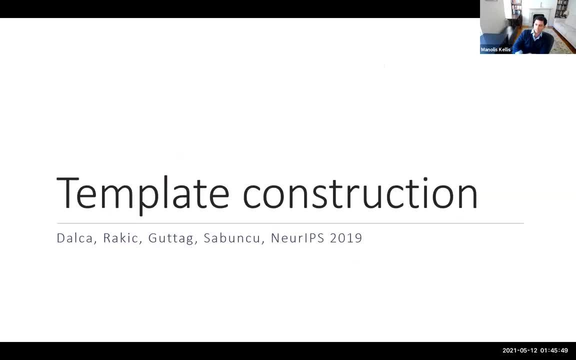 But I'm having a hard time reconciling how different the hyperparameters for different regions of the brain need to be with the fact that you could get this whole thing started with random images getting warped Right. So the advantage of that other, that's true, that's a good point. 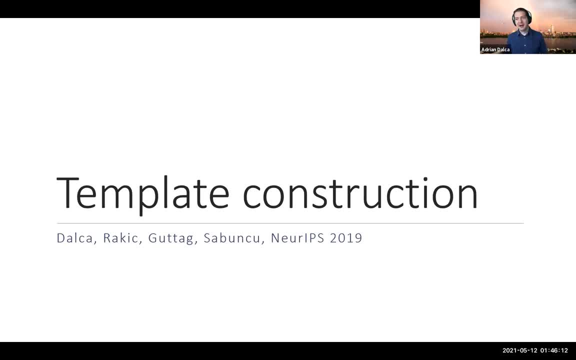 The advantage of that other model that has these random shapes is you're getting something else there that is a little hard to describe. You're actually really, really, really focusing on anatomy there Here, and so you're kind of learning to discern anatomy. 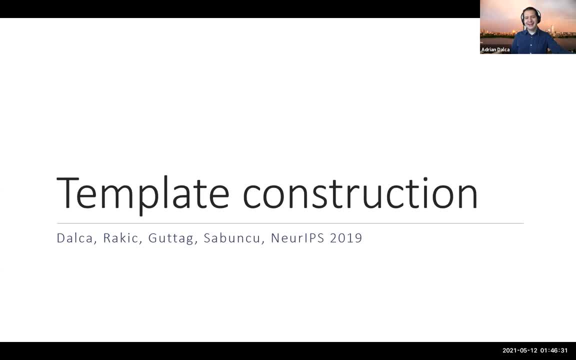 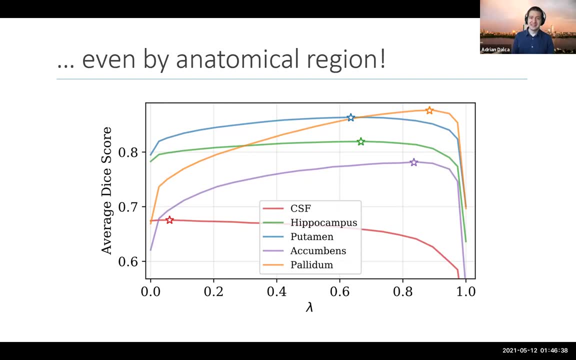 even in very subtle noise In here. what we trained in hypermorph, we trained just a normal one, trained on real data, And that's a little bit different because that one is not going to try to match up shapes at all right. 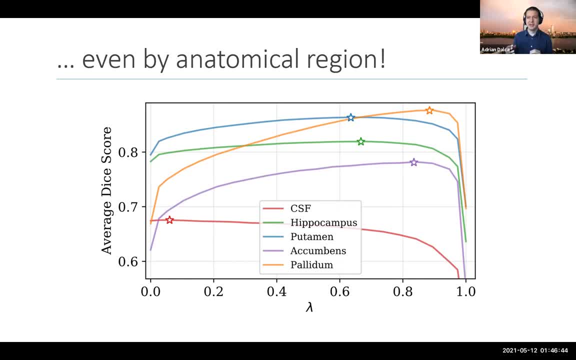 That's gonna be more susceptible to noise in different regions. That's gonna be. it's gonna match up shapes that have a lot of contrast, but it's not gonna match up shapes that have limited contrast. And so, to answer your question directly, 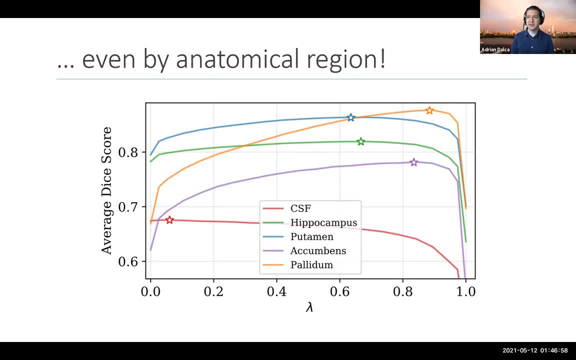 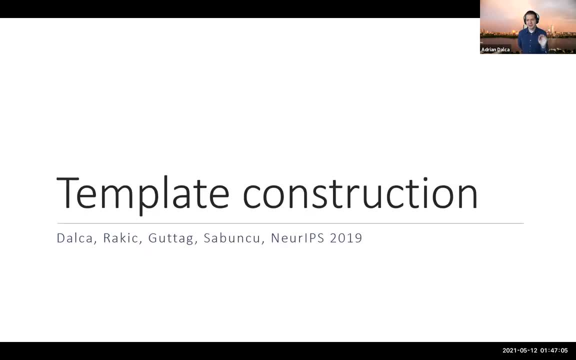 it might be a very different. this graph might look very differently in the synth morph case. Yeah, All right, the last thing I wanna cover. I know I'm sort of boring, I'm running a little late, but it's the last project. 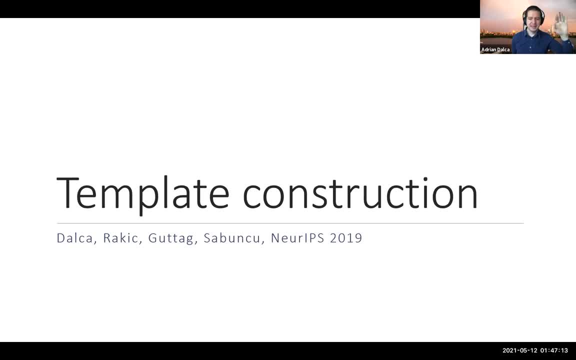 is because I really like it is this idea that well, a lot of times we align all our data to a common reference frame, but in a lot of projects we don't have a common reference frame. We could choose one example as a common reference frame. 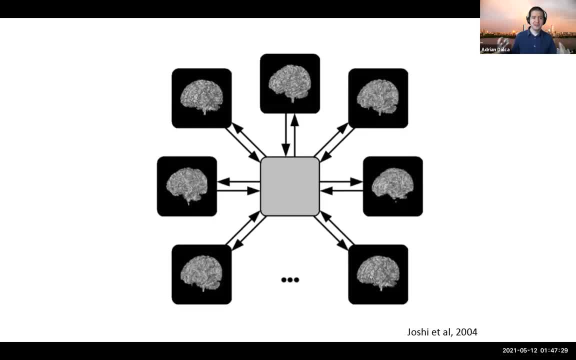 that has all kinds of problems. classically we build references, we build these kind of centroidal brains or other anatomy with this complicated process where you initialize it in some way- maybe you just throw an image or something and then you register everyone to that image. 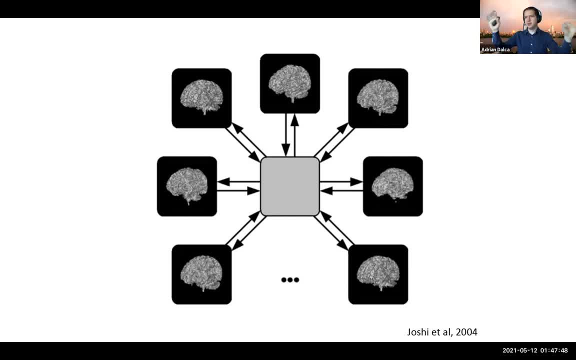 average those registrations and then you register every one again and you average and it takes forever. So, classically, there are algorithms. Honestly, it's not really done in practice because it takes a while, And so we started thinking about this. 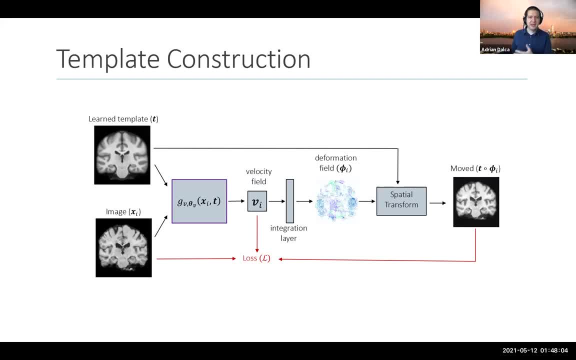 Everyone said, well, great, we can register, but we need a template. And so we thought: well, wait a minute. the Atlas is already learning something about the population. right, It gets to see all these data and somehow it's learning to approximate. 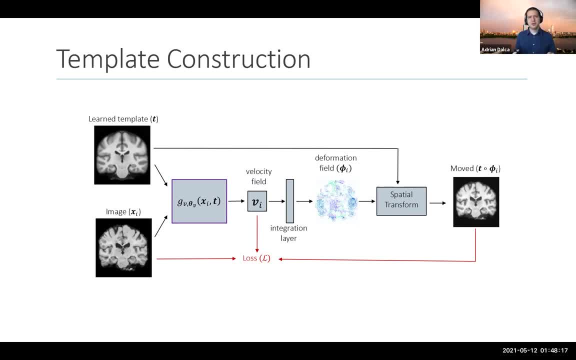 the result of registration. So instead of, let's say, we're learning a network that registers images to an Atlas, instead of giving the network the Atlas, what if we just tell it to estimate this Atlas at the same time as it's learning to register? 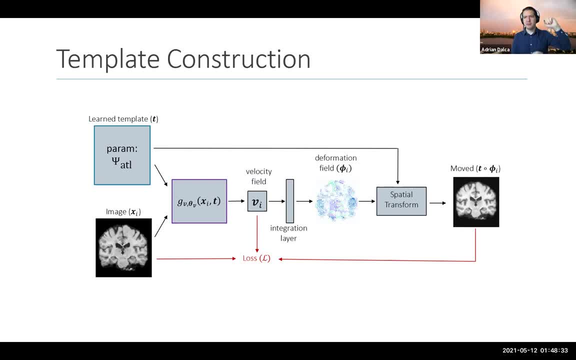 Basically, what we're saying is: oh, there's an image here, but it's not an input anymore. You have to estimate the intensities, And so we're just gonna feed it data. We're just gonna feed it an image at a time. 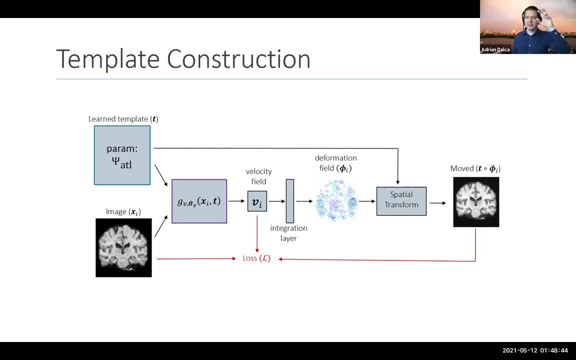 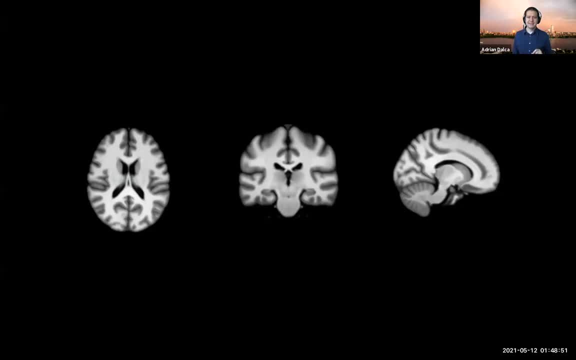 And over time the network learns what is the best Atlas, the best common reference frame for everybody that I can align images to. And this is what we got And it's really cool because this looks quite good for a template for our data. 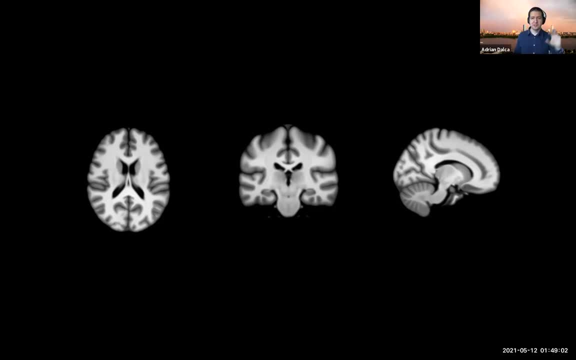 but also we never made any sophisticated changes. It was really just Voxelmorph with a couple of little changes on getting it to learn this Atlas. Importantly, it learns really nice anatomy, as I'm gonna show you in a second. But the real reason, I'm excited. 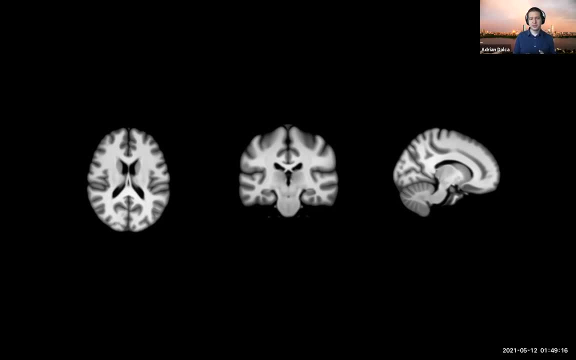 is because now we have this tool that is so flexible that we can solve a lot of problems that were fundamental, classical problems that were hard to solve. So, for example, let's say you have a really large population of subjects, This means usually a single template. 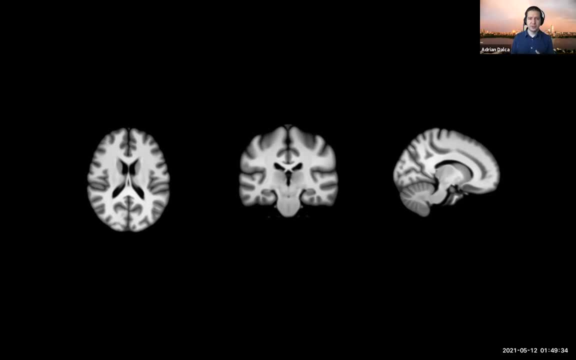 is not a good representation, So your analysis isn't going to be that good. So let's say you have 15 year olds and 90 year olds in your dataset. those brains will look different. So you would really love to sort of build. 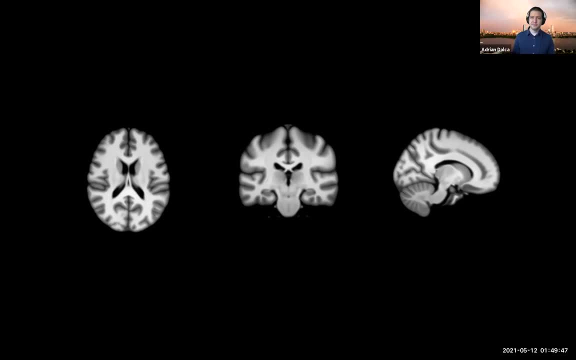 different templates, And so classically what people would do is they would sort of put people into bins and learn separate atlases. Of course that has all kinds of problems because it's very discreet, very approximate. So what we thought is: well, what if we learn? 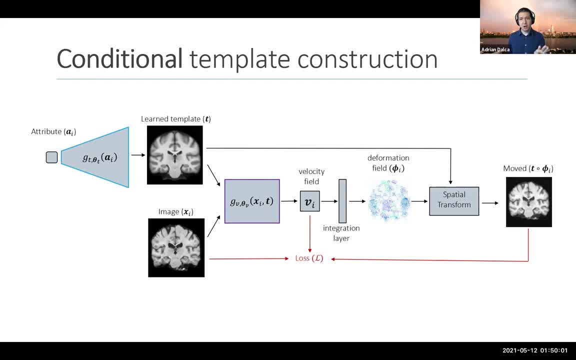 what we call conditional templates. So we're not gonna learn a template at all. We're gonna learn a function that gives me a template as a function of a property I care about. It could be age, it could be sex, could be some sort of genetic information. 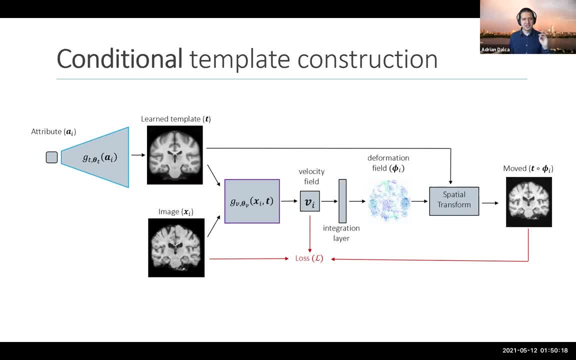 could be some sort of diagnosis, but we're gonna go with age as an example. So now I'm going to feed in. when I get brain of a patient, I'm gonna feed that to the network, but I'm gonna also feed in that patient's age. 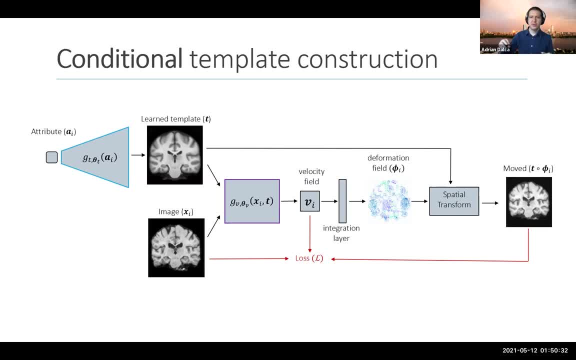 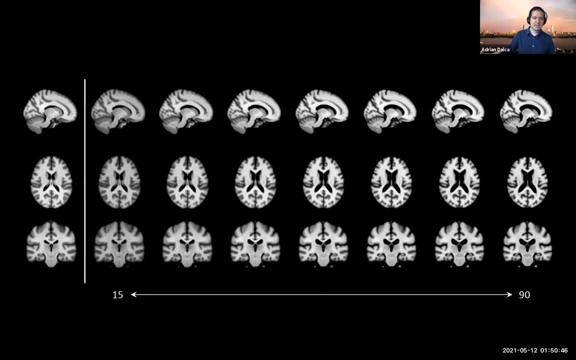 And over time the network learns this very smooth sort of age-dependent atlas as it sees the whole population And it looks something like this: Now, here I'm just showing you seven instances, right, Seven different ages, but you can see that it's learning. 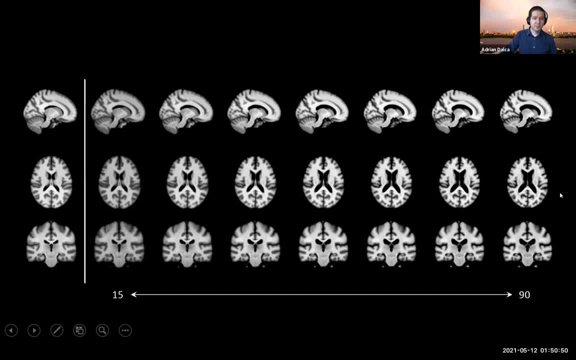 certain effects between this brain and this brain, right, So they're very. for example, these ventricles are much smaller here for people who are in their teens. or these ventricles are much larger here, In fact. I can show this in video form, which I like. 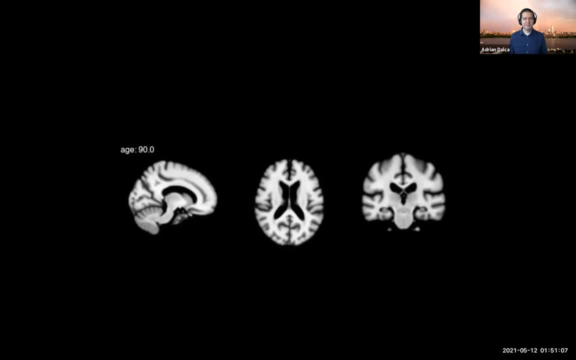 It's a very depressing video if you sort of know neuroanatomy. Basically it's showing that the brain shrinks with time. These ventricles in the middle, which are basically just filled with fluid, grow, and the rest of the brain- here it is- again- grow. 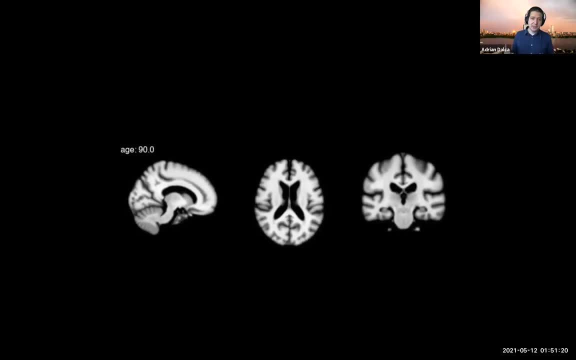 Here it is again: the rest of the brain shrinks And the really cool thing is we learned this from data alone. We never modeled any anatomy. We never explicitly created some sort of constraint. Of course we can add those for modeling purposes. 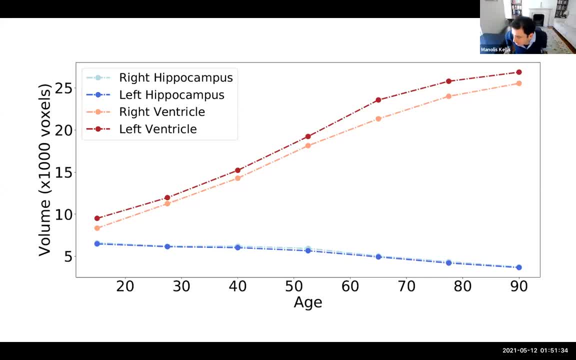 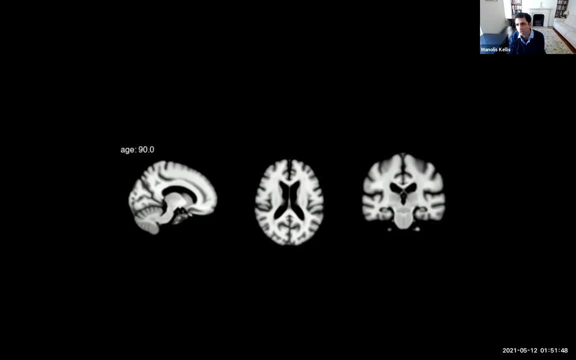 but we can then look. Adrian, a little bit on the variational to encoders that we've seen in the class earlier. Curious if you don't explicitly give age but you just tell it. basically, learn a family of models across different parameterizations. 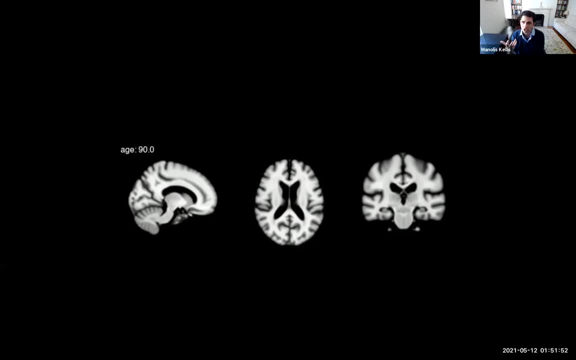 whether the system would automatically learn the concept of age as a parameter of variation in a different fashion For sure. So we tried this and it so it will learn the highest variability, kind of hidden covariates, And then it turns out those highest variability covariates. 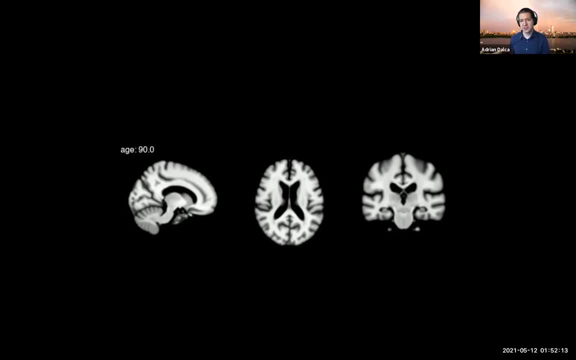 correlate very much with age and they correlate very much with some very bad neurodevelopmental problems like Alzheimer's right. So so we, so we ran that, and I mean we, you know, I don't know if what they're learning is actually age. 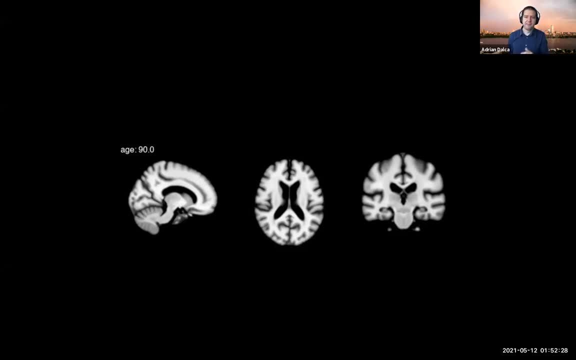 or just something that's deeper than that, but that correlates with age, right, But, but, but, yeah, definitely. So exactly what you're saying is the sort of stuff I'm excited about, because now we can actually try these sort of things, right? 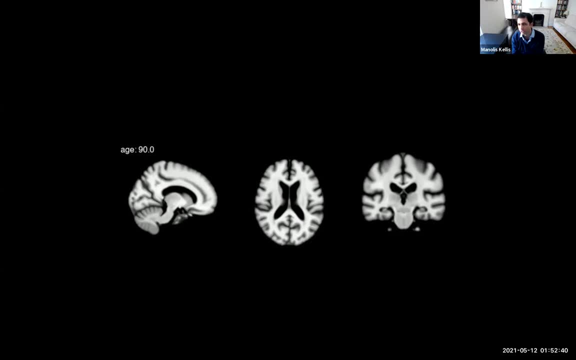 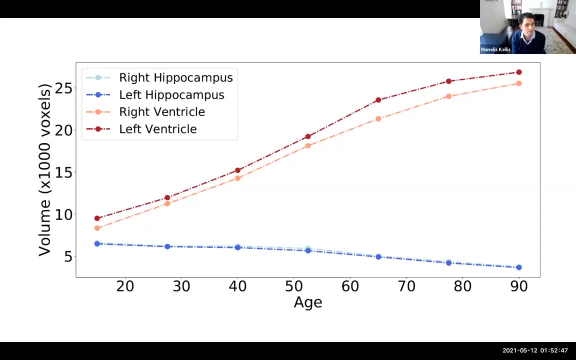 Yeah, And learn about parameters we didn't know about before, And that's what's very cool. basically, Exactly, Yeah, I love it, Yeah, Yeah. Yeah, The genetics part is actually one of the things we're actively doing too. 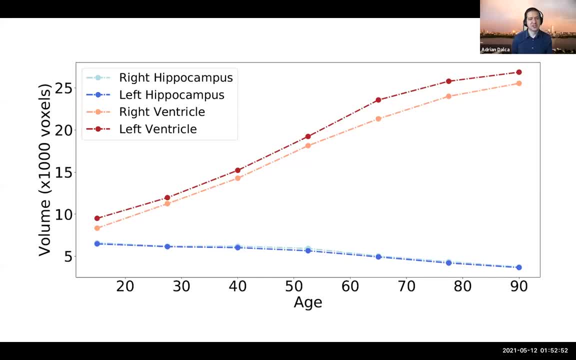 So, which again like, offers more interesting directions, And so you can actually measure these changes and you can actually verify them against the sort of stuff we knew. hippocampus shrinks, with age, ventricles shrink. We can also run these for, for, for, for populations. 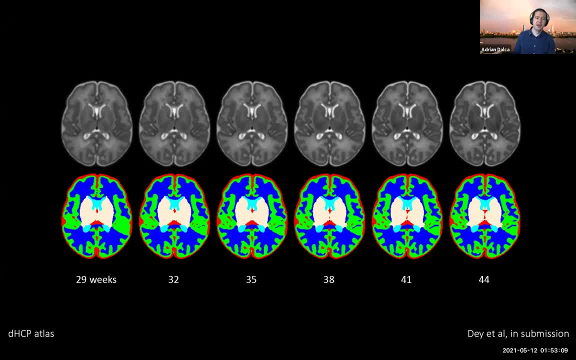 We don't have atlases for, or very good atlases for nowadays. So DHCP is this large, you know, effort for developmental brains And those are challenging. They brain, these are, these are very young subjects, right, 29 weeks. 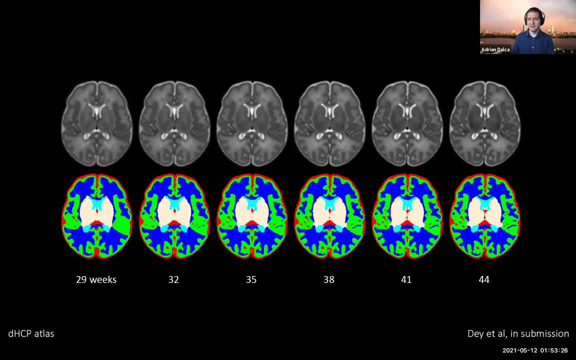 We even have some that are in the days, you know, kind of five days after birth, and you know, the brain changes like crazy. then like there's falls, the shape, the intensity is a change, and so on, And we can build those atlases now. 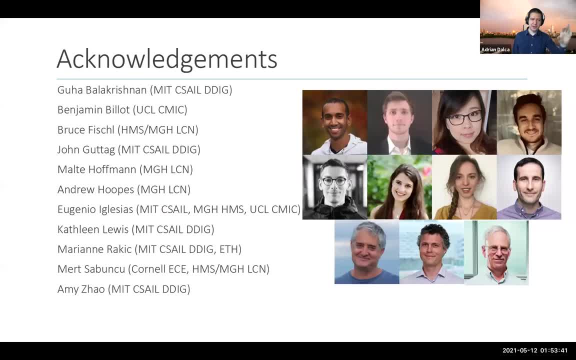 which I'm really excited about. So before I kind of close with the summary, I just want to acknowledge that you know there's a lot of projects, A lot of really great students and collaborators. So I again I didn't talk about this- 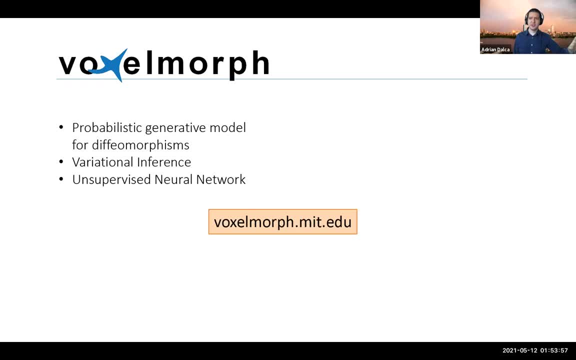 but underneath all this there's this probabilistic generative models that you can write, that drive this whole thing Connected to variational inference. you can get these unsupervised neural networks that have really been a new paradigm. They're really fast, definitely accurate. 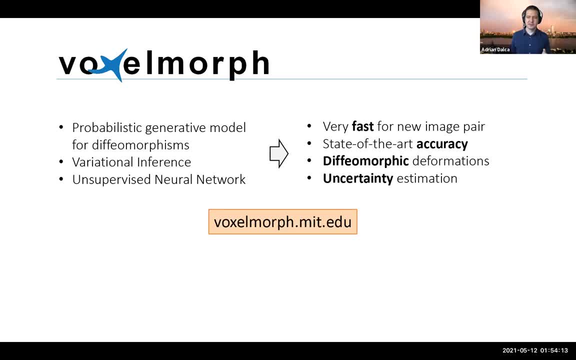 They have all kinds of properties that we wanted in the past: The few morphisms which I didn't get to talk about, but they're basically guaranteed. These smooth invertible fields. you can get uncertainty estimates, but really they have all these other cool properties. 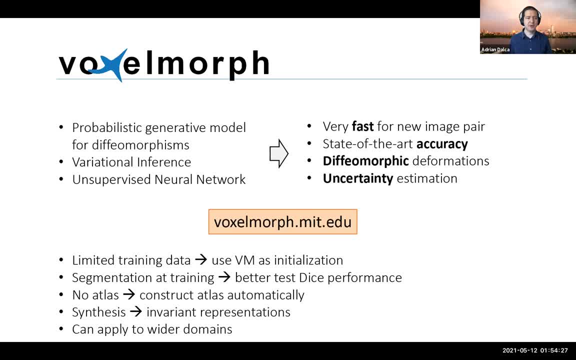 Answer to limited data. You can use segmentations if you want to help you along. If you don't have an atlas, you can build one. You can build in variances to contrasts And really this applies sort of broadly, as Manolis pointed out. 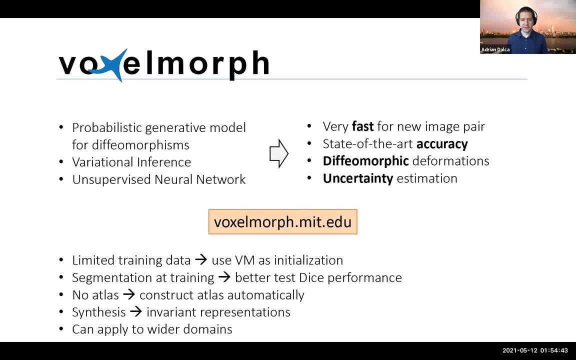 a lot of these concepts are really just a lot broader machine learning concepts, And that's it. Thank you Awesome. I want to ask everybody to join me in thanking Adrian for an awesome, awesome lecture. So thank you. Thank you very much. 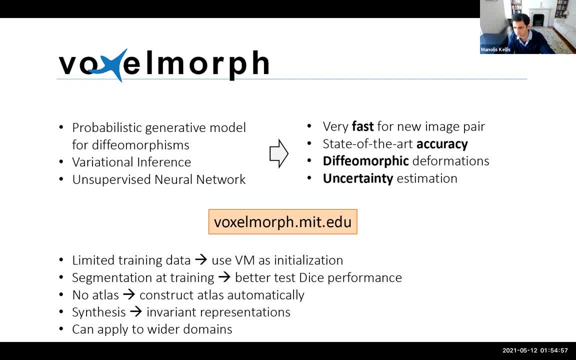 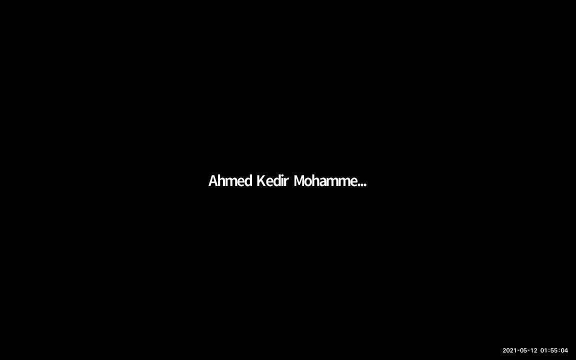 And we are also fortunate to have Ahmed Khedir-Mohammed, who is joining us as well, to give us another guest lecture. So let me stop the show. Okay, I got it. So, Ahmed, Yes, Can you start sharing your screen? 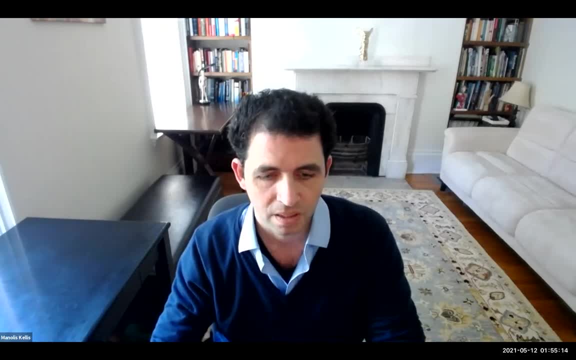 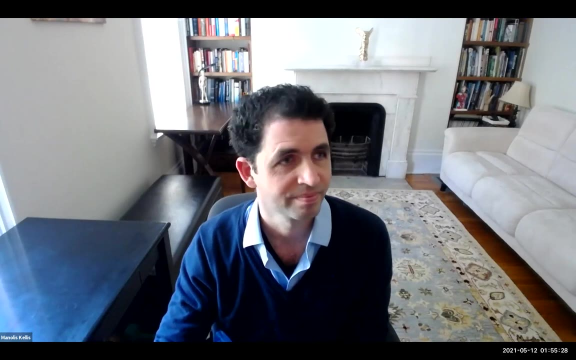 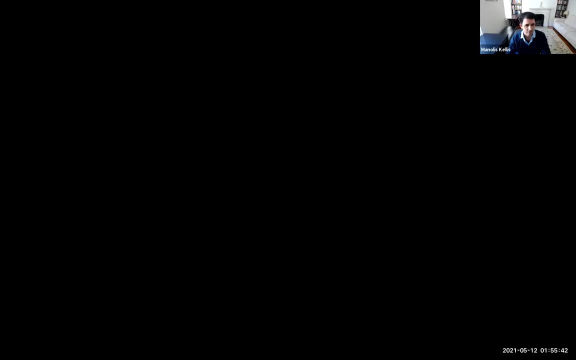 Yeah, Okay, Give me a sec, And then everyone, you can find the slides in Canvas and also at this Dropbox link. Thank you so much, Adrian. Really really appreciate it. Thank you, Everybody's able to get access to the slides. 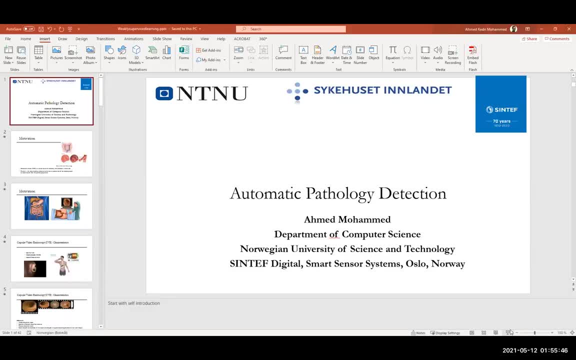 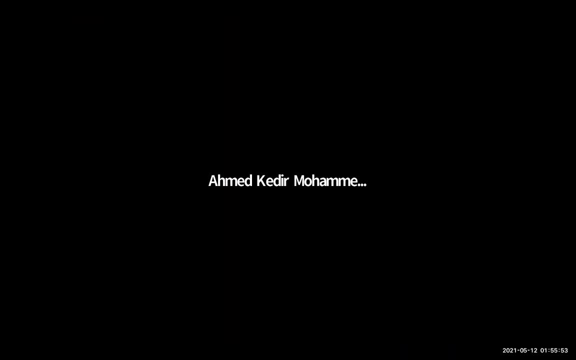 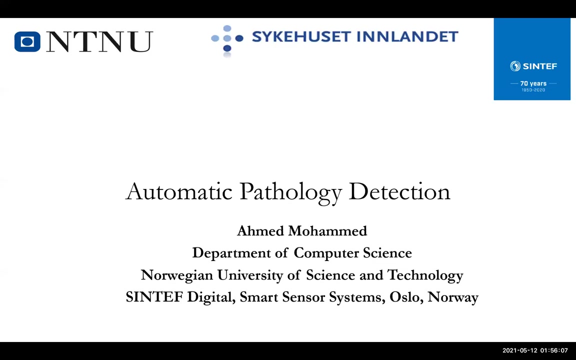 Great, And then we can see your screen. Beautiful, Awesome. Can you see my slide? Yeah, You might want to do a swap displays, Okay, And maybe let me stop showing them. Yeah, How about now We can see the whole thing. 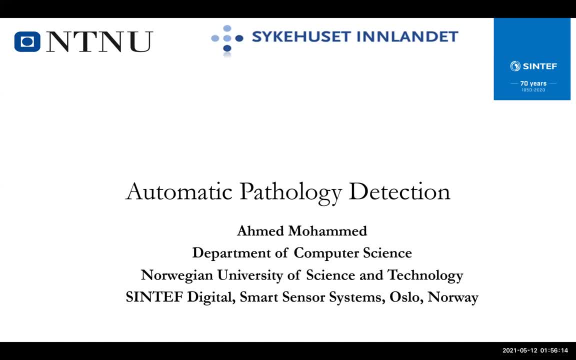 Yeah, Perfect If it's okay. but No, no, Turn it on. Okay, Perfect. Yeah, Yeah, All right, Welcome, welcome. Thank you for inviting me. I was looking at the lectures and they are very interesting. 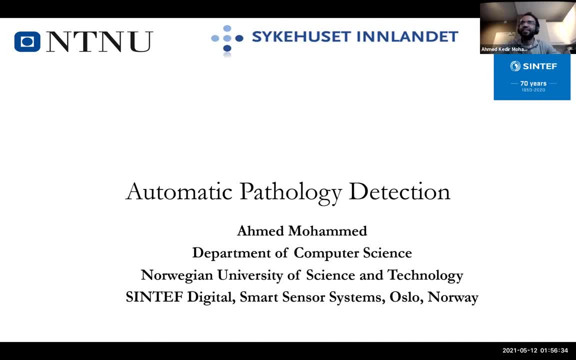 And thank you for making it available for everyone to see as well. They are very interesting. So my presentation is on automatic pathology detection, mostly for capsule video endoscopy. So this is a collaboration work with NTNU, Norwegian University of Science Technology. 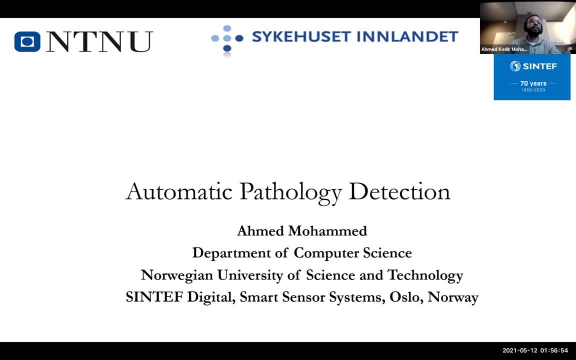 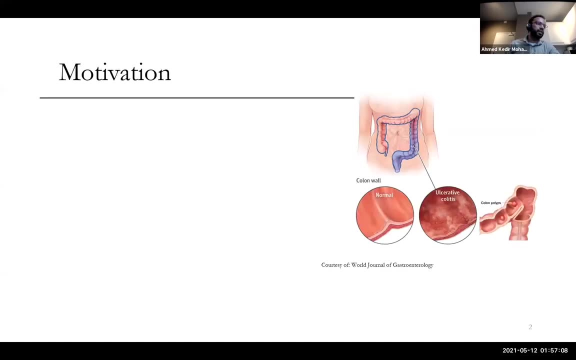 and a Jivik hospital here in Norway. So, from what I see, most of the modalities- the modalities you have been checking- are very different from what I'm presenting, So I will go through some of the modality that we are working on, which is capsule video endoscopy. 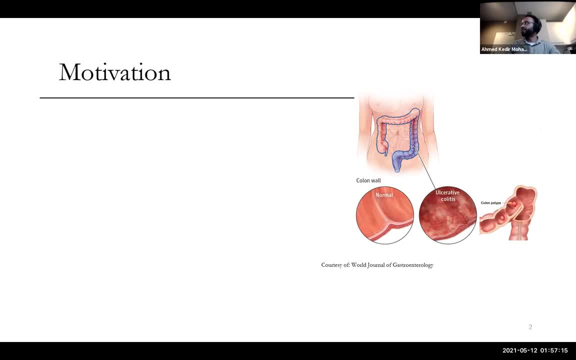 and colonoscopy. Okay, So I will go through the modalities, Which is capsule video, endoscopy and colonoscopy. If you guys know it already, then it will be a nice summary of what it is. So the motivation for our work is the colon, the human colon, which, for example, the colorectal cancer detection and something like that. 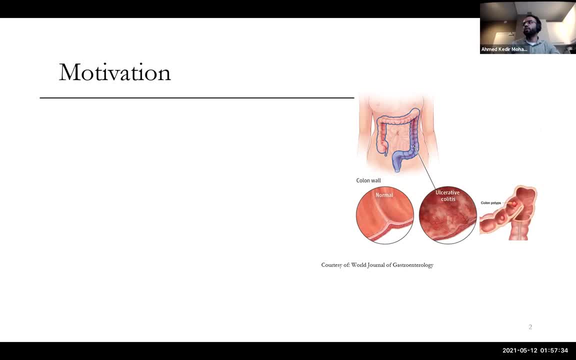 So if you have a normal colon, then the wall of the colon will be very smooth, as you see it here. So you have a smoother surface And when you have some disease, for example, like arthritis, colitis or Crohn's disease, then that will be eroded. 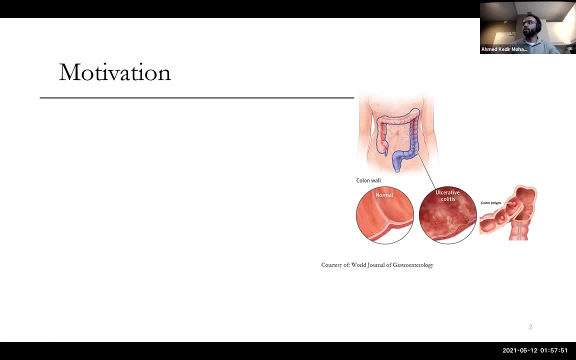 And you have a Crohn's disease, then you have bleeding or something similar. So the colorectal cancer is a major source of death from cancer And if you have arthritis, colitis or Crohn's disease, then it could also happen. 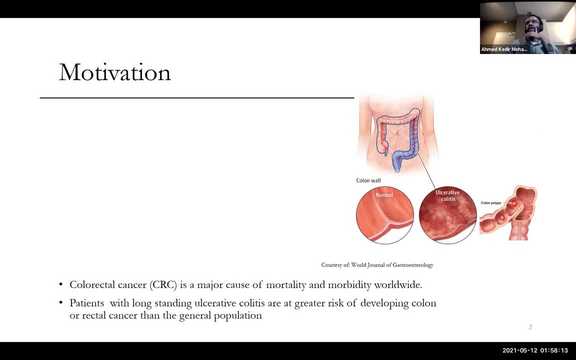 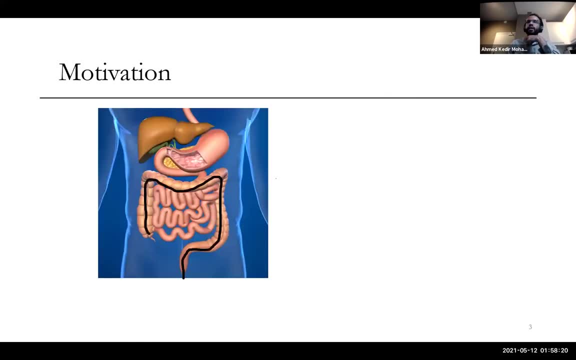 So you have a higher risk of developing a colon tumour or rectal tumour, So it is very important to detect it early on. So the human colon is like around 150 centimetres long and compared to the small intestine, which is long and narrower. 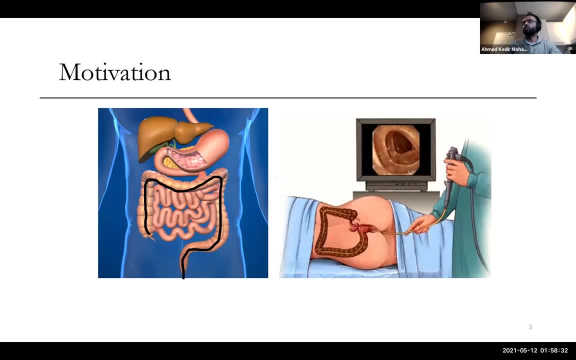 So the typical way of investigating it is through colonoscopy, where the doctor enters the colonoscope and tries to see the walls of the colon for any kind of abnormalities. But, as you can see, this is actually recommended by doctors, mostly after the age of 50, depending on the country. 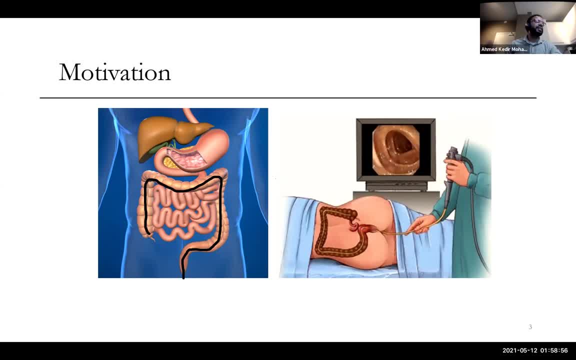 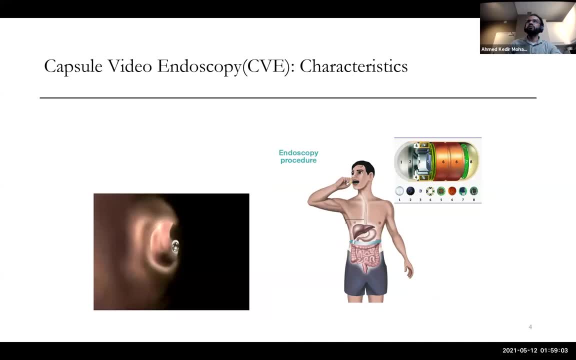 And there is a lot of it's not accepted that much by the patients. So there are alternative ways of imaging this and that is where it comes to capsule video endoscopy. So a capsule is a small steel-sized camera which is 31 by 11 millimetres long size, and you have a DOOM sensor and you have a battery and you have an antenna transmitter. 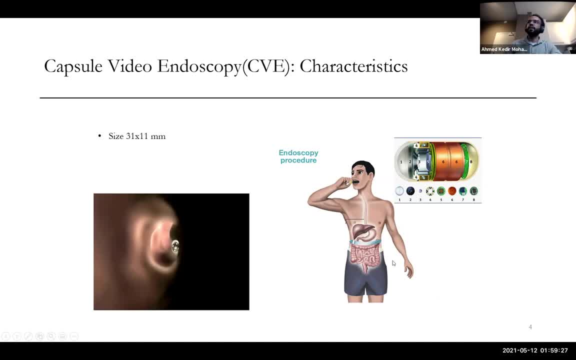 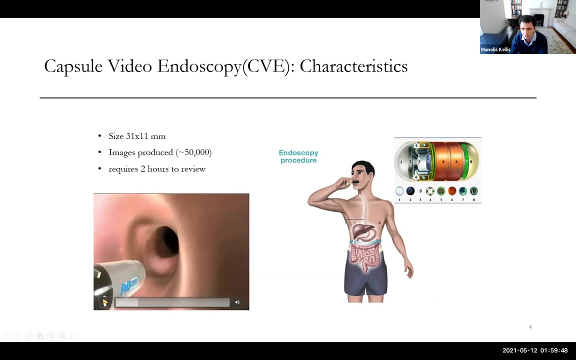 and the patient will wear a vest and the image will be transmitted through that vest basically. So it produces a lot, of, a large amount of frames- around 50,000 frames- And- and it takes almost Sorry to be so blunt here, but one of the advantages of colonoscopy from the other direction is that you actually empty the colon. 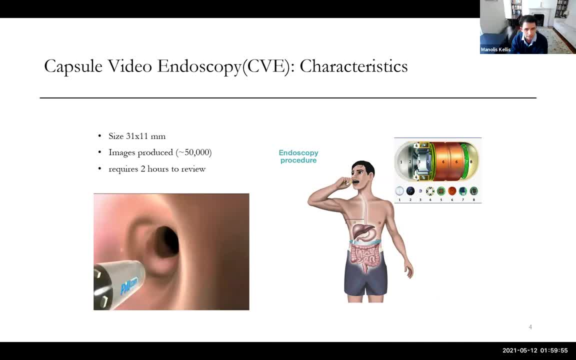 Yeah, So that you can actually see polyps, et cetera. If this is done without actually emptying it out, is it that it actually misses a lot of the features that would otherwise be visible? Yeah, So that is colon cleaning procedure. 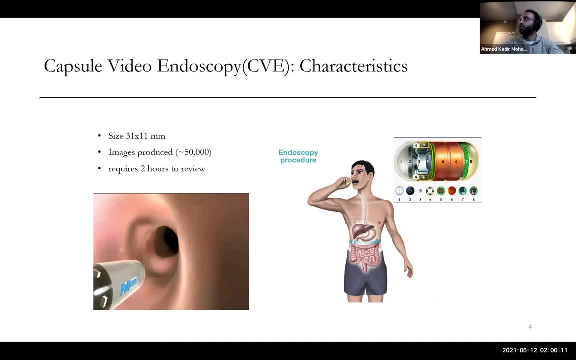 That is done for both colonoscopies And capsule video endoscopy. Got it, Got it. So it's just that you don't have to do the other part. So the other question is: if something is swallowed in an empty stomach, does it sort of change the way that it travels? 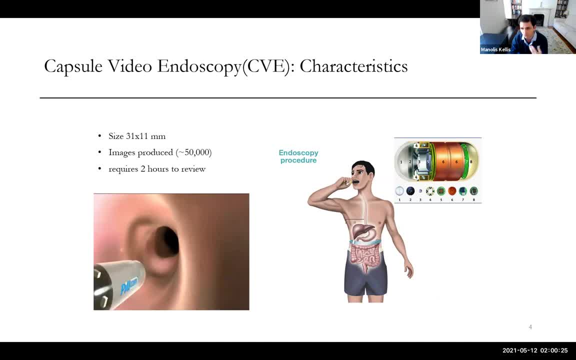 Does it need to wait for food to actually come, And when the food comes, will it obstruct its view? Yeah, yeah, yeah, That's true. So you need to be. for example, if you are doing colonoscopy, I hope none of you does- you take some regimen? 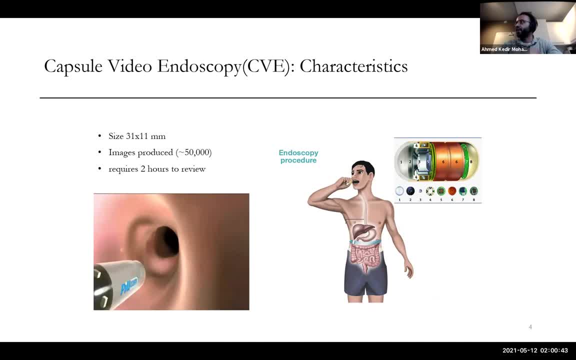 Which cleans the colon completely, and then you have empty colon. You do the same thing, but you take extra procedure for this, for capsule video endoscopy, because you need a full, empty stomach. Plus, as you can see, it is going with the food. 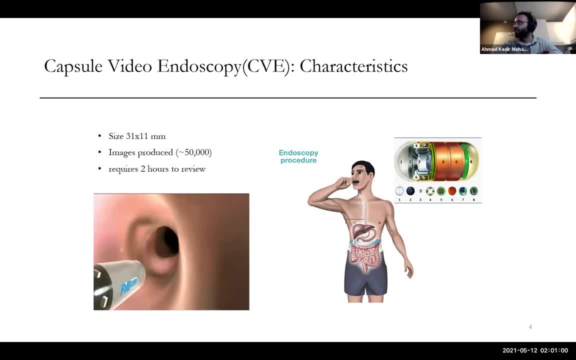 So you are not flexible in imaging where you want the image. So, for example, and especially in the colon, the colon is a bit wider- That's why I bring it early on- compared to small bowel. Yeah, So since it can go, the polyps could appear in the folds of the colon. then you could easily miss it. 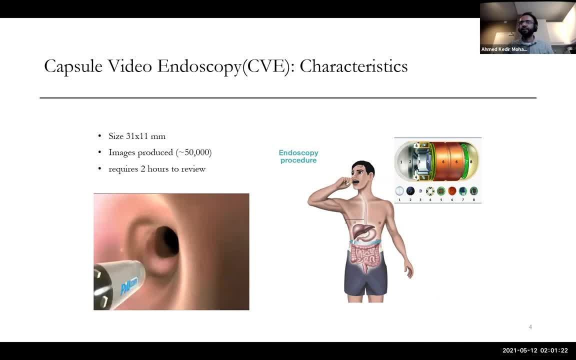 So that's a huge problem with this approach. Another question that I have is a lot of the food after it exits the stomach. it's already much smaller than the size of the capsule. Yeah, Are there issues that are just simply geometric in getting through the small intestine? 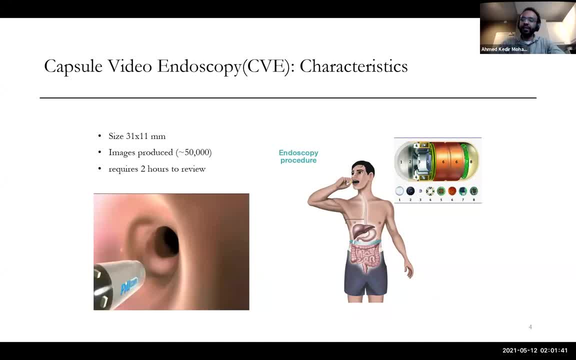 So that's also very important. So that's actually a huge, not a huge problem, but there is a solution to it. So, for example, there are some diseases called diverticulitis- I will show you some- with the result- where you have holes, basically in your colon pads. 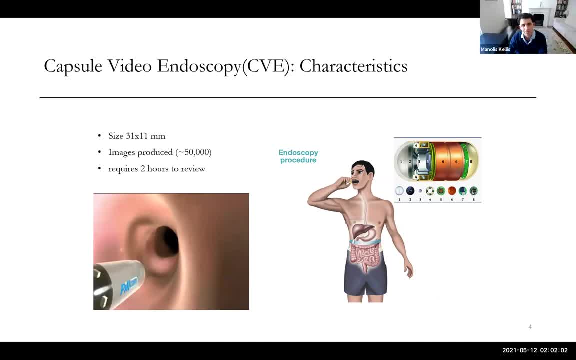 And then it could stack there- Wow. So the usual approach or the medical solution for this is usually doctors will give you one, Yeah, And then they will give you a dissolvable capsule early on- Wow. So that's like an extreme case where you have known such kind of problems. 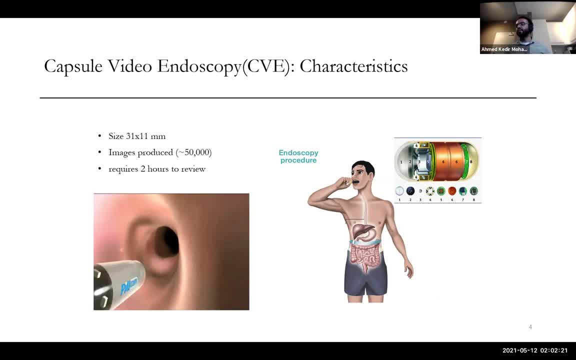 Yeah, But in any case, if the capsule is going to be stuck, it is almost you need to do surgery. Yeah, yeah, But even if it doesn't- for example, if the food starts stacking somewhere, a bacteria will be developed. 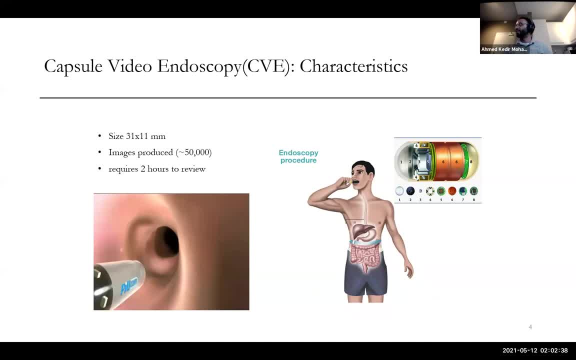 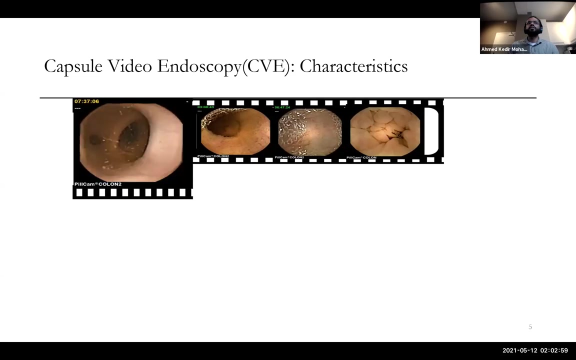 So you'll have surgery anyway, So it will not be harmful to do that surgery. Okay, thank you very much. Yeah, no worries. So this capsule just travels in the colon. So to show you some of the videos that come from the capsule is: if you look at this, this is from actual colon, capsule two: 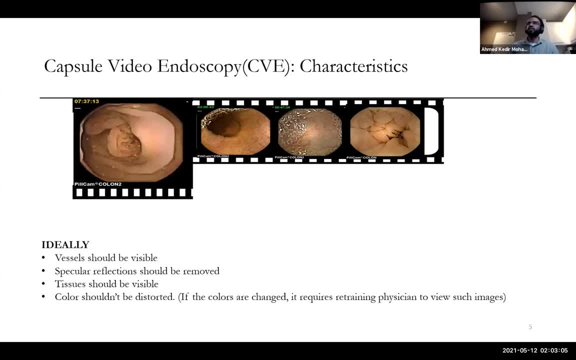 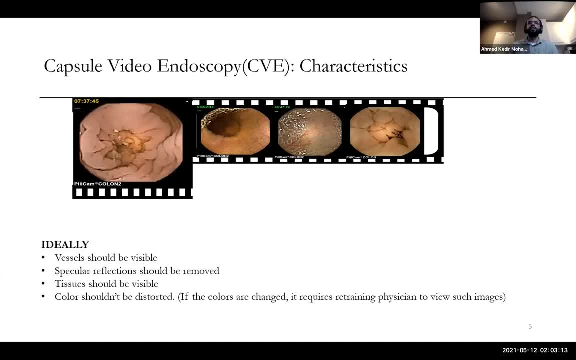 It's not as good as the HD. It's not as good as the HD And for the doctors, what they need is the vessels should need to be visible, because the vessels have a lot of information to give And you don't need a lot of specular reflection. 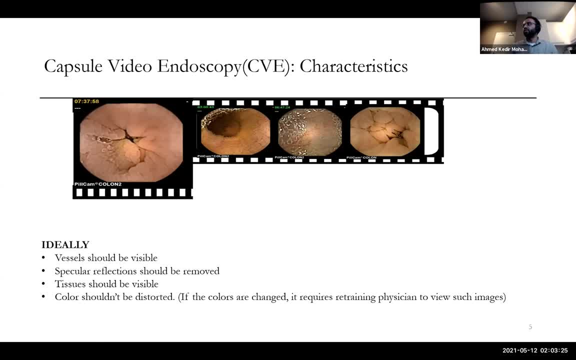 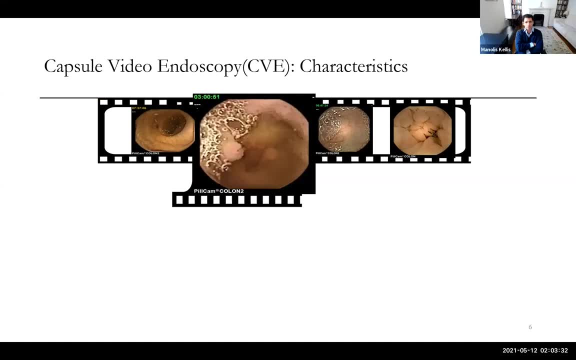 And you need. also, the color should not be distorted, Otherwise you need to retrain the doctors to do this again. I'm very surprised by how straight it goes. I would expect it to do a lot more tumbling, Yeah, Yeah. 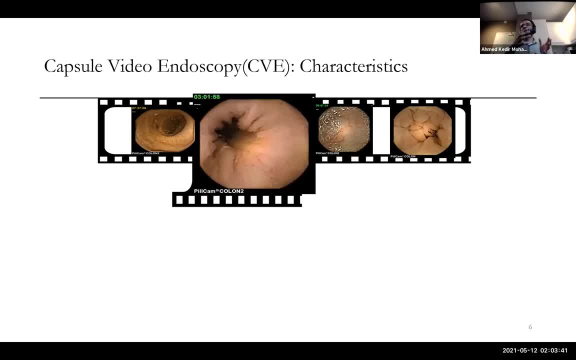 So it depends, Like, for example, it's not as good as the HD. Yeah, In this case it's going here and there, But it depends, for example, if it is ascending colon and descending colon, Like when it's descending colon it's going fast. 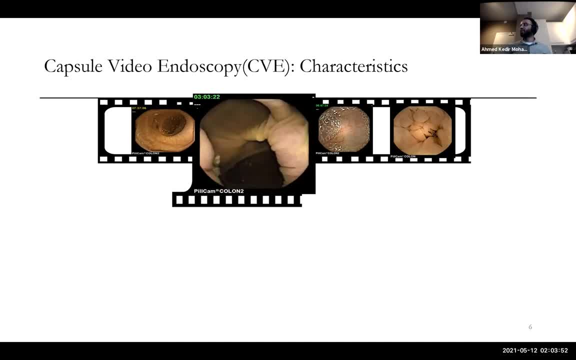 So when it's ascending colon it's going slow, So it depends where you are, And when it's traversing colon, it depends where you are. imaging: Wow, Thank you. Yeah, And like, regarding the video, if you look at it it doesn't have smooth transition. 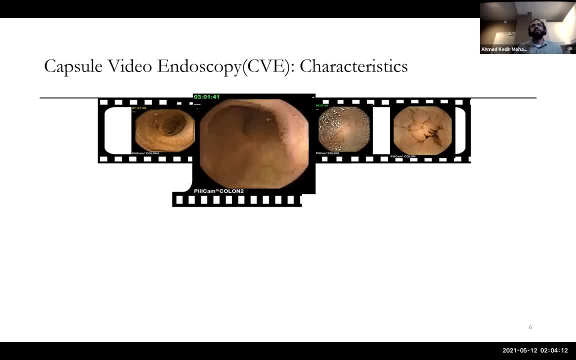 As you wish for with the smartphone cameras currently have. So you don't have this five effect, which appears that you have this living picture, moving picture, which makes it a video. You lack that And, of course, if you want to transmit a lot of frames, then you're going to kill the battery, which is around eight hours. 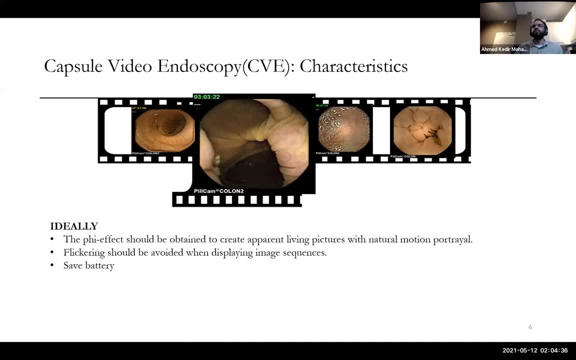 Or approximately, or sometimes it takes six hours, less than that, But then you're going to kill The battery, So you need to save the battery as well. You don't want to send a lot of frames And, But you can see the videos are not smooth. 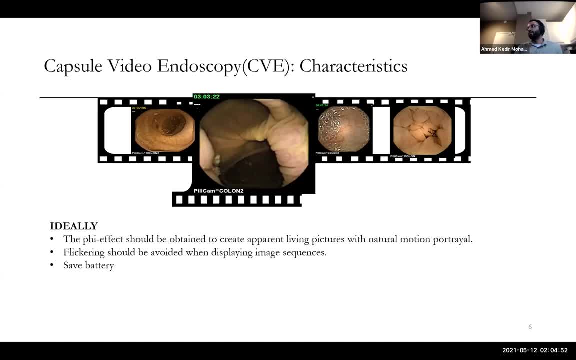 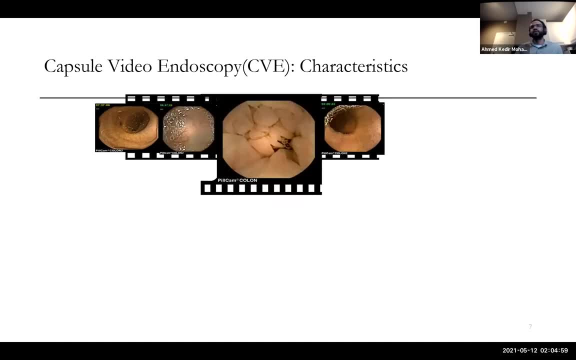 So I would like to give you on the next, on this next video I'm going to show you. I would like to give you try to see any kind of abnormality you can see. you can find on this one. So let me know if you find anything worth investigating. 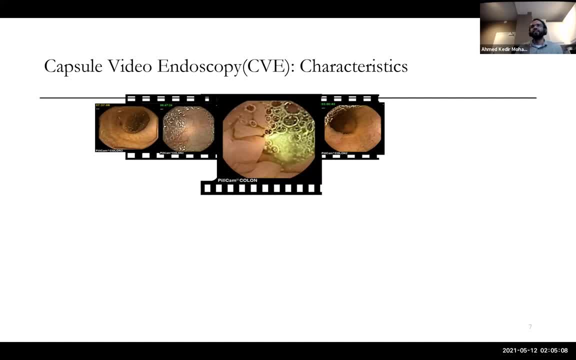 I know you are not medical doctors. I don't know if maybe there are some medical doctors in your class. So do you see anything unique in this video? Bubbles? There are both, And there is also one nine millimeter polyp that is hanging in the wall. 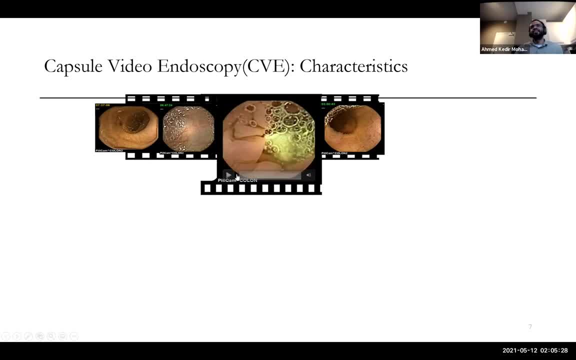 It just comes around here, That giant red thing Here. Yeah, exactly, That's a polyp. And the challenge is like you have this polyp coming, appearing and disappearing Very fast. So the doctor needs to be very attentive when when looking at these videos. 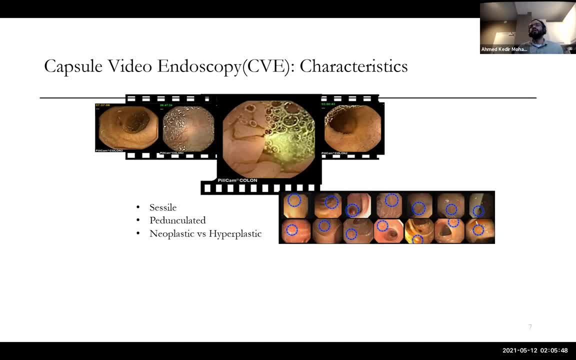 So the other problem you should have is like you have a lot of diseases, like even the polyps that are sys side, where you have broad base on the colon and you have peduncated the one that grow like mushrooms, and you have neoplastic, which are more dangerous one. 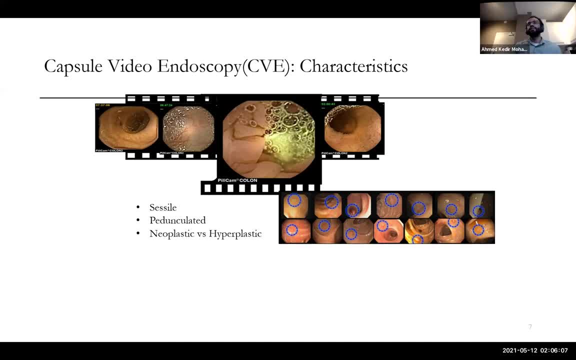 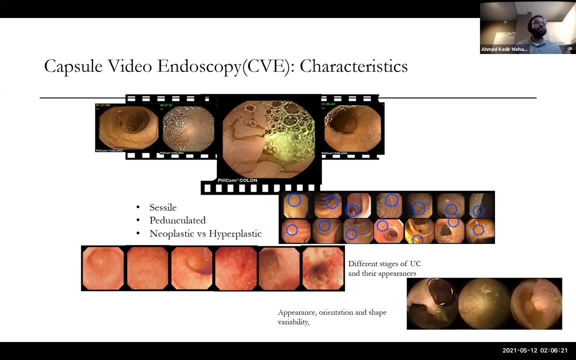 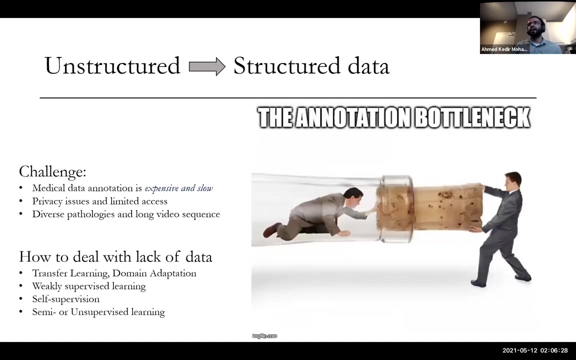 Like adenomas and hyper plastic, Which are are not daily, but so you have a lot of variations of this and you have different states of this disease. so if you want to do some sort of machine learning, then the problem, then you end up with having absence of lack of data, so you have alone this, a lot of video frames. 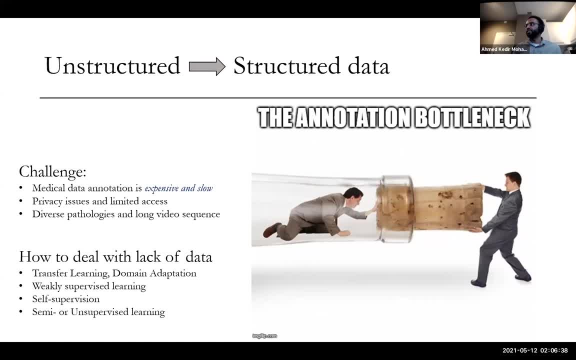 around 50 000 video per patient and if you want to do a medical, uh, in general medical determination is very expensive and slow and you need multiple doctors to approve a given, a given- i'm not seeing a comment, or if there's a question on on the chat, don't worry if there. 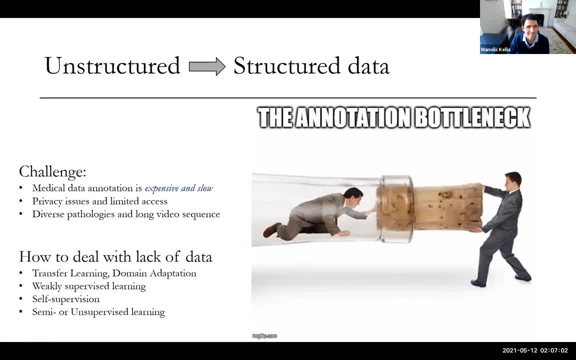 are questions the staff will ask you or we'll answer them. yeah, perfect, yeah so. and also you have this private issue and the limited access when it comes to like, especially in europe, you have gdpr regulations and you have a lot of privacy issues. you have a lot, you have to do, a lot of paperwork. 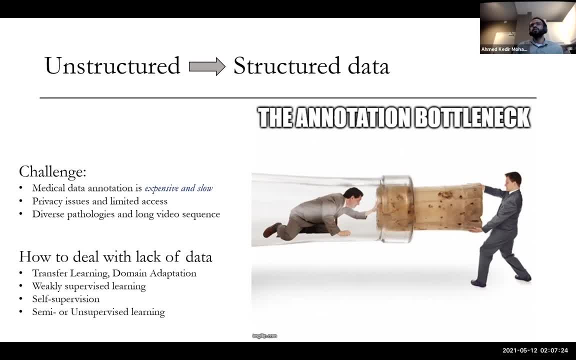 and the other problem is you have this diverse pathologist and a long video sequence. so the problem is this annotation where you need the people to do the labeling of the data. so in the current talk i'm planning, what i'm planning to do is to go through some of 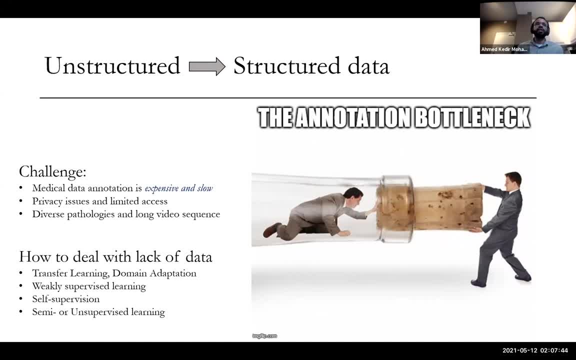 the machine learning approaches that we have been doing in regard to how to do machine learning in absence of data or with the lack of data. so that's the main problem that we are working on in our group. so typically, some of the ways to handle lack of data is one is transfer learning or domain adaptation. 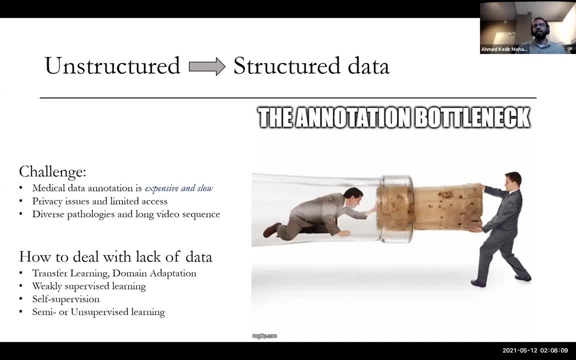 and weekly supervised learning and self-supervision. of course, holy grail is, of course, unsupervised learning. if you can do unsupervised, then you are good to go. yeah, so i will try to cover at least the top three works that we have been working on. so earlier approach. so i will take you now for a 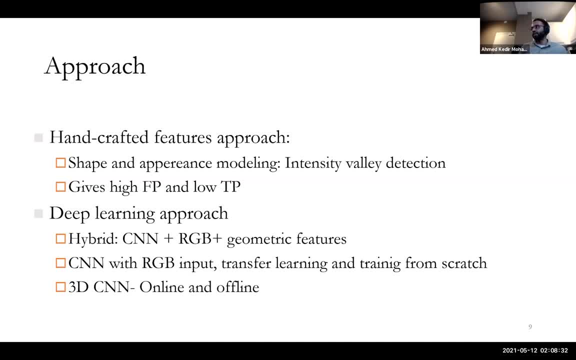 colonoscopy kind video poly protection problem, so earlier approach. so i will take you now for colonoscopy kind video poly protection problem, so earlier. workers in colonoscopy polyp detection. they take this shape information, for example the curvature information of the image, to try to model. 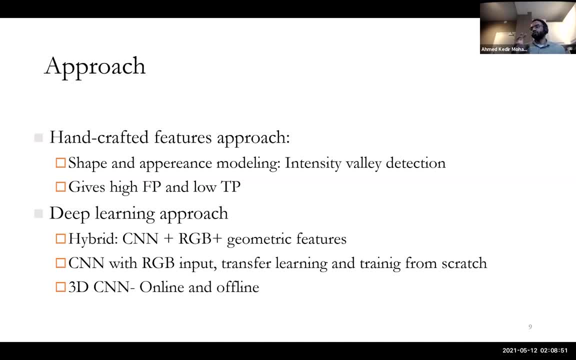 what a polyp looks like. so if, if you try to model it, it's like it has compared to the surrounding area, polyp have a higher curvature as compared to the normal tissue, so you can do some sort of intensity by detection or something like that. but the problem is you'll have this high. 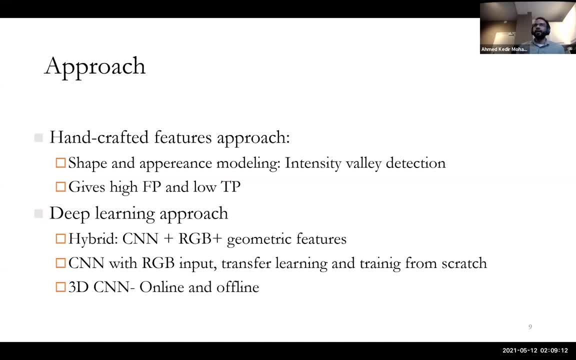 false positives and and that means the doctor needs to check it anyway. so that's a big problem and there have been. since the deep learning come to mainstream, there have been a lot of work that try to do deep learning on it, for example, using CNN with our 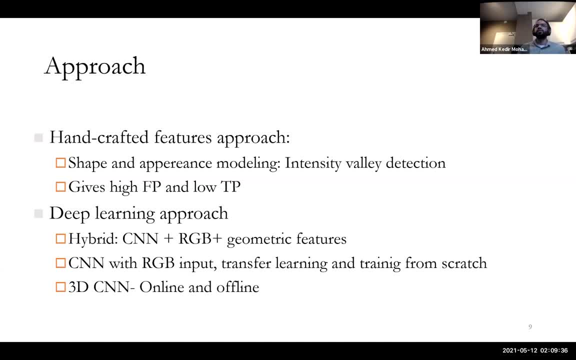 rgb image or adding some geometric features, or there are also transfer learning approaches where you try to fine-tune image, net trained weights, or 3d CNN, using the video as a whole sequence and doing 3d convolutions. so the the work i'm presenting today is one is 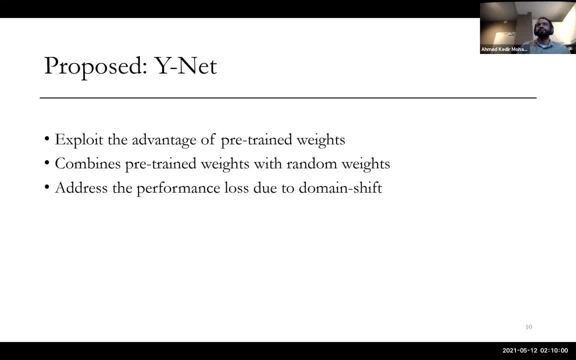 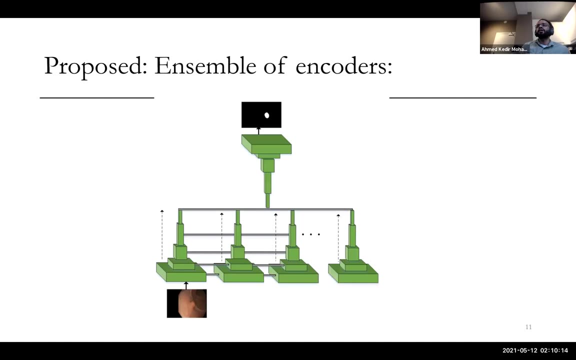 ynet. so this approach is we try to use. we try to exploit the advantage of pre-trained weight and also random initialization and we try to address some of domain performance loss due to domain shift. so the architecture is basically, if you look at, a lot of work is. 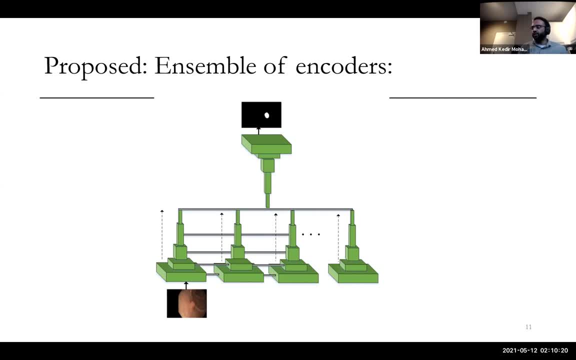 the focus, especially for object detection, image segmentation. most of the focus is on the decoder side. so in this work what we try to do is we have, we have the an input image, then we have different variation of this input image. so this is a general approach. so we have this encoder. so we have two encoders. one is pre-trained from image net. 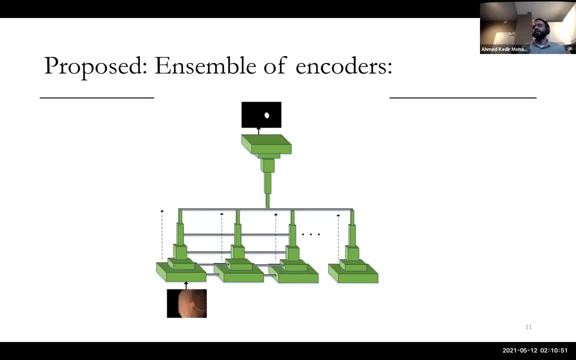 and the other is pre-trained and random initialized weights. then on each image the images are augmented, not geometric augmentation that changes the, the mask of the image, but any kind of augmentation, like intensity augmentation or contrast enhancement and something like that. then what we try to do is since, like, for example, if you already 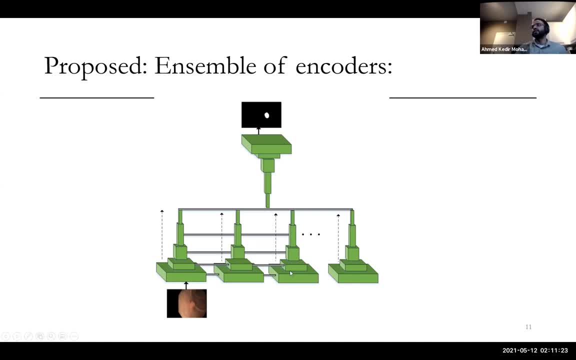 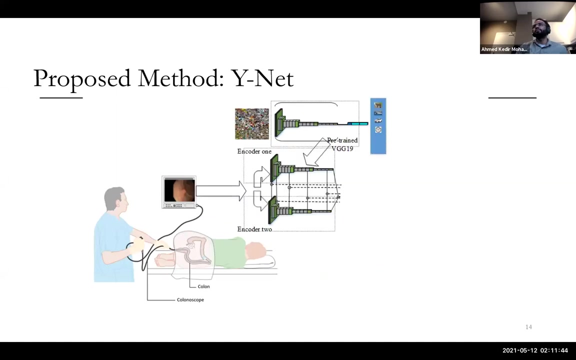 pre-trained these weights and this is random and this is pre-trained and you have different variations of the input. so the assumption is the mask will not change anyway due to the augmentations. so you want to have this consistent kind of representation, yeah, so then? so we start with pre-trained vgg network which is trained on image net, then the 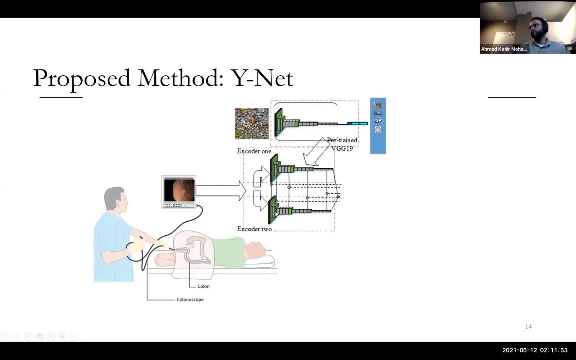 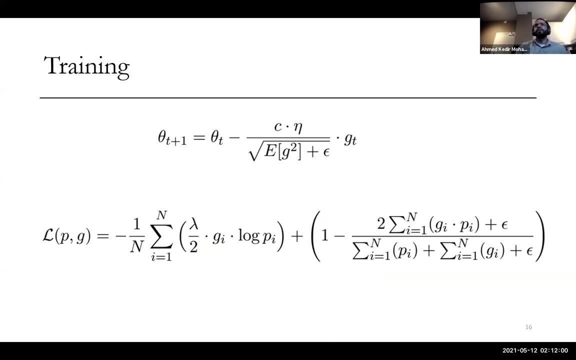 second encoder is random initialized but the image is transformed or enhanced, any kind of augmentation. then what we, what we did next is we modified the learning rate based on which encoder you are training on. so if you have, for example, if you are training, if you have the encoder of the first encoder, which is pre-trained, 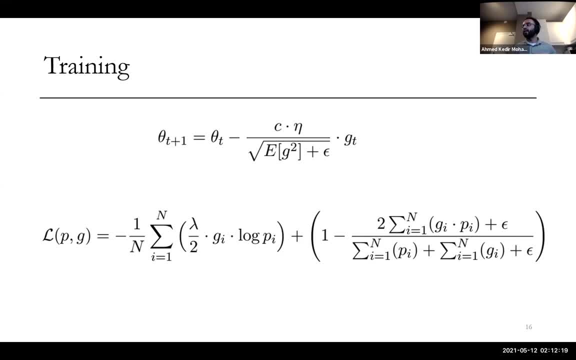 from image net. we know that earlier layers learn something important, for example like color and early features, so primitive features. so you want to keep those features, so you don't want to find you in those layers. that much so you. you take higher learning rates on the other encoders that. 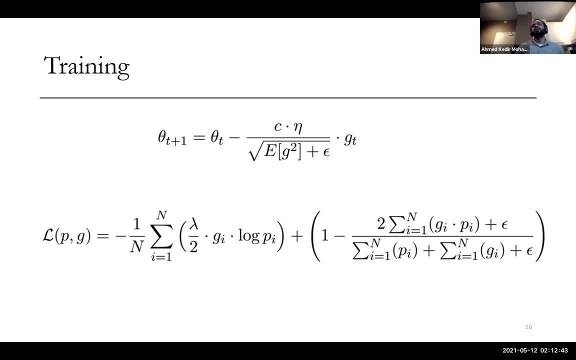 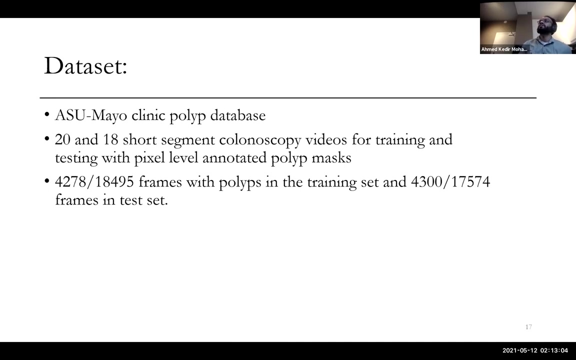 are initialized from random then. so it depends on which encoder you are training on, so you have this encoder based learning rate. then we take the binary cross entropy and the dice loss function together. so for the assets- for this one i will come later on- we collected our own test as well, but for this one we take the publicly. 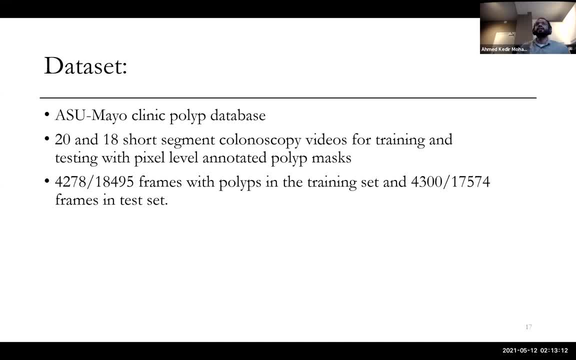 available assets called the isu myoclinic assets, and we have 20 and 18 short segment colonoscopy videos for training and testing. so they are split and out of that one, uh 4278 frames have polyps and the remainings are negative and the same is for this test. so for evaluation we took a 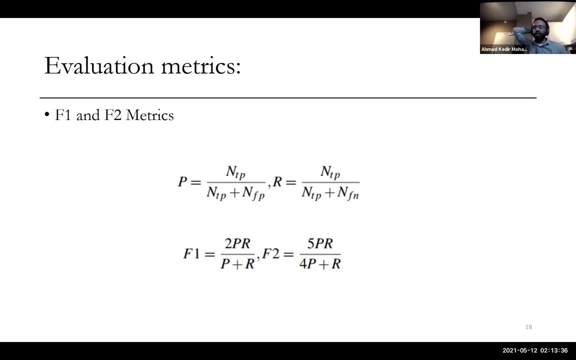 precision recall f1, f2 score. so a lot of people, especially when in medical imaging. i think recall is very important as compared to precision, because if you have high recall then if you have low recall, that means if you miss detecting, then that he will develop a tumor. so 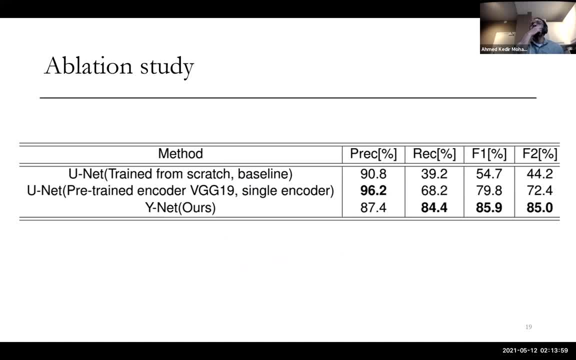 that's a problem. then we did some ablation study. so the first thing we did was we just take the unit architecture. then if you uh trains from scratch, then the performance for f1 score is around 54.7, and if you use unit pre-trained on vgg single encoder then that actually helps. so, uh, that's. 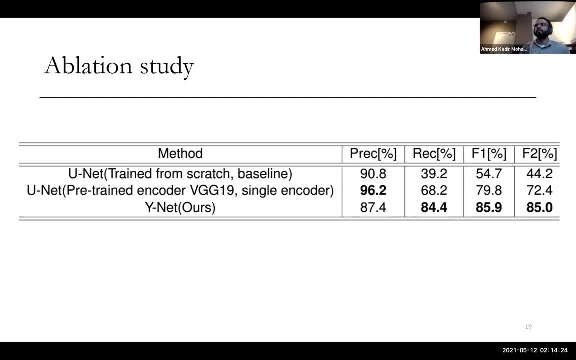 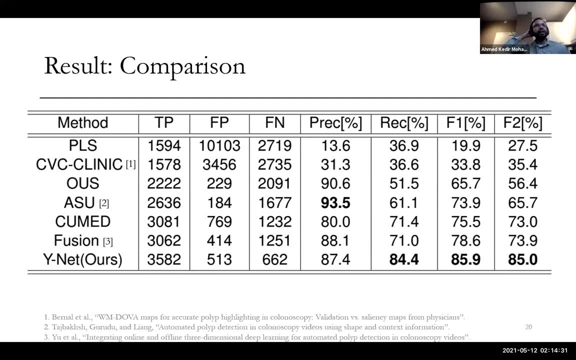 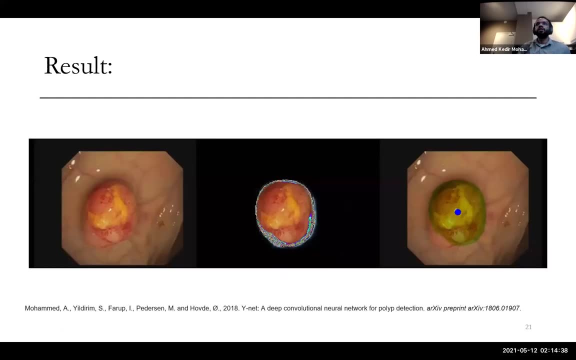 around 79, and if you use y net, which is multiple variation of the same input, you get around 85.9. so we also compare with other existing methods and, uh, this is uh the result. so, uh, let me show you some videos, uh, so this is a. 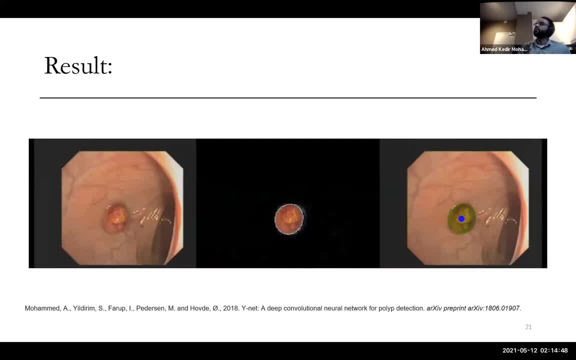 that's so. this is a polyp. so if you look at this you can't say this is natural acid, because it's. it's like, in normal case, the doctor. so this is the observer effect. that is common in vision problems as well, like here. the chronoscope is moving very slow, but, uh, in real case the doctor will be very fast. 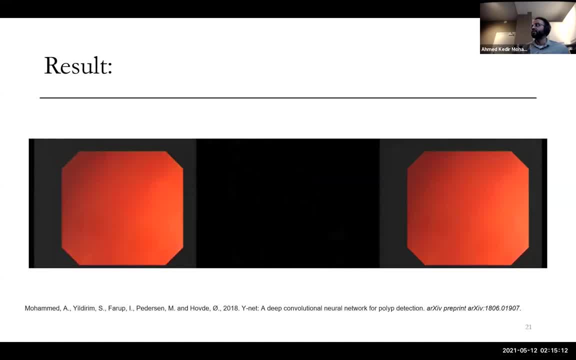 you have a lot of patients and he will be doing, but this is the acid that currently available and a lot of people are using it. yeah, it's not that fun to watch, so if you guys don't like it, i can just pause and pass. yeah, so, uh, the next thing we try to do is we try to collect our own assets. uh, so, 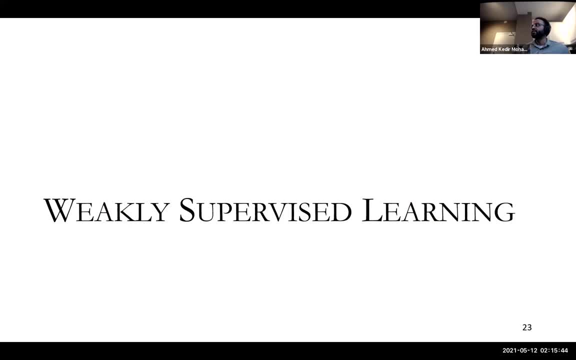 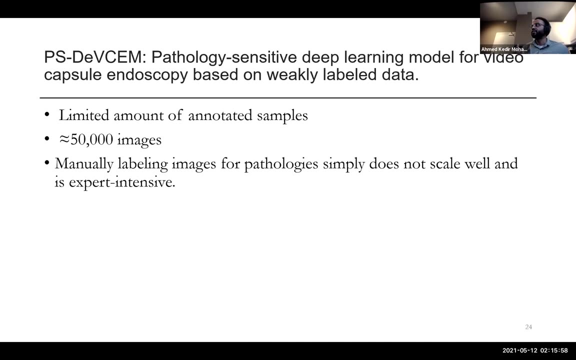 the problem is the supervised learning problem, and i will come to that. what, what means uh? so we have around 50 000 image for for given procedure and we collected around uh 41 videos. that's a lot of frames to label and so we can't label this. so it's- uh, it's very hard problem. so what we, what we try to do, is: 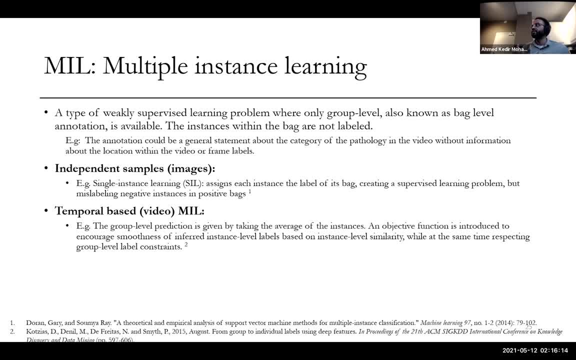 we try to formulate this problem into multiple, multiple instance learning, well, annotation. but you don't have uh individual label for each component, uh each element in the bag. so the assumption is like you have a bag which, for example, this could be a bunch of frames you have. 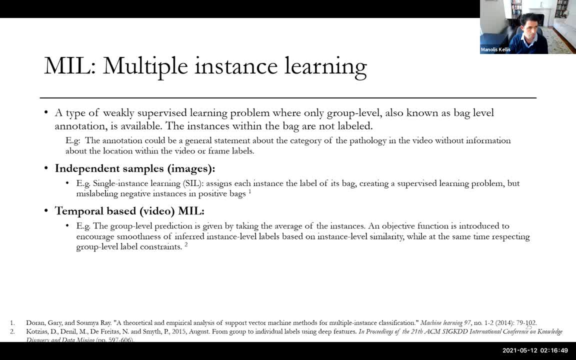 a label for all of them, but you don't have the labels for in the individual frames. so it could be that you have a video. in the video it says like okay, this video contains a tumor, but it doesn't tell you where the tumor is. i don't know where the tumor is right. so you can do a lot of this. 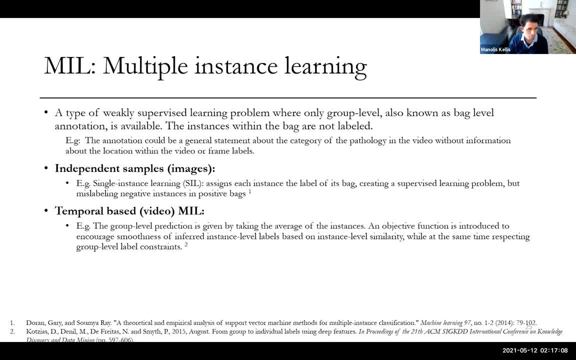 and there's a lot of problems with that. you can do- uh, you can do. one simple approach, for example, if you want to solve this, is you take- okay, let's say, let's take the labels of the bag to be the labels of the the individual components, and you can do supervised learning problem, but that will. 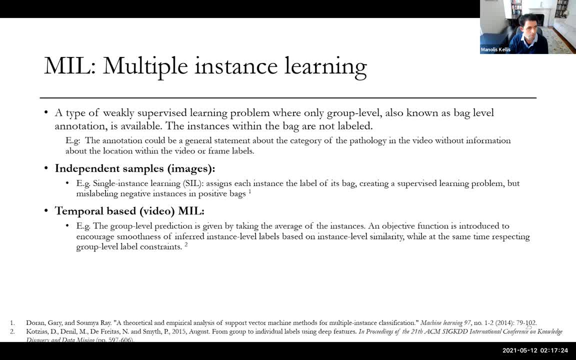 not give you an optimal solution because you, in the video, not all of them have the polyp, so some of them have, for example, some of them in the video, some of them are negative classes, okay, so So you have that problem, So, but that's yeah. 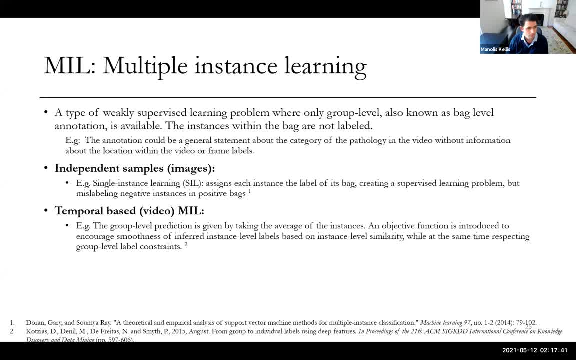 If you want to do a simplified version of the problem is you just assign the label of the bank to the individual frames. Then if you do self fully supervised learning, you will get some results, but it's not the optimal result. The other approach would be is: 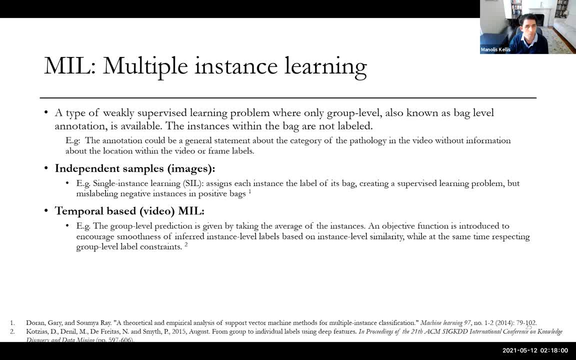 since you only have the labels for the video, what you can do is, like you try to predict for individual contribution from each frame. then you optimize the loss on the final video label of the aggregation. So that's what have been like in this paper. 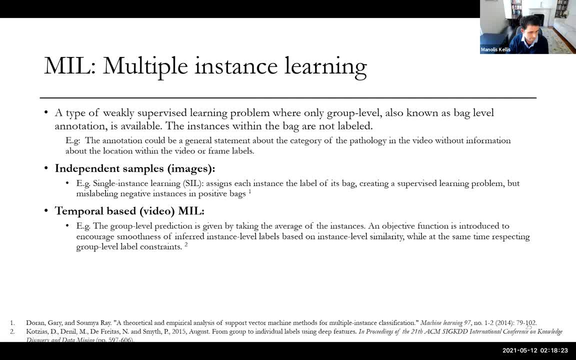 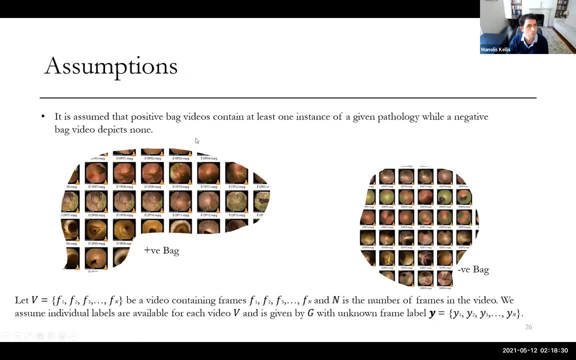 that's what they did. So the basic assumption of multiple instance learning is: you have this positive bank and this negative bank. The shape of this positive bag and negative bag has nothing to do with the actual learning, So it's just a bad drawing from my side. 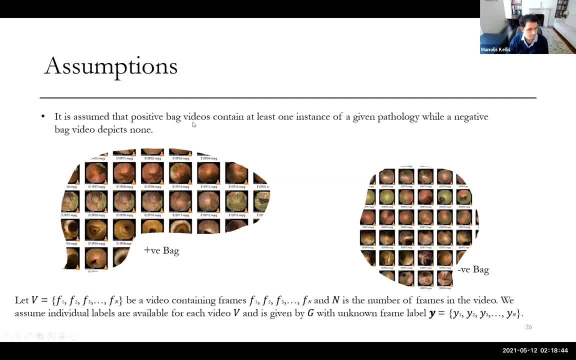 So what? the assumption is basically: positive bag at least contain one of the pathologists- Yeah, that's what I'm interested in. But the negative bag is always negative. There is nothing negative, positive in the negative bag. So if you assume, like the 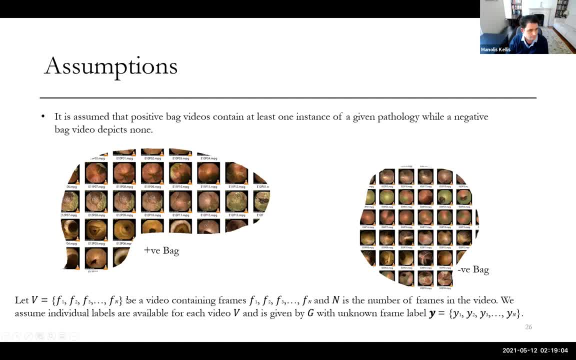 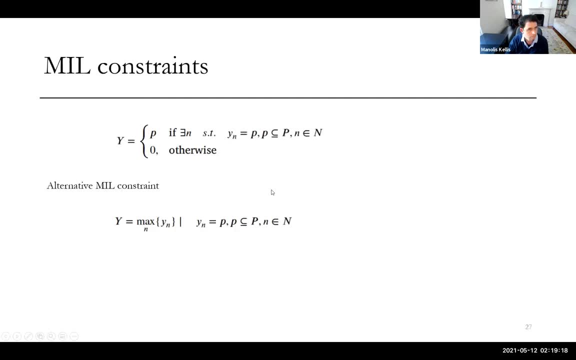 frame one and frame and the video contains in frames and the sole number of frames then for each frame you don't know this label, but what you know is the label of the video as a group. So the meal constraint problem: you can reformulate it as such that this is a 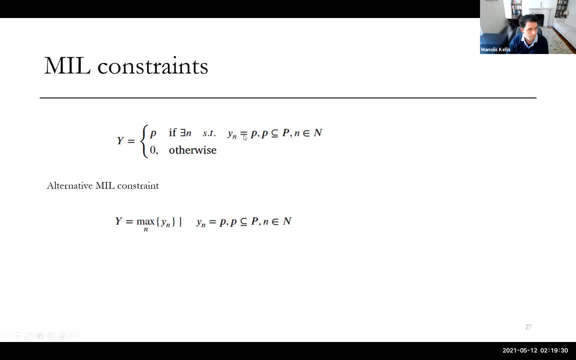 the pathology you are interested in, such that Yn is basically the frame. the frame that contain any pathology will be the label for the whole bag. Or you can also alternatively formulate as the maximum on all frames that contain the pathology. So if you look at the problems, 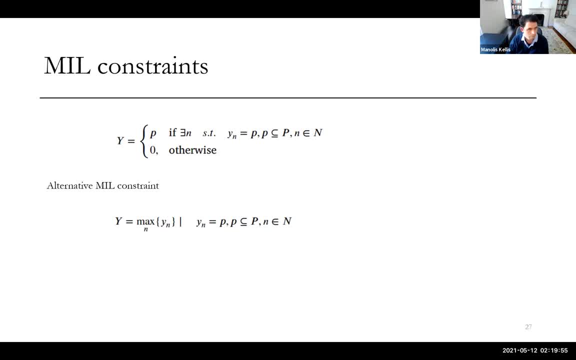 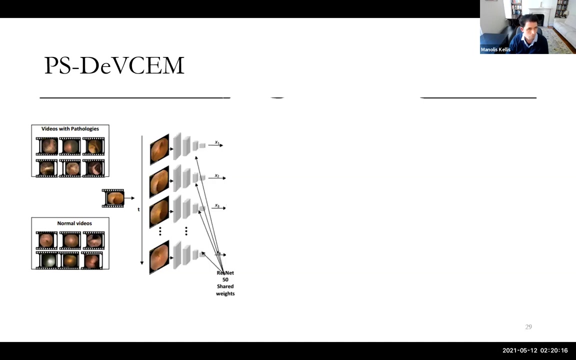 basically how to find which frames contain the pathology as compared to the rest of the video. So to do that, what we started is we have this videos with pathologists and the normal videos and we converted, we extracted ResNet 50 features from for each frame. 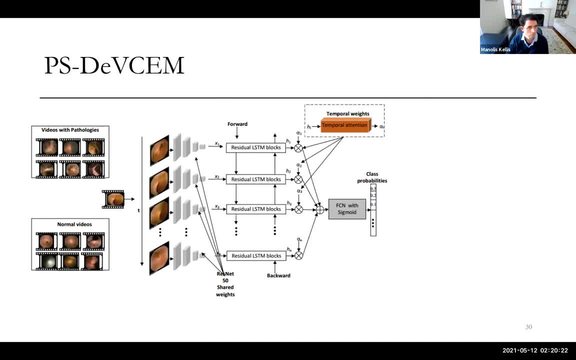 Then we pass through the residual LSTM blocks. So this residual LSTM blocks are contains bidirectional, two bidirectional LSTM and you have a skip connection taking the row image feature to the output hidden layer. So what we are interested in is basically how to find 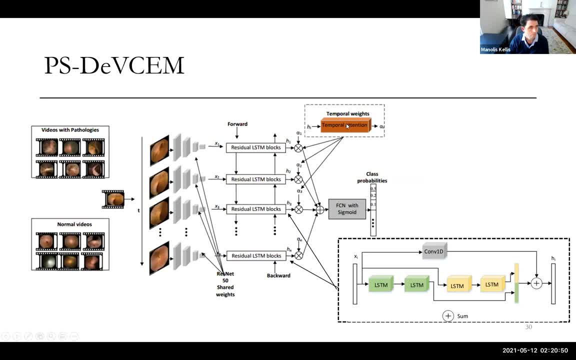 these alphas. So basically this is a contribution of each frame to the final video classification problem- Then what? the only thing we have is actually this: the final video classification. So this alphas are really kind of the contribution. So if you are able to find, 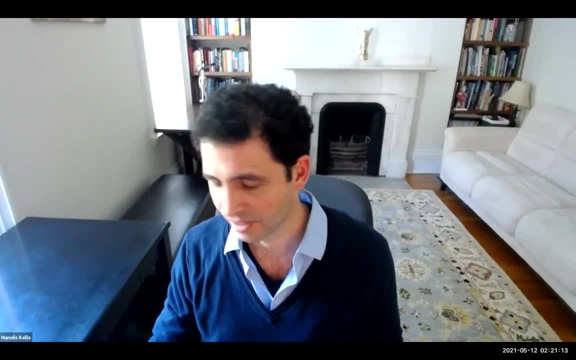 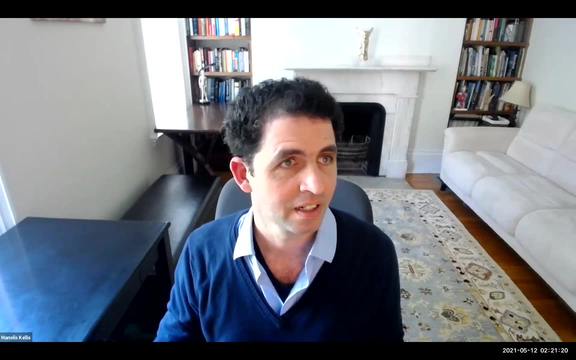 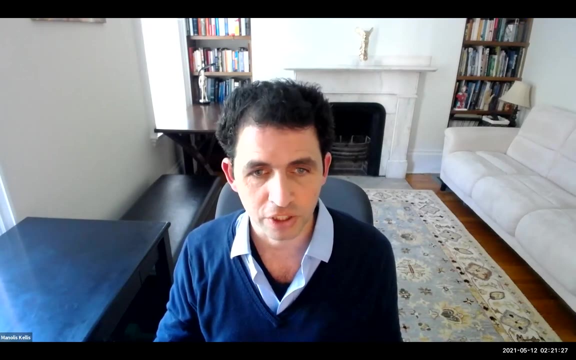 Okay, I'm afraid we've lost our guest speaker. I was a little frightened earlier when we had a little bit of a disruption, So I I don't know if folks have questions to ask Or anything else, I'm going to pause the recording again. 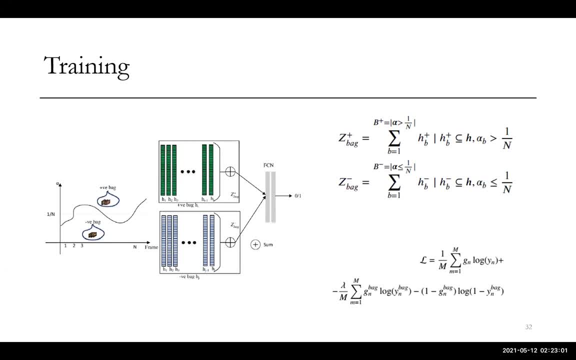 Yeah, And high attention, why? Okay, sorry, Yeah, perfect. So one thing you can exploit is high attention value frames are supposed to contain pathology, So you can exploit this. So if you have, you can try to move the positive. 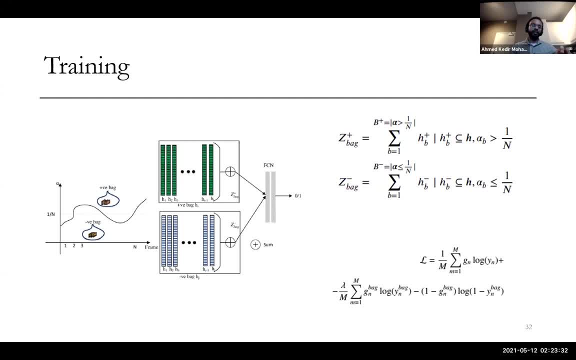 high attention pathology frames with respect to the negative classes and you try to separate them apart, Then the final loss function will be then the binary cross entropy of the video classification, as well as the separation of the bags between the positive and negative bags. 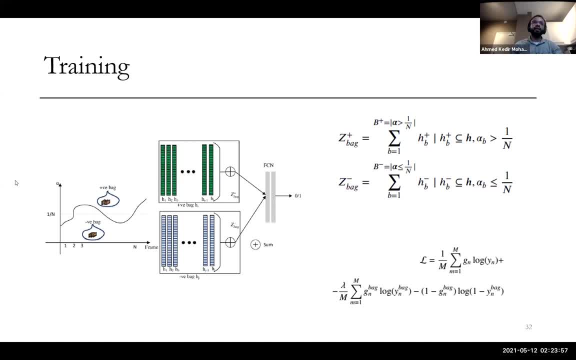 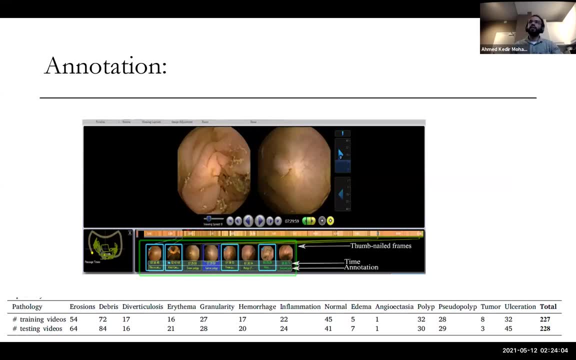 So call in simple higherふ. So to do that, we went to the doctor. So this is how we unfit the data sets. So this is a rapid reader: around 455 small segment videos And I think this is the largest capsule video endoscopy. that's it. 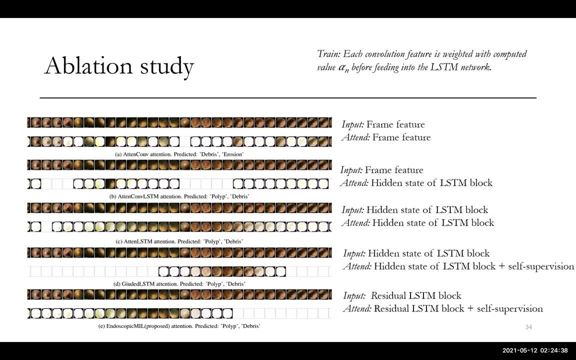 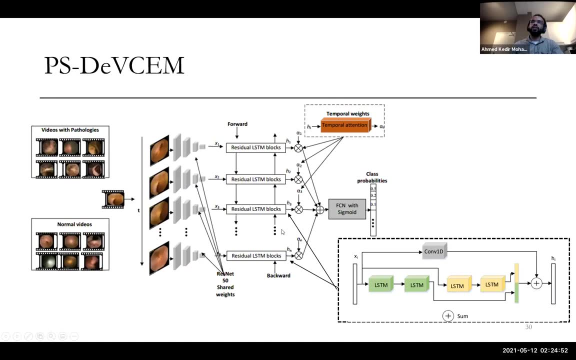 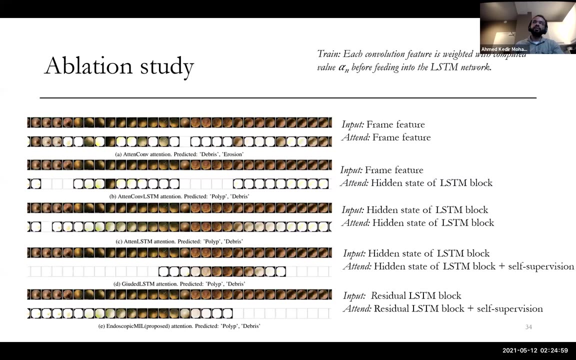 Then the one thing we did was also try to analyze the where to put an attention, So, for example. so what I mean is basically where you want to learn this attention, the contribution. So we did an ablation study where we take, for example, 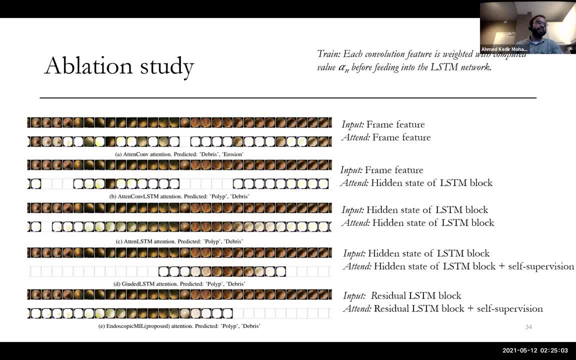 we take the output of ResNet and apply attention on that, Or the other alternative would be is you take the input feature from ResNet and have attention on the LSDM blocks, or have an input to attention block from the LSDM and having it on the LSDM. 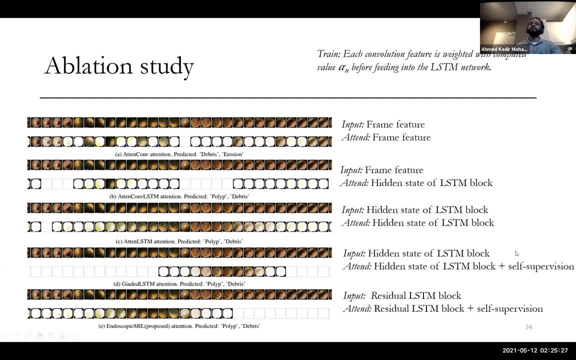 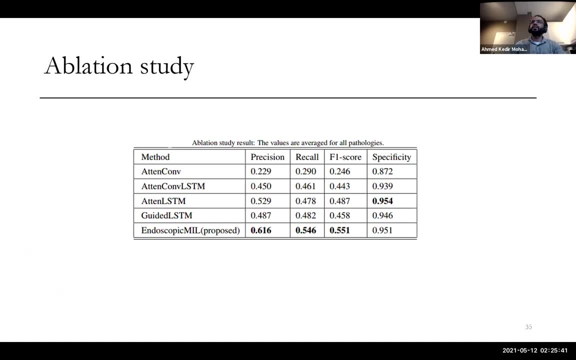 Or you can also have another kind of ablation study where you have this trying to move the high attention classes from low attention classes, And so if you look at the final results out of this, the one that gives you the best is vertically, If you attend the final hidden representation. 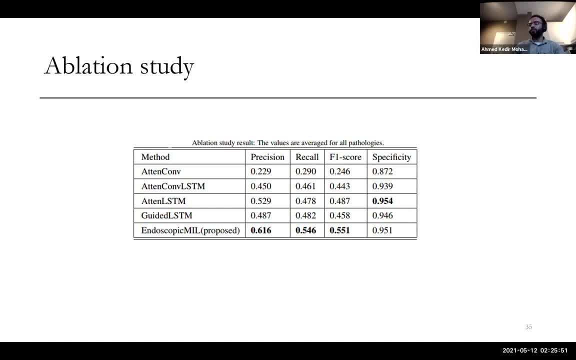 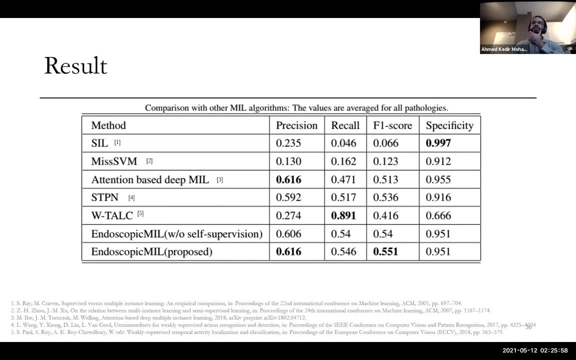 and apply it on the final or on the final output. that will give you the best performance, And we compared it with the other approaches. that uses metric learning. So this all some of the methods here. we just implemented them for capsule video endoscopy. 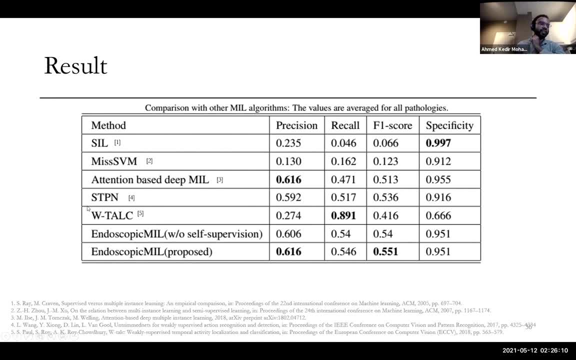 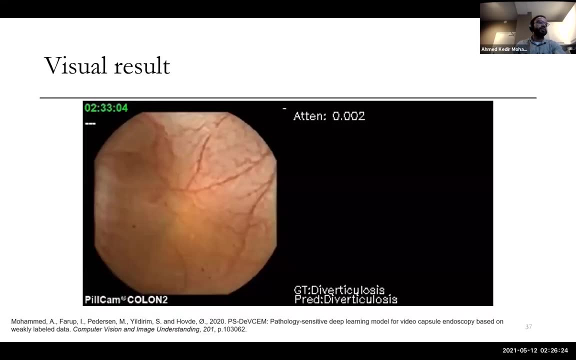 but some of this work is very similar to activity recognition kind of problem in natural video analysis. So we implemented them and we tested And we got the results. So I just want to see the results. So the data was very good, So I'm going to show you the results. 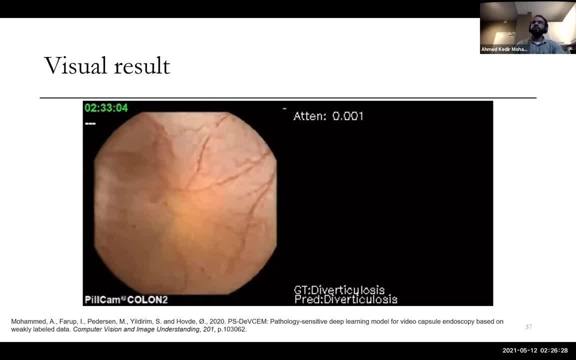 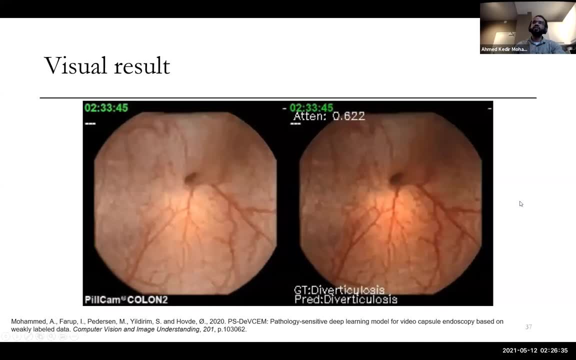 This is the data versus case. So this is the attention, or the networks, what it sees. So so that vertical is vertical. This is the diverticulus. So you can see that when it's this diverticulus, the networks start firing. 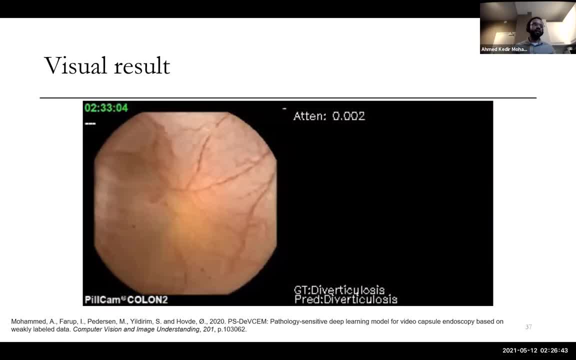 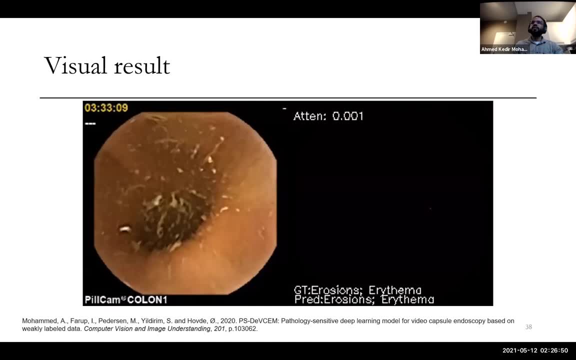 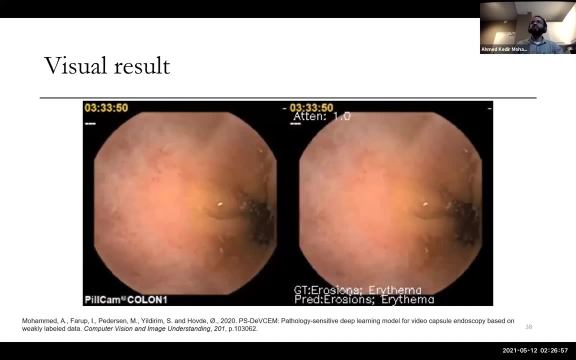 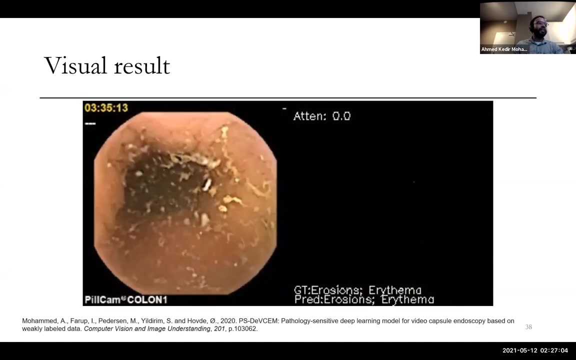 So the the other was attentions will be like there is no attention to other frames. yeah, so this is erythema, uh, and erosion. so i don't know how many of you will know erythema and erosion, unless you guys are medical doctors. so, yeah, so the other approach that you 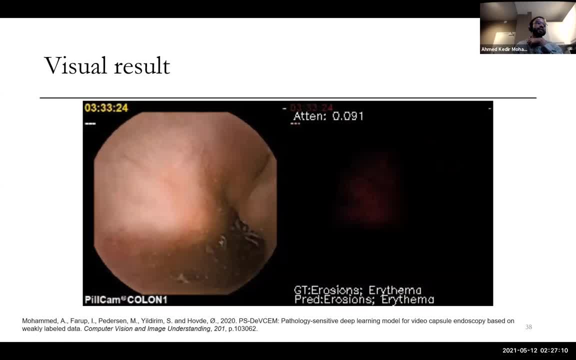 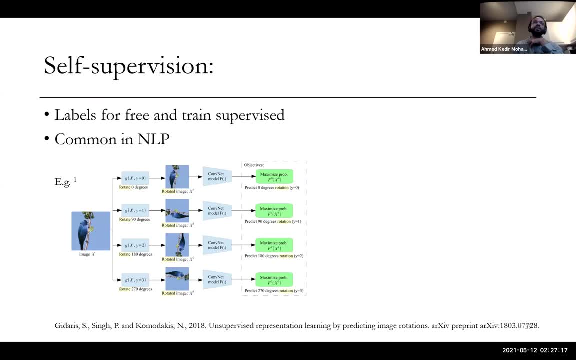 could follow would be is: if you don't have a lot of label, data is self-supervision. so i think you guys have seen this block diagram a lot. so basically, in self-supervision, what you have is the data contains some sort of the label and that you try to learn that one and you train. 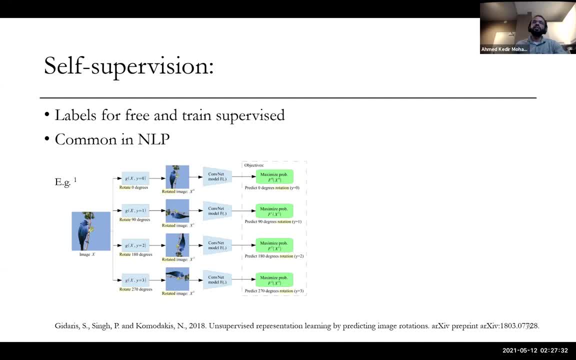 supervised, basically. so in nlp, for example, you try to predict the next word in a sentence. so in image processing, like in computer vision, one of such famous words work is basically: uh, try to predict the rotation. so you have the an image and you rotate it by 90. 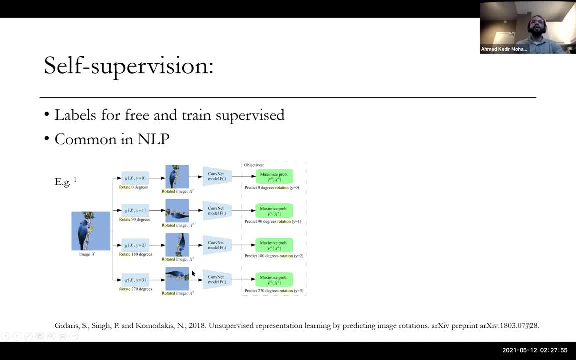 degrees and different type of degrees and you try to predict what is the angle and use this one for, uh, warm, starting your training or uh, it's actually falls under representation learning problem. so this: do you guys think this will work for capsule video endoscopy? all the images are tumbled up, so i guess not. 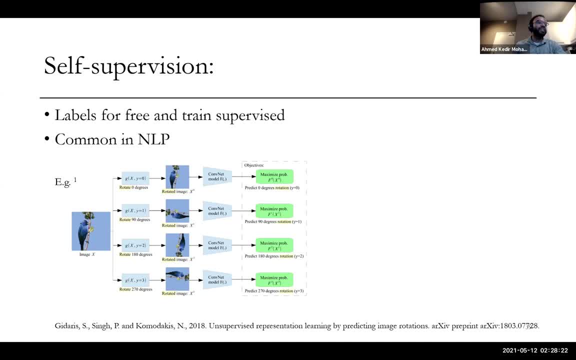 exactly. so. that's one problem when you work on medical imaging. so if you look at the colon, you can't see. you are looking upside down because there is no. it's a rotation invariant, so you need to come up with different ways of uh learning some representation. so, uh, one approach that we find. 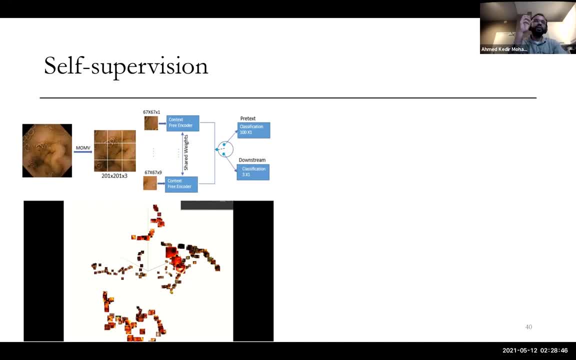 kind of working is a jigsaw problem where you have, where you partition the image into patches and you pass through the uh, an encoder. so each patch you pass through it an encoder. then you try to reconstruct the image. in all honesty, ahmed, i don't know how well i would do at that task. 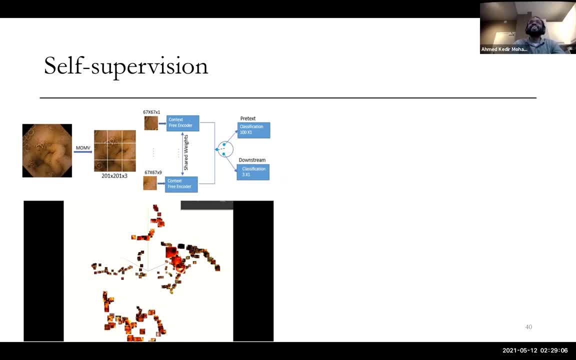 yeah, so even i asked. i have medical collaborators and very hard for them as well. yeah, yeah, so in this problem is very good, try to, uh, yeah, reorganize the frames. we've seen many of these uh problems in, uh, our previous lectures, so it's very nice to see them again in practice. yes, exactly yeah, so what we found is very good. 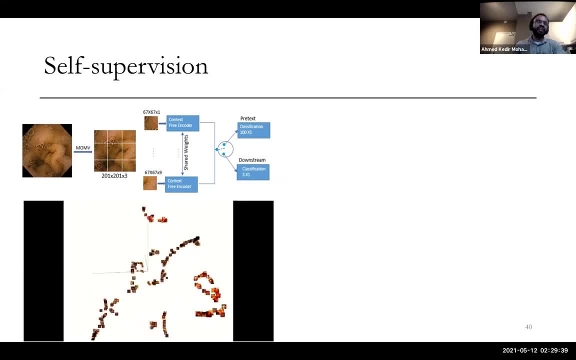 they form some sort of cluster, but they, the clusters, are not meaningful and pathologically meaningful like you want to have um something. so, uh, basically, this is called pretext task. so a pretext task is this: three tasks that you do, and the downstream task is, uh, the one that 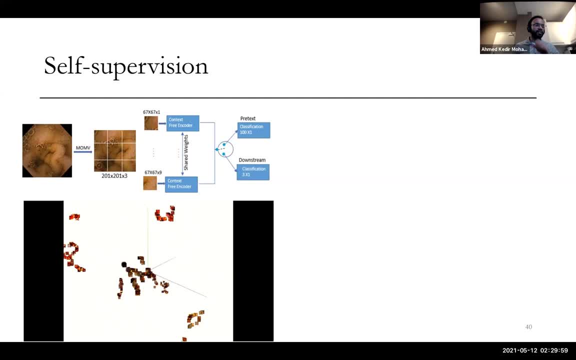 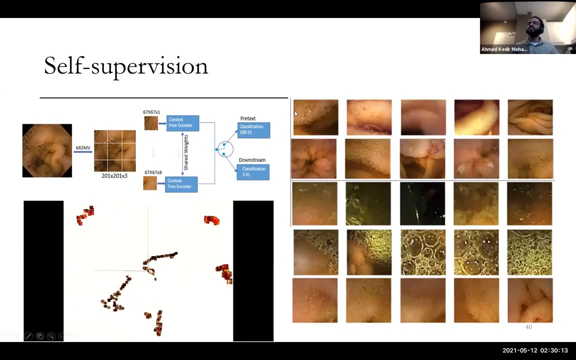 we are interested in, which is pathology classification. so now what we see is basically, we don't have that much of that pathology classification. what we have is another interesting classification. so If you, for example, if you input this image, what you get is something that looks similar, but it doesn't mean it is clinically significant classification. 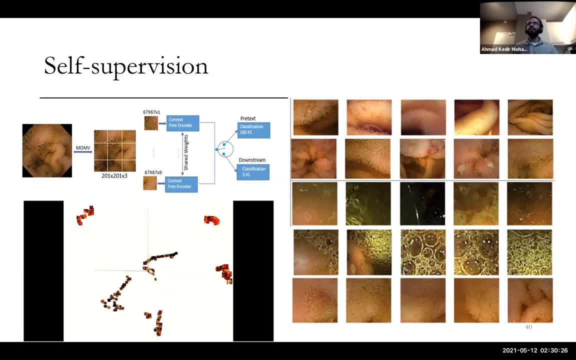 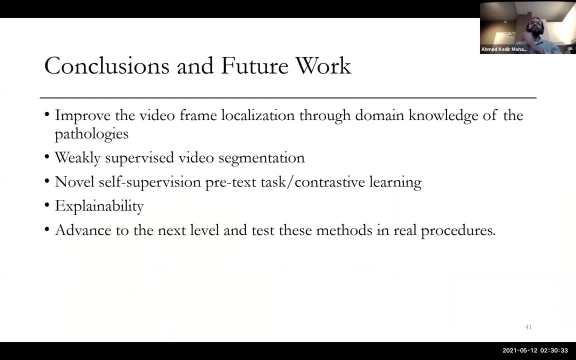 So we are looking into a lot of these pre-tech tasks now. Maybe I'll share another time some of the works on this side. So, in conclusion, what we see is it's important to improve the video frame localization through domain knowledge. For example, if you have Crohn's disease, as compared to arthritis colitis, Crohn's disease could be it starts from, if arthritis colitis starts from, rectum, 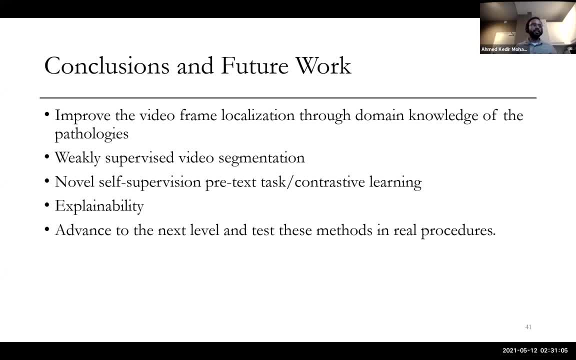 and it goes up And Crohn's disease can happen anywhere. So there is some pathological information that could be interesting to use to try to localize the disease more precisely. So we are looking into that as well And the other thing that's interesting to look into.